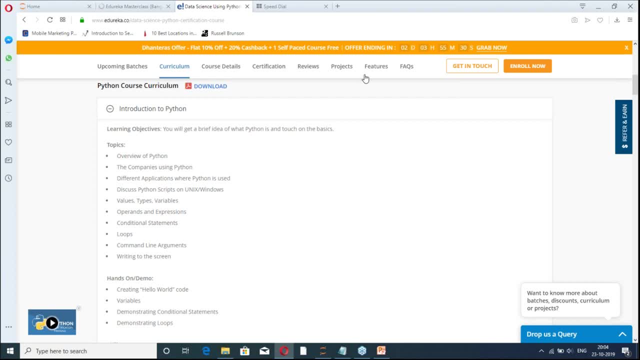 language properly right and some of you guys might know python already and some of you might start learning as well, and some of you might have seen few things, uh, during the code which i have been showing you guys, uh, which belongs to python only, you might have found it is somewhat easier to understand. even you might. 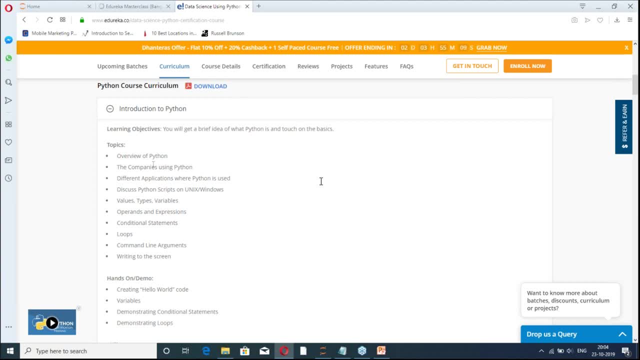 be completely new to the programming language, right? so that is one of the beauty of the python, and you will be studying now in the detail about the python programming language, right. so here, this is what you are going to study first. the first thing- uh, initially you will study is the basics. 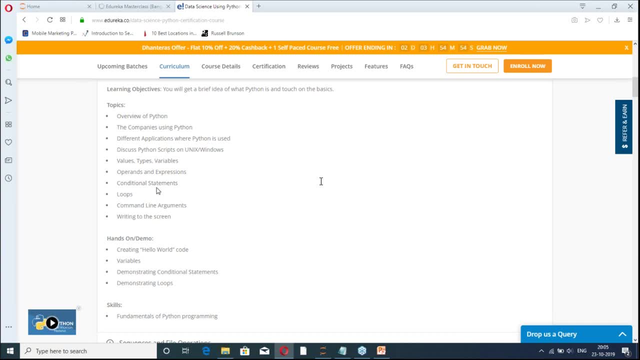 of the python, right. so overview loops, how you can write the loops, operators and all those things. basically right and like writing your first program, which we call as a hello world program, and after that you will be understanding variables. and if you guys are new to python or if you guys 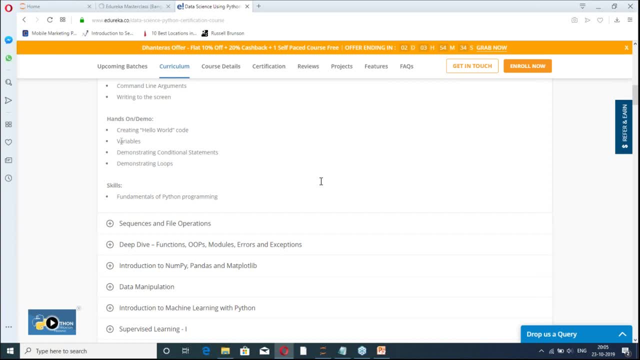 have already gone through some other programming language and if you're coming to the python then you will see here the things are little different when it comes to data types compared to other programming language like java, c, c plus first. python is completely different when it comes to. 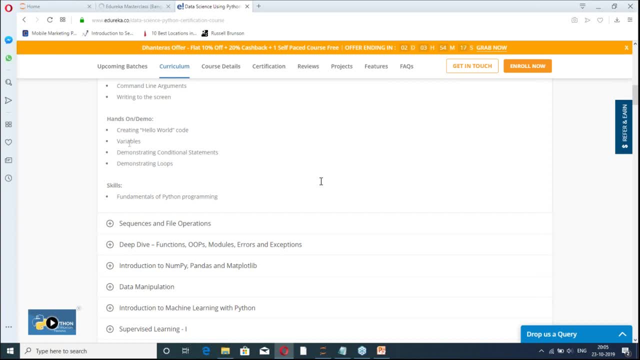 assigning the memory and data types and all those things you will find its make is make it easy for you guys, so much so that you will be understanding here and you will see the way memory is being allocated to. the variable is also completely different compared to other ones, right and similarly. after that you will 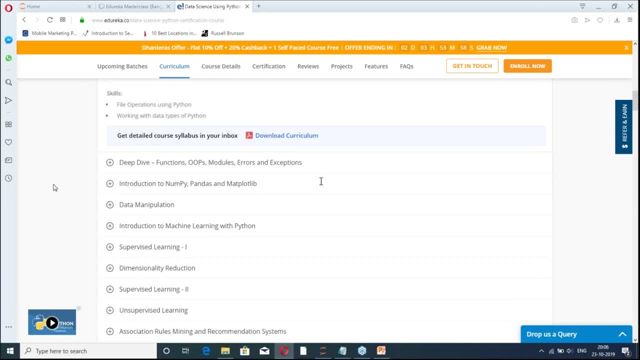 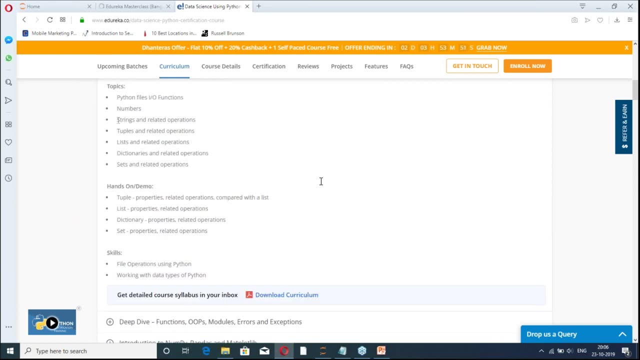 be studying the core, heart of the python. that is your sequences, right. so you will be, uh, studying about the strings, tufl list, dictionary sites- These are basically heart of the python and that makes lot of operation pretty easy for you guys to do right. That is one of the beauty and that is why 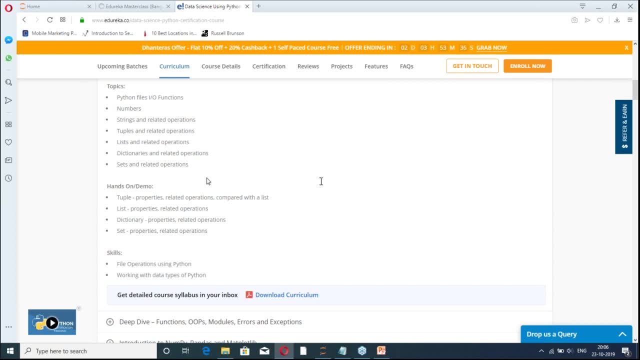 I love personally python programming language compared to the programming language. that is specifically these differences which make programmers life so easy, actually right and as well as you will understand here how you can read the files using python programming language, and then we will have some practicals as well. case studies will be provided to you. 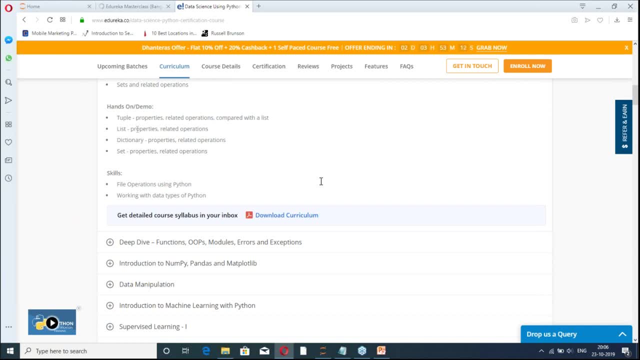 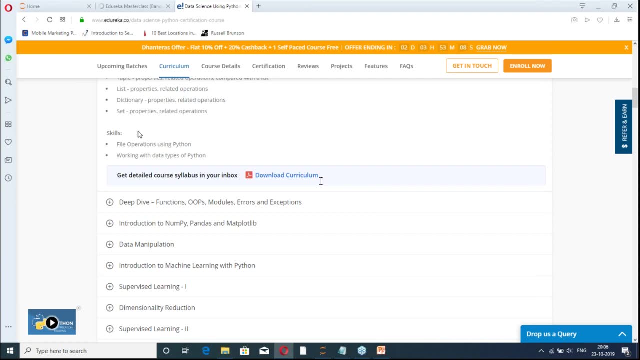 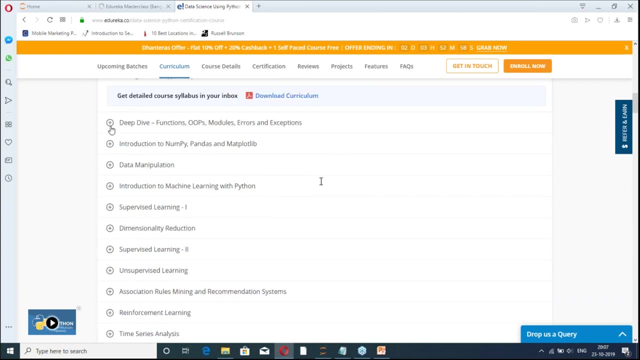 Some practicals instructor will show you guys and some of the practicals you are supposed to do. you need to do some assignments yourself as well, So that is one of the good thing about it. and then let's talk about the next. after that you will go into the detail very. 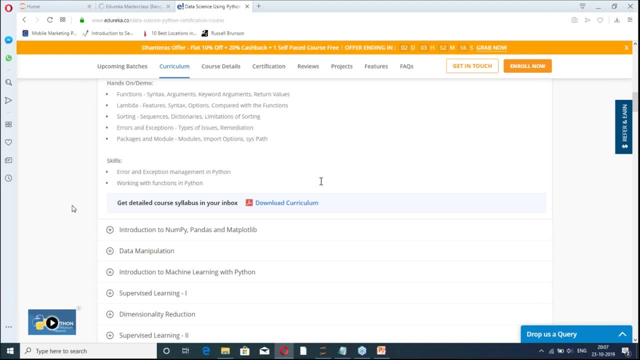 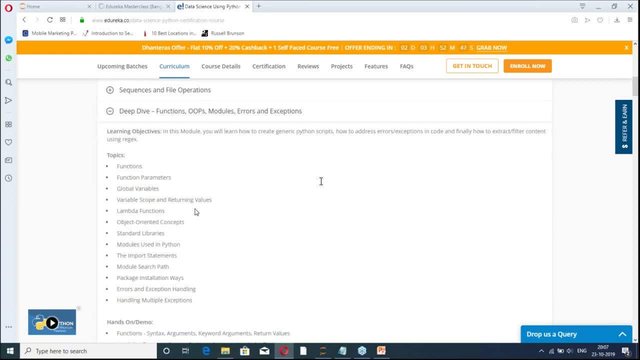 detailed way of python which you will be studying. little serious here. you guys will become like function rules. modules are an exception, so you guys need to be little serious here in this particular topics when you will study, because these are the important topics, as well as lot of things you can do pretty easily if you understand all these things nicely. 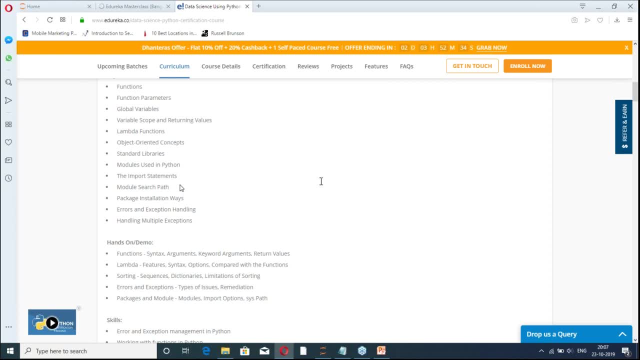 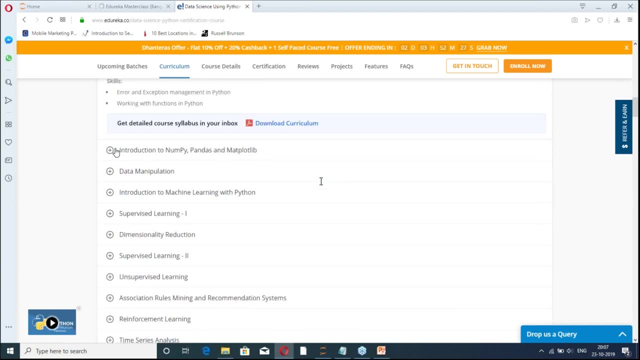 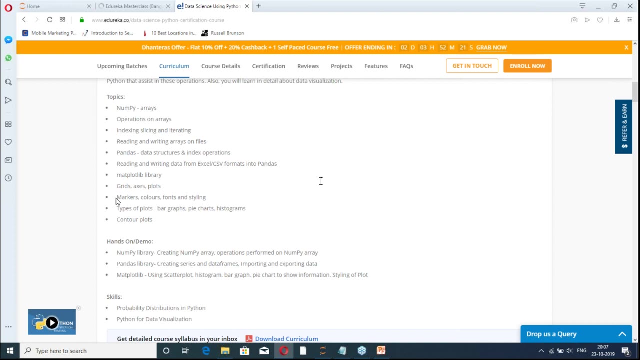 So these are, if you go for interview, these are the concepts which would be asked a lot to you guys, right, and after that, now the things are getting ready for you guys for data science, right, And this is you will have your first And counter to the libraries which are called to the specifically pre-processing of the 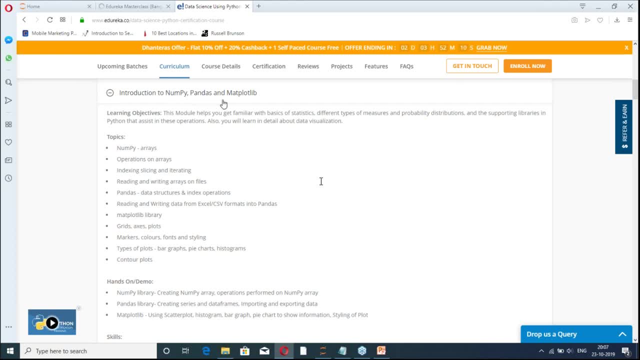 data in the data science and you will be studying about NumPy pandas and that plotly so- NumPy is like num name- might be telling you something like numerical python, which will be. so here you will be dealing, doing a lot of scientific calculation and all pretty easily using the 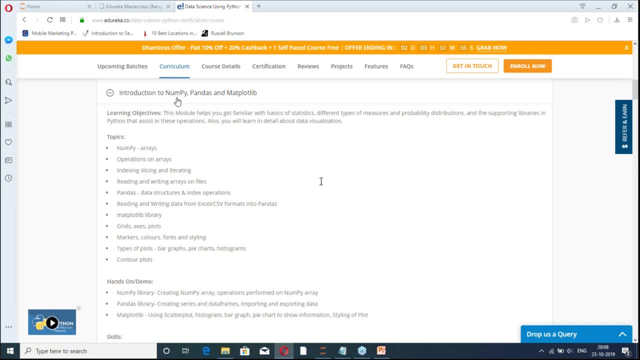 NumPy and that, too, also very faster. if you write your own code to do this, it is going to take a lot of time, But using NumPy you will be doing. you will be able to do it quickly and then find out. so pandas provide a better way to store your data and operate on them is basically from. 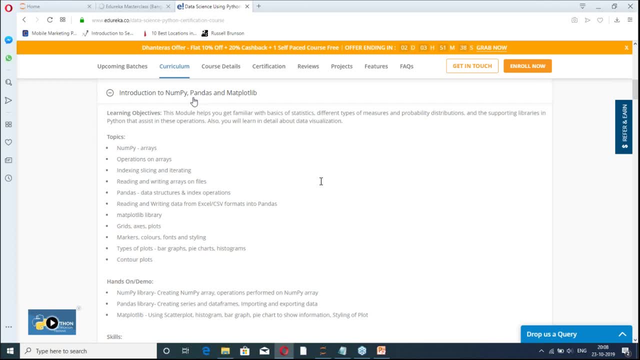 the point of view of data science. So that is a good thing about the pandas. how is it different from the other data structure? is that it is specifically made for data science purpose only. after that you want to do visualization. as you guys know already, visualization is one of the very, very core and important things. 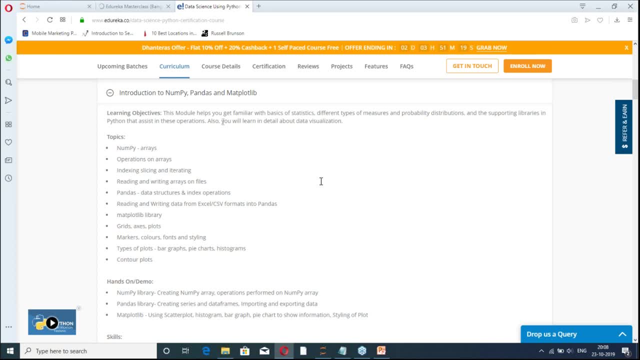 in the topic of data science. so how good data scientists to you guys are going to become, that depends on how cool and good way visualization you can do and you can understand your data, and that would be done using the matplotlib library. So matplotlib is one of the library which is written here, even though we will not stick. 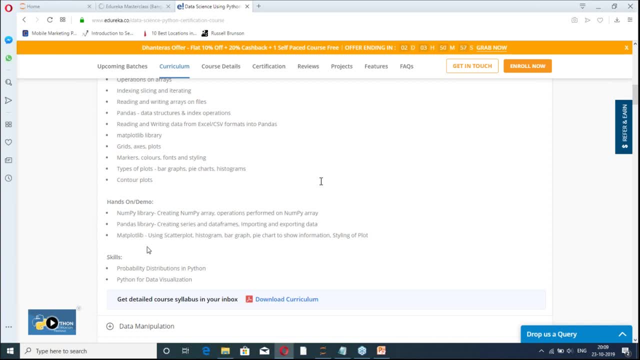 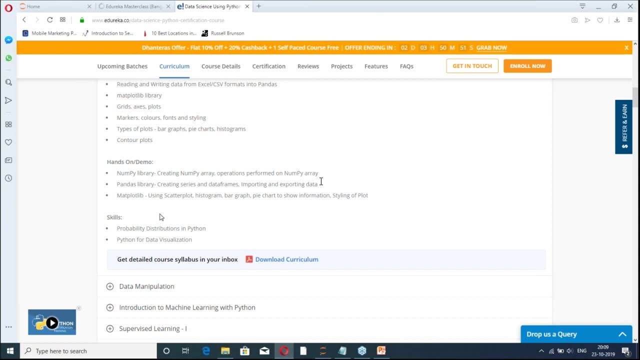 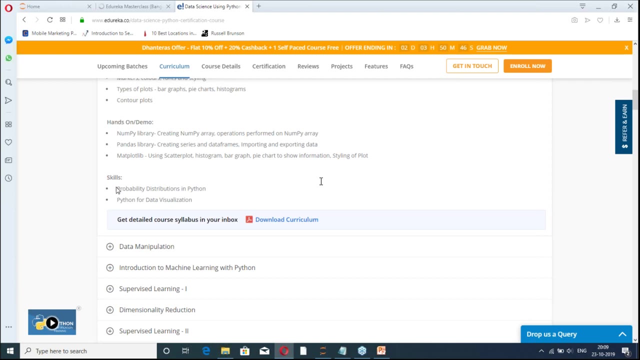 to only the matplotlib library. we will do little advanced library as well, which make your life even more easier and more interesting, And that is the Okay. So we will study about seaborn as well. right, and here you will need to have these, these skills. you will be having probability distribution. you will understand Python for data visualization. 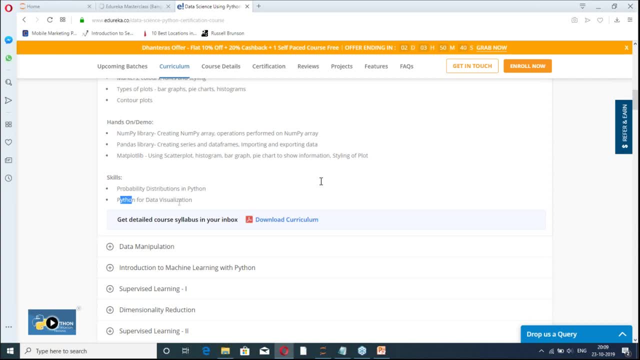 these things, you will understand. and now, once it is done, now you want to play around with your data, and that is what you will do in this, in this module, which is data manipulation. here you will be seeing, you will be having your data into the pandas data frame only. 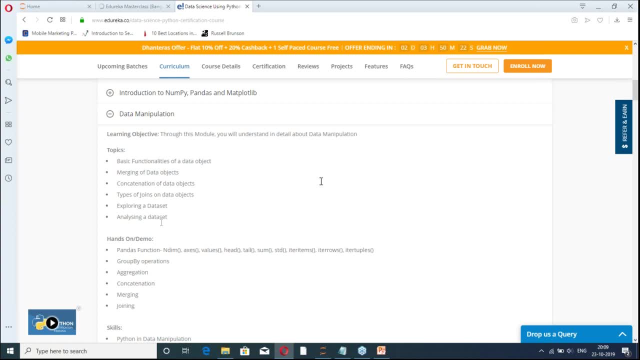 but now how to operate them, how to manipulate a data set, how to do the pre-processing on the data, how to do different, different options, how to aggregate, concatenate, merge, different data frames and how to handle the null values and all those things you guys will be studying. 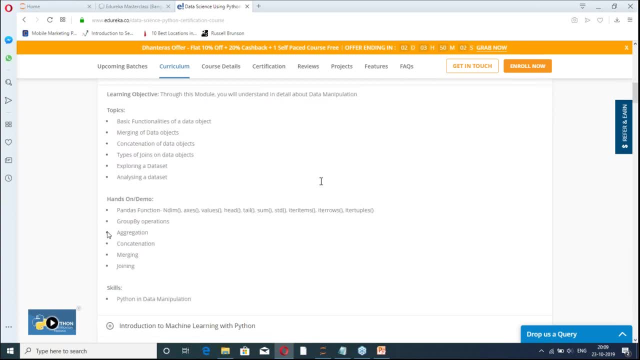 in the data manipulation, and you guys are going to love this part, because here you will need to be little bit logical. it is not only that. what function you are going to use? definitely, Functions Examples are going to make your life easy, but it's still, you need to be little bit logical. 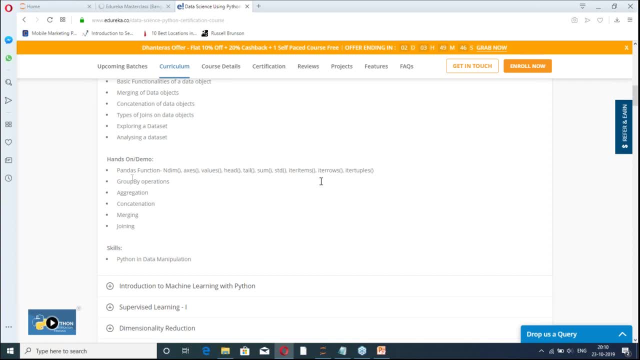 here right and which you guys will be learning as you do. some practical examples here. Okay, and after that, then, the machine learning techniques are getting started and this is the first encounter you guys will have, where we will start. we will discuss about properly in detail what is machine learning exactly, and we will see many use cases. 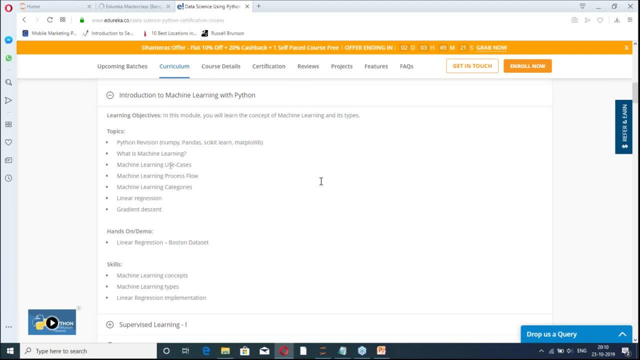 How, How in industries, different, different problems can be understood and taken as a machine learning problem. and then what flow you guys need to follow when you are applying the machine learning technique. this is what you are going to study in this particular module, and then you will. 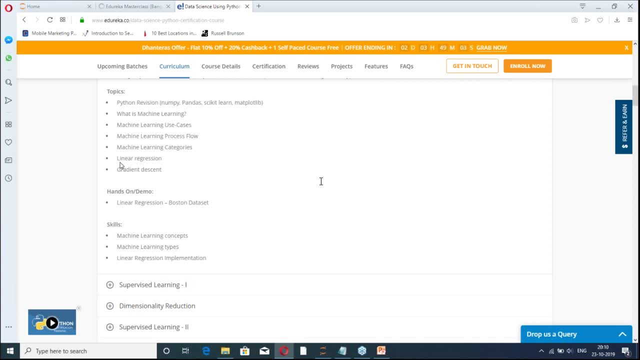 have your first encounter to the supervised learning technique, which you guys might have studied even during the session, free webinar- which is linear regression, but you guys have not gone into The detail yet. and here you guys will be going into the detail property, and then we will 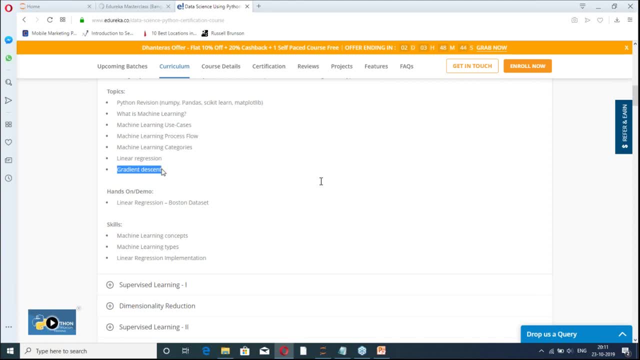 be discussing about the gradient descent specifically, which is one of the very good technique to understand exactly how the training is happening. till now, you just use the functions, but you didn't understand properly- till now because we didn't have time, we also didn't have those things properly- how you can play around different, different parameters, tweaks and what impact. 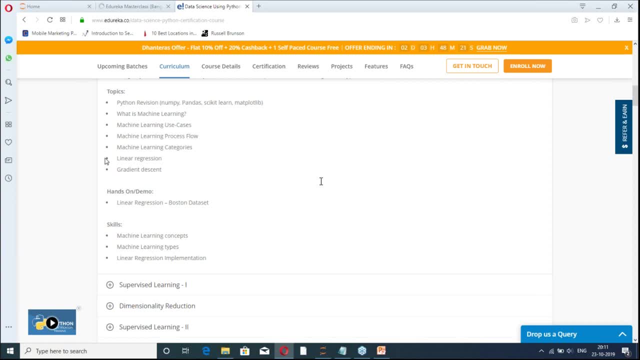 it can make on your algorithms, And that is what you guys are going to do here as well, as you will be studying here in the detail. what is what is the we have? what is the? we say that our training has been done. as you know, overflow- I'm getting this name wrongly- something like overfitting, overfitting. 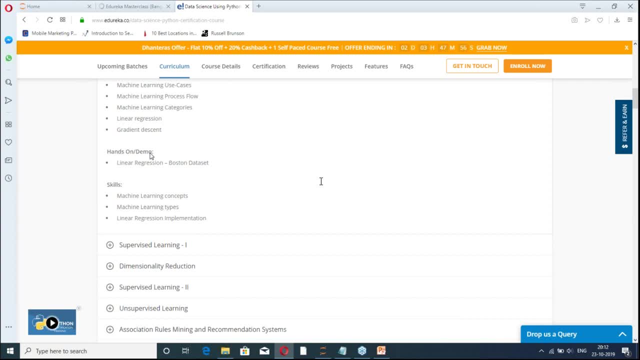 underfitting right and what is the good fit model is that you will go into the detail here in this particular session. Okay, And then, after doing this thing, we will start discussing about supervised learning technique in more detail. we will discuss about the logistic regression- this is entry random for us and 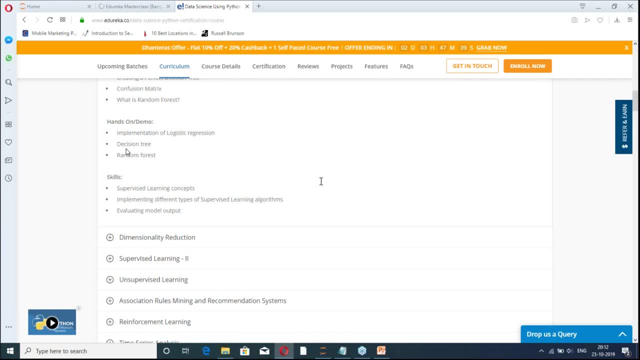 you will also understand here how you play around with their different different parameters, how you can improve your algorithm. also, it is not just using simple playing function, but how to play around those stuff so that your you can do pretty nicely and you can really build something which can. 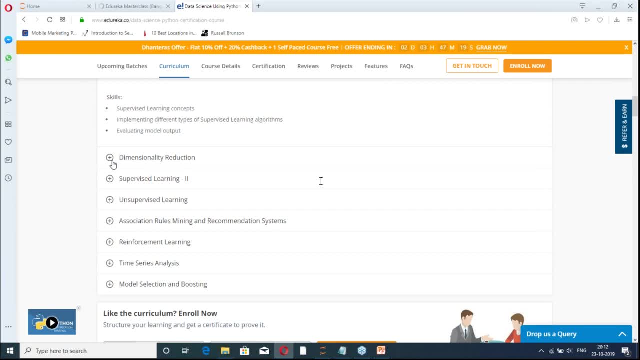 Use in the real world. right and after that, the pool was not the core again. I'm saying this is again very, very important topic, that is, dimensionality detection. in many cases it is going to be used as a first, as a staff, which you are going to apply even before applying. 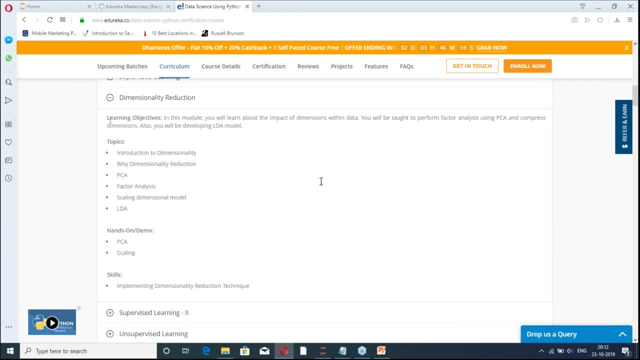 your supervised learning or maybe unsupervised learning. many times you see a lot of competition are happening in machine learning. you find it on the. you do the research on the internet and High dimensions, right, he's lot of columns are there and many of this these columns are. 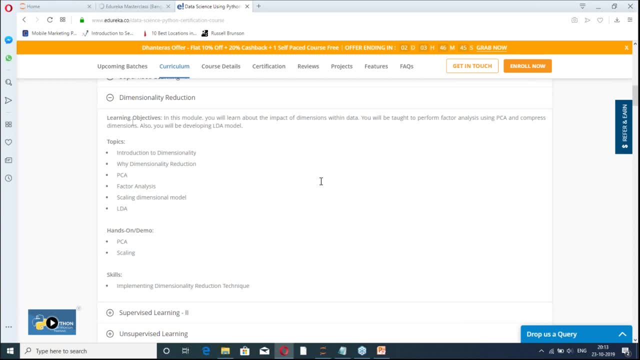 useless and it might not be possible for you guys to go through all columns and understand and try to find out which is good, which is not good. right, and in this case you need to apply the dimensionality reduction algorithm here and that is what you guys are going to. 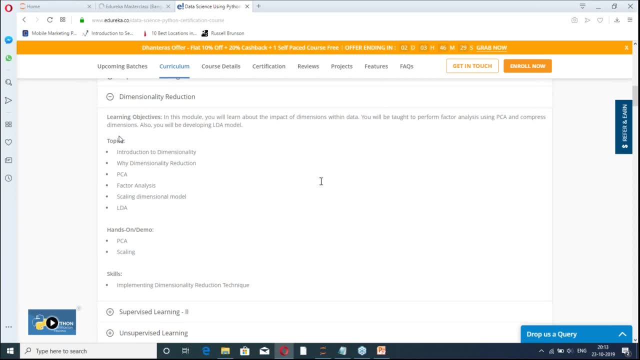 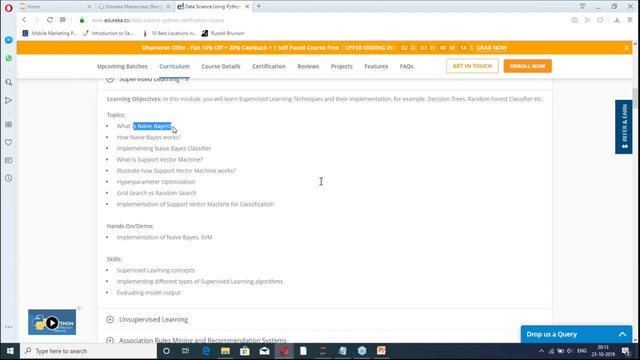 study here in dimensionality reduction how you can reduce the number of columns you have into your data set, And then you study some more supervised algorithm. so till now very few algorithms we see. after that you go to the probability based algorithm, like name based algorithm, which is depending 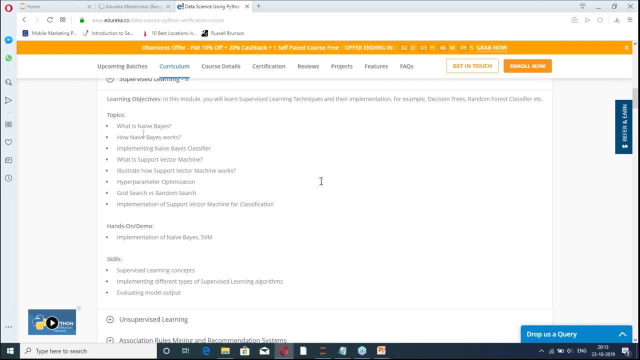 completely on the base theorem, which is one of the probability theorem, we can say: you will be implementing this thing after understanding those, the mathematics behind it, and after that, one of the brilliant algorithm is super support vector machine, and that is what you guys are going to study here. 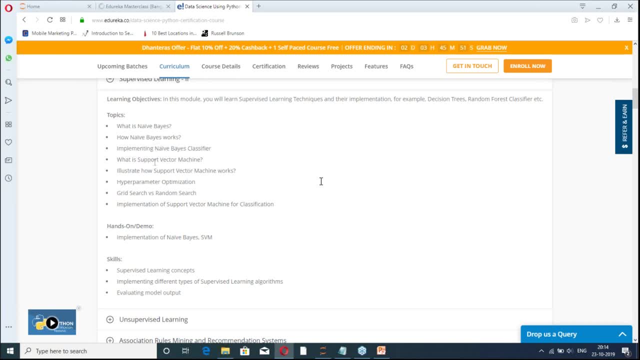 And when you, When you study support vector machine, let me tell you there is a saying about the support vector machine that you take any algorithm in the world and support vector machine can give nearly same result. whatever kind of data set you have, provided you know how to find. 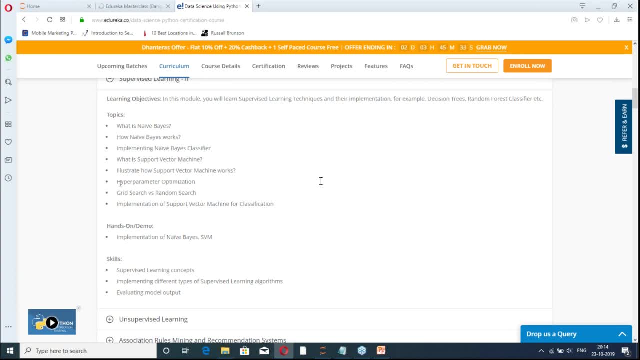 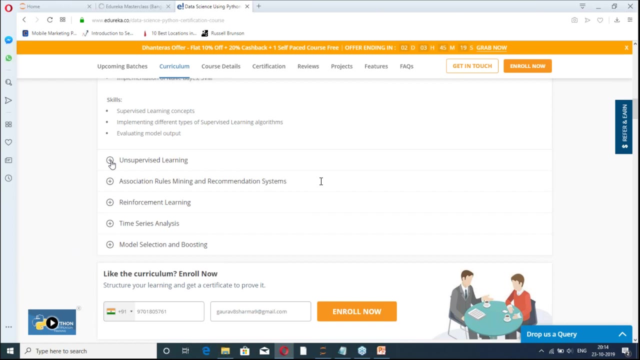 out the correct parameter and this is what you guys will be studying in the hyper parameter optimization: grid search versus random search, different, different ways. you guys will be studying here, right? So that is what you guys will be going through here and then you guys will study unsupervised. 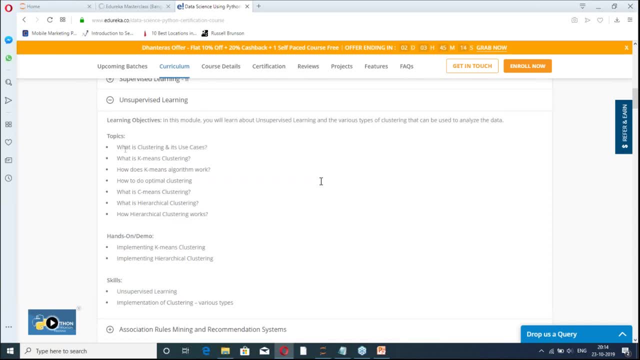 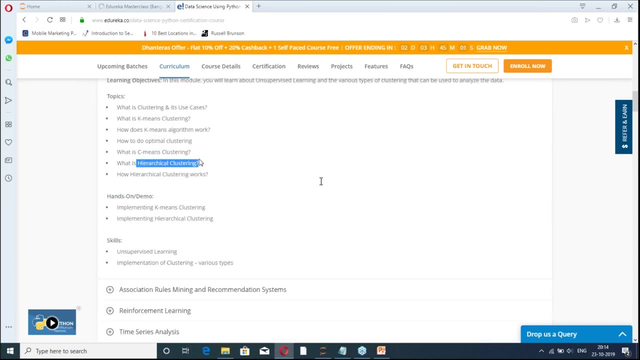 learning technique in little bit detail till now is you might have seen only K-means clustering algorithm. so you will be seeing here K-means clustering algorithm in detail, and after that you will study C-means clustering algorithm and after that you will study the hierarchical 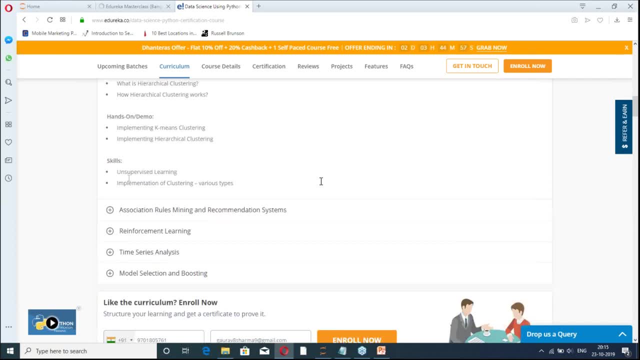 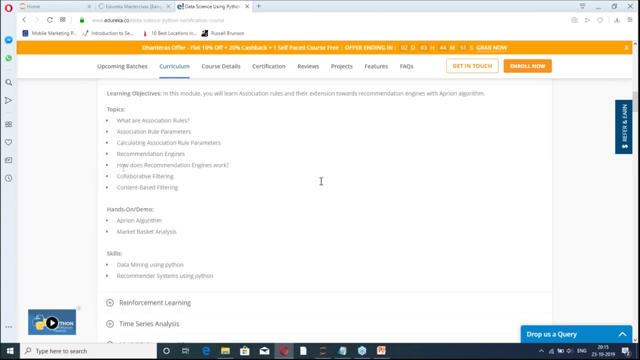 clustering algorithm as well, and then you will do the implementation of these algorithms as well, practically Right. and after that interesting part is coming right, and that is association rule mining and recommendation system. so association rule mining, let me tell you very quickly like you have shopping malls where you cannot make the recommendation system for each and every. 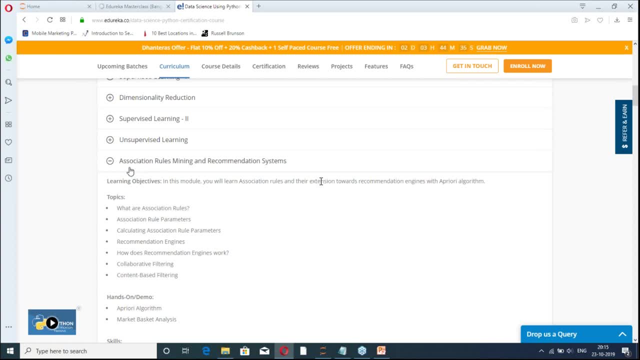 person separately. there you use the association rule, mining, right, and that is what you will be studying first of all and that you will study the recommendation system. and recommendation system is Right. That is doing the recommendation on the internet, right? you see the Amazon which do the recommendation. 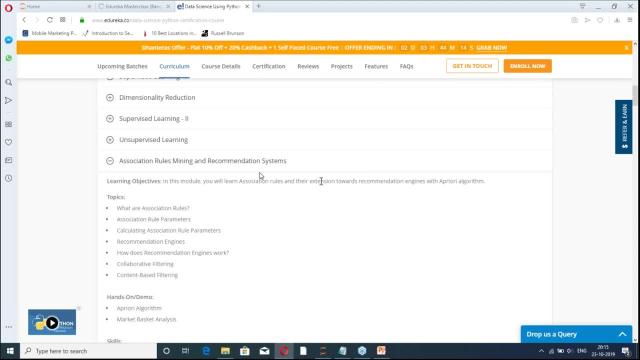 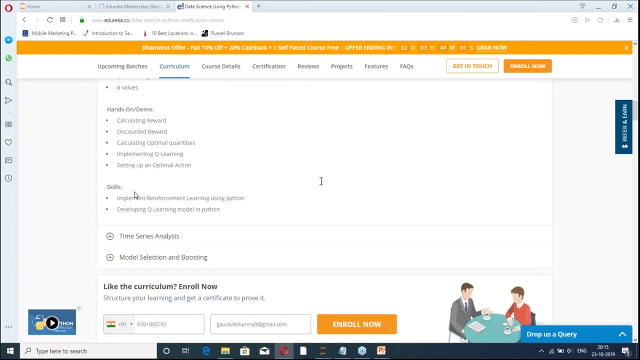 you go to the YouTube which do the recommendation, you go to the Netflix, which do the recommendation. so you will be building some recommendation system yourself, right, and that is we doing here. practically you guys will be doing there, and then you will study the reinforcement learning there which we are going to study today also here, and definitely we will not. 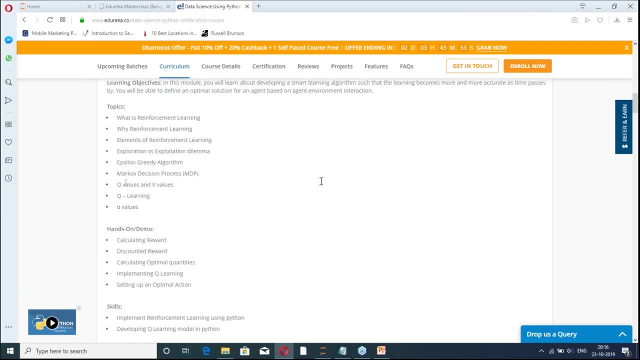 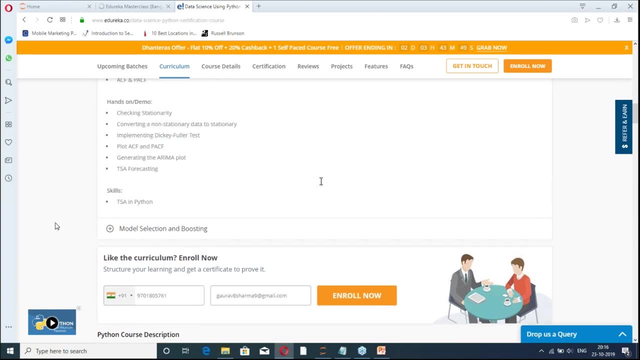 be able to go into that much detail, As much it will be taught during the class and after that time series analysis. so some of you guys have studied it yesterday but we were unable to go through the complete thing. like we didn't discuss about the ACF and PACF right, we didn't discuss about the 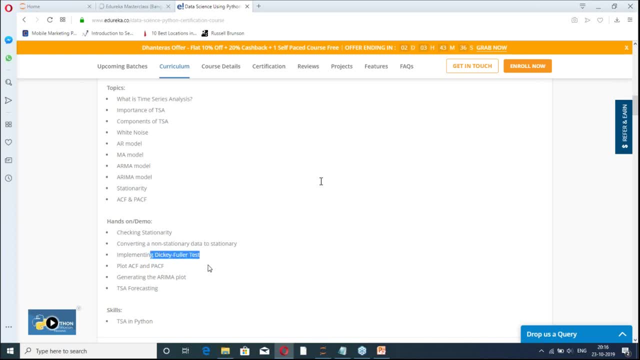 Dickey Fuller test right, how you can implement the Dickey Fuller test right, how you can plot the ACF and PACF. so these extra things will also be taught to you guys so that you guys would be enjoying those session And at the end you will be studying what is the right way of training your model right. 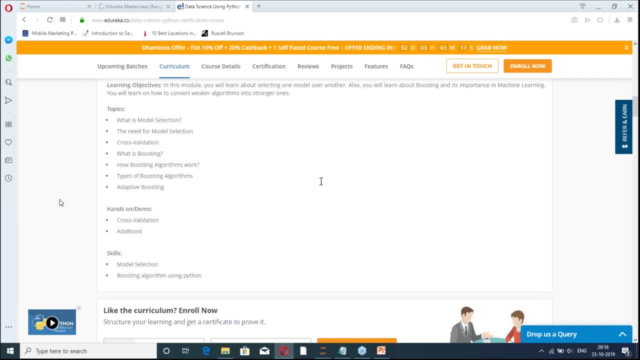 so till now we are just using the method which is taught. you know. we are using the method which we just trained: test split function. till now we have been using right. so if you guys have gone through earlier right and in the future here, you will be understanding. 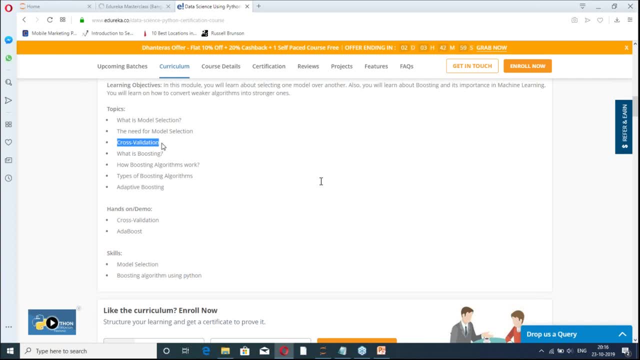 that that is not a very good technique, but cross validation is a better technique. there are some issues. We are just doing the randomly trained test split, so that issues we will be discussing and then you overcome those things using the cross validation. after that we will discuss. 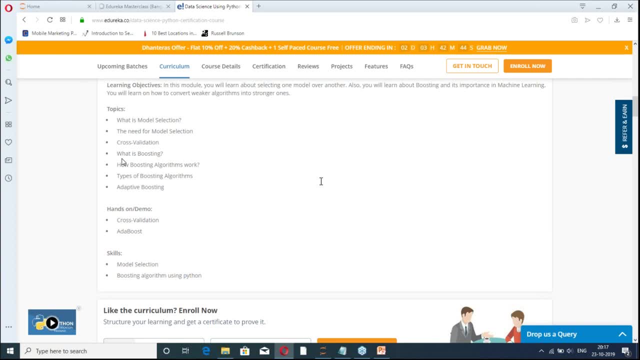 let's say you will try different, different model, but still you were unable to find some good model right and they are not giving very good result. then you will study the boasting algorithm here, in which we will be discussing about how you can improve some algorithm. if you are not getting a good accuracy, what shall you do? how, what methods to do? 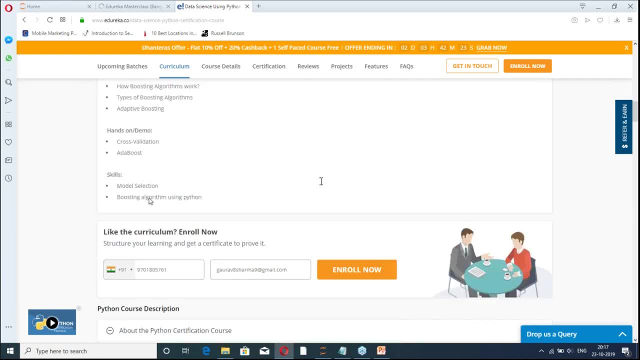 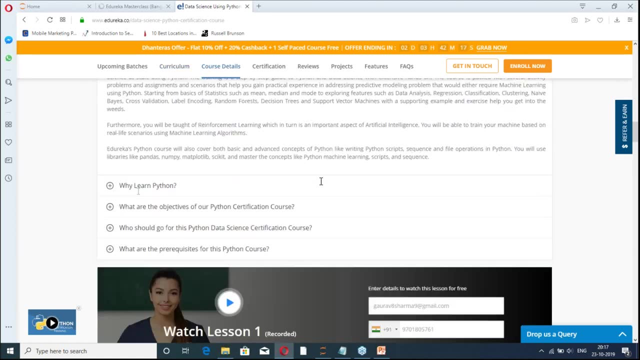 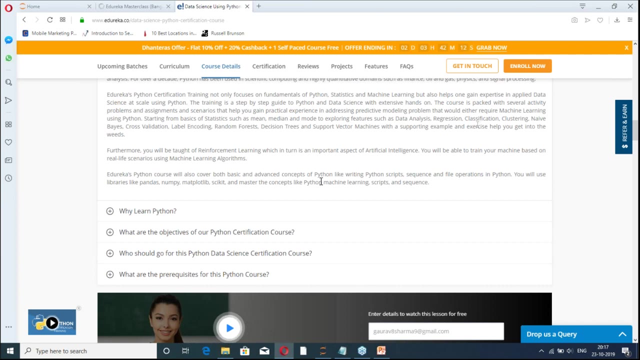 So that you can improve the accuracy, right so? and you will be doing all these things, particularly with some projects, at the end you need to do some project as well, right so? certification projects are there, which you need to do. two, three projects will be given to you which you guys need to complete, and after that you guys will be understanding. 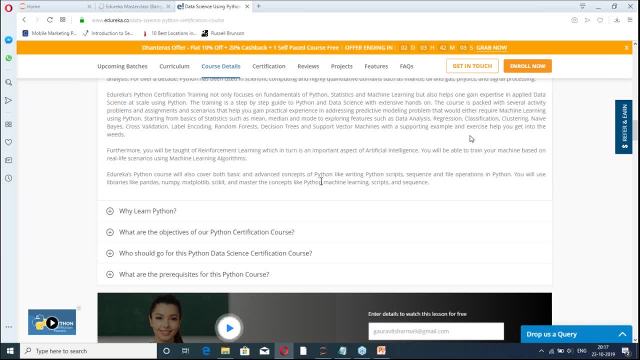 all these things okay. So I hope so this is clear to all of you guys and let me tell you, if you enroll for this session. And let me tell you the good news here. there is a good news if you guys enroll for this course and because you guys have gone through these webinar regularly so you can use this. 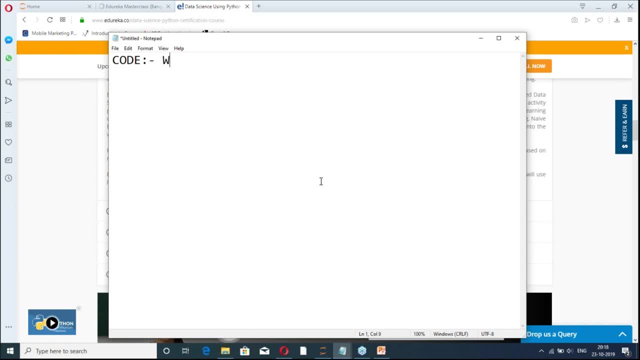 code. I'm giving you guys this code. if you use this code- webinar 25- then you will get flat 25% discount and definitely it will help you a lot and you will be getting the certification from adbutecacom, One of the very one of the very famous. who certificate has a lot of value in the industry. 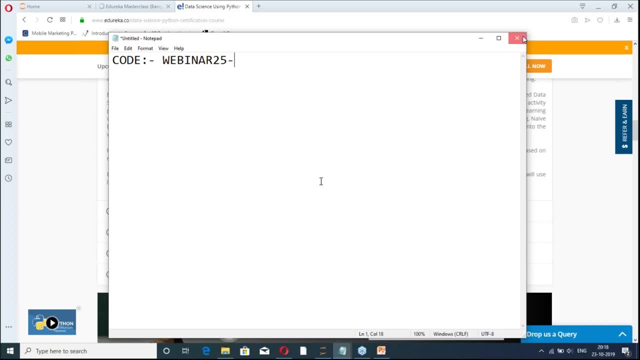 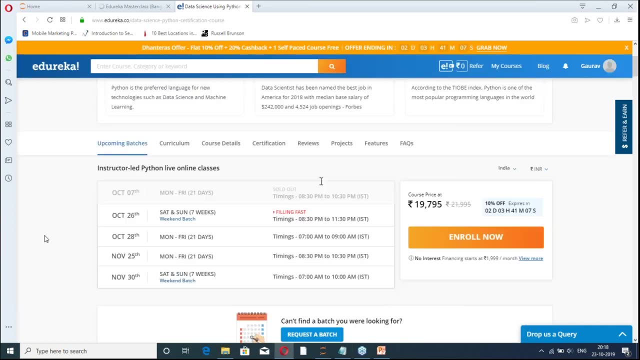 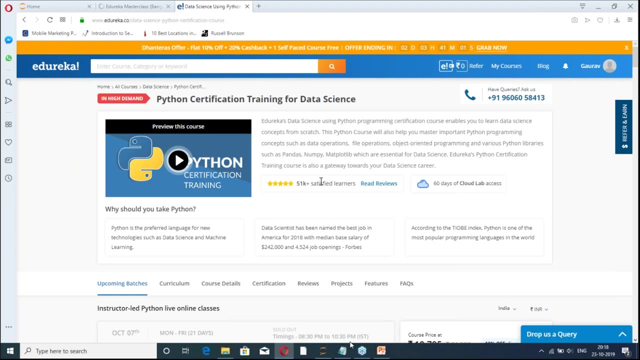 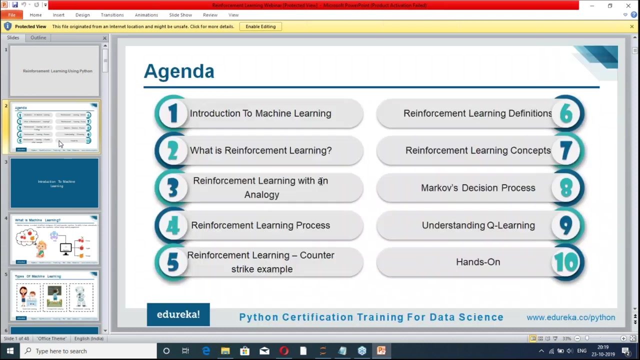 Okay, so let's start the today's session. that's all for today from the point of view of discussing about this course. right, and let's talk about now. let's start the session that is our reinforcement learning using python. Okay, so here we are going to discuss about. we will see intro. we will have an introduction. 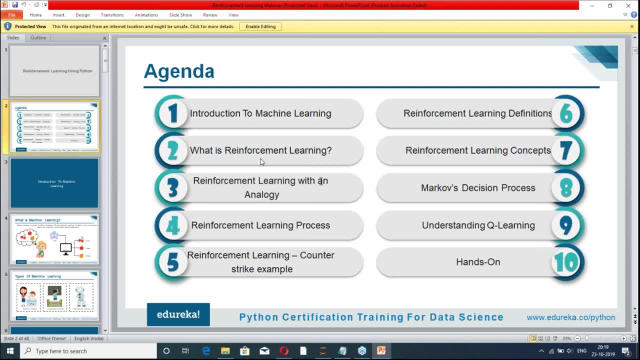 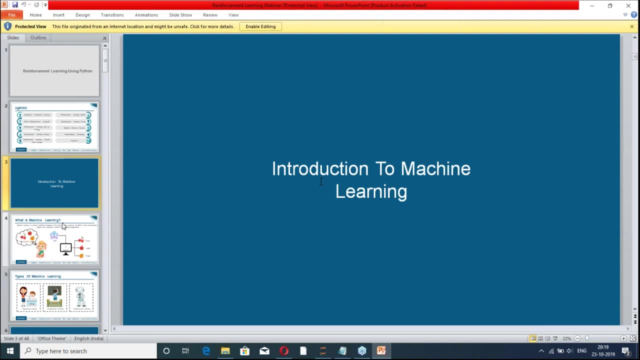 to machine learning. then we will discuss about what is reinforcement learning. we will start about some of the analogy to be used. okay, let's start better than, rather than discussing this thing, we can start the session and then you guys can see all these things. okay, so let's go. 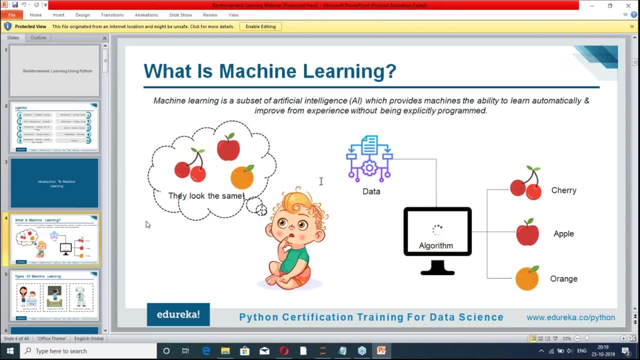 So let's start the session and talk about the introduction to machine learning. as you guys might have already understood, machine learning is all about teaching your machine right the way the human being learns, so the way we can take the decision, the way we can recognize the things, we want the same intelligence to be given to the machine right, and we give 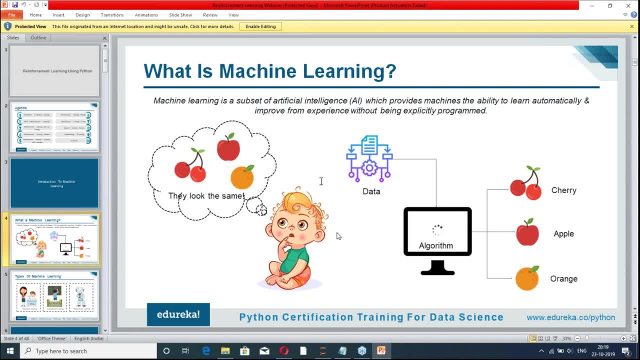 them intelligence. the good thing is that they can do a lot of processing in the parallely, a lot of data, so they have some extra features right. So all aim is the machine learning. So let's start the session. We have align, the machine learning feature, which can be used for tuning machines, so we 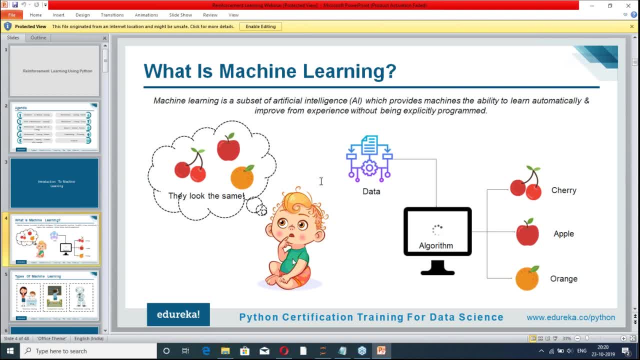 will speak about which machine learning feature could be used for tuning machines and then how to do that so that it can become like us. for example, to a child, if we show different, different fruits and we tell them how which one is which one, then slowly and gradually child will learn, and later on the teacher. if we ask any child which fruit is, 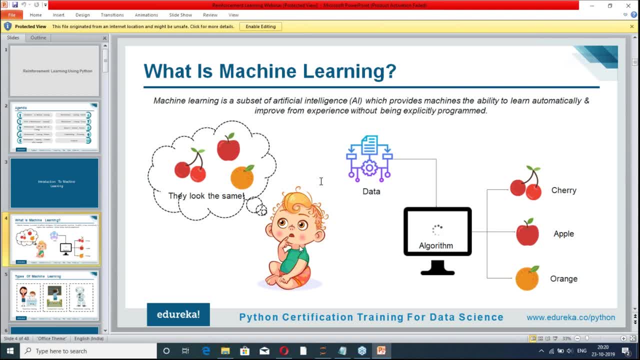 which one is. she or he will directly state: this one is this fruit right? and you doesn't need to tell the features of the fruit. you just show the fruit to them and you just tell the name and they themselves whatever features need to be expected. they will be able to do. 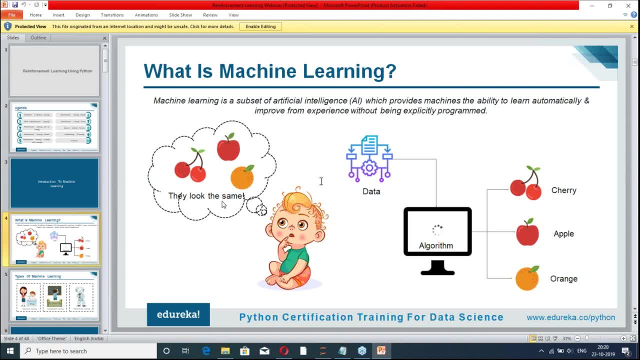 it. We now have the process. Okay, do them themselves right. and similarly, in the same thing with the machine learning when we are bringing. so there is some kind of algorithm to which we give the data, like we are giving the images, and while giving the images we are not telling that what they should look into the image. 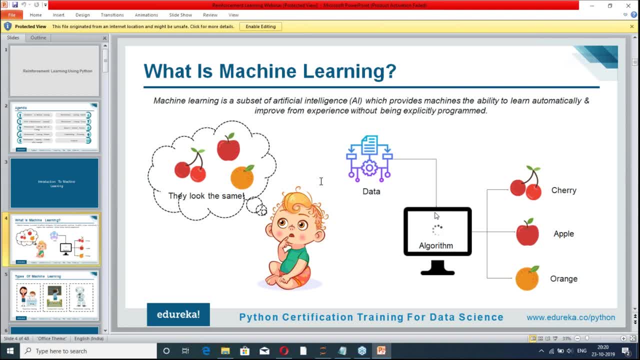 but we are telling just that this image belongs to this particular fruit. this image belong to this particular fruit, then automatically it will try to find out that what things belong to. now, what kind of features are there for which view right? we doesn't need to explicitly tell them. 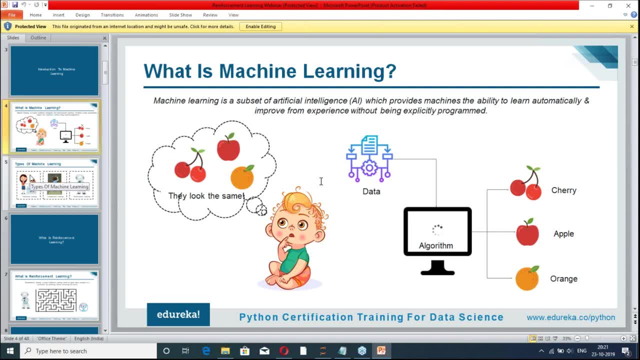 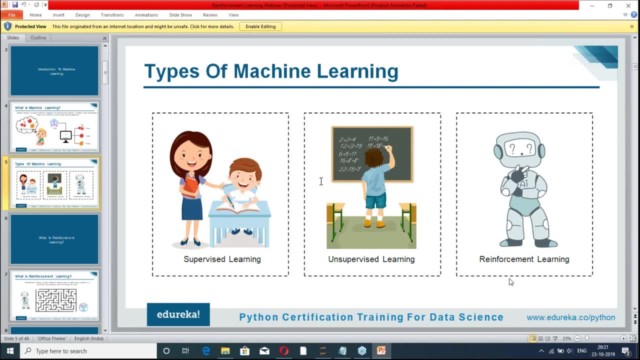 that, which features are there for which view? so let's talk about the different kind of algorithm we have. we have the supervised learning algorithm. we have unsupervised. we have enforcement learning. as you guys have already taken the earlier lecture attended, so you guys might be knowing already. 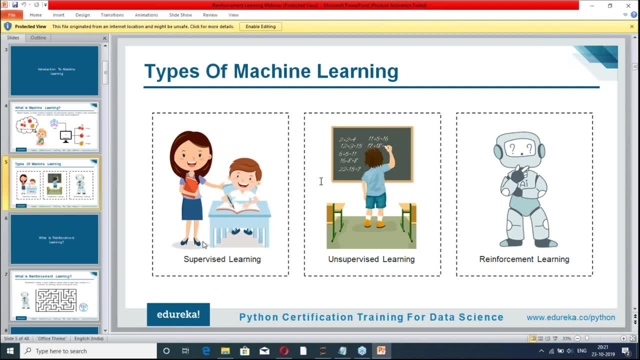 supervised learning technique is all about telling: uh, teaching the machine with the help of some supervision, right? so same thing as a mother or teacher is teaching a student, right? so they give the example, they give the question, they give the solution right. a teacher is showing them exactly this is the question and for this question, this is the solution. then the student is learning. 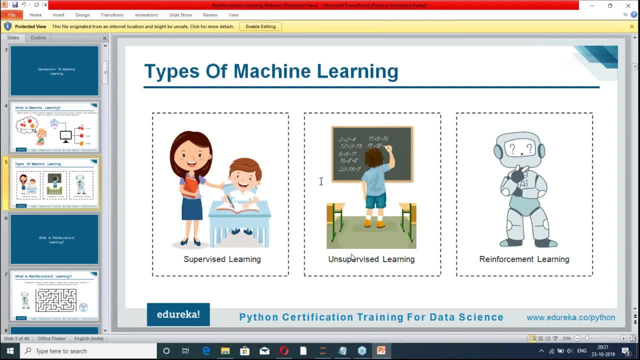 right. so this is supervised learning, unsupervised learning. nobody is there to teach you right. you have to learn yourself. they just give you the questions and all let's say in the short: i am telling this thing. it is not correct. it is more so in the short way. you can say nobody is supervising. first thing means they might be. 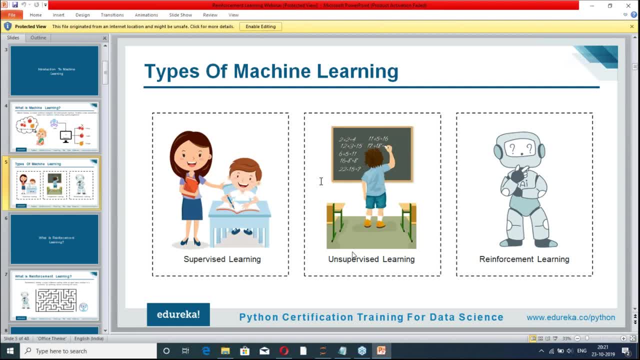 showing you the images, but nobody is telling that which image belong to which field. right? so if this is the case, then this is the unsupervised learning, we say, and mostly the aim for unsupervised learning is clustering or grouping of the items. and after doing the clustering and grouping of the items, 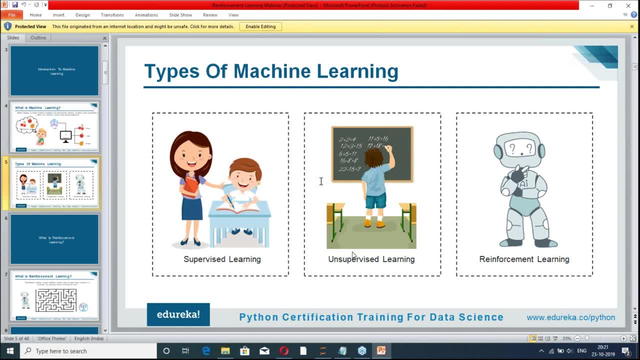 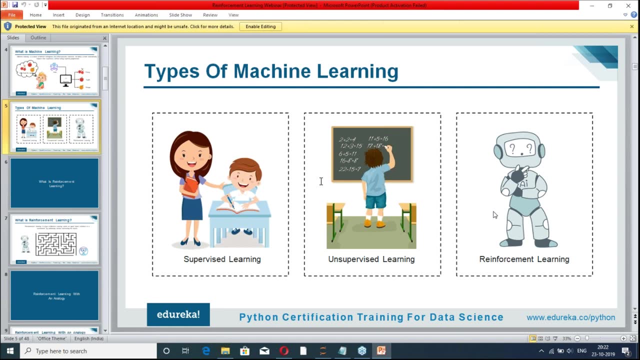 then further, you can bring out some application out of that right. so that is what we say as the unsupervised learning, and the next one is the reinforcement learning right. so let's go and the reinforcement learning which we are going to study, and i i told you already in earlier classes that 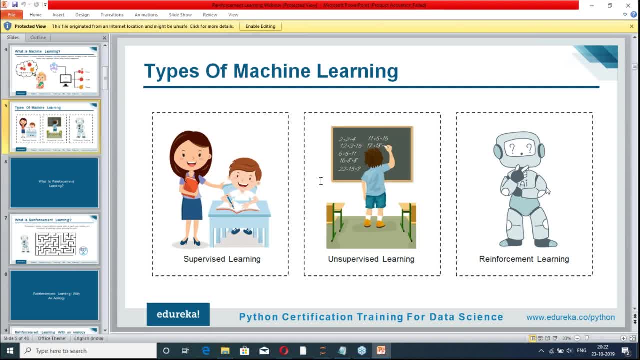 reinforcement learning is all about teaching the skills to the uh machine. right, skills, like we have these skills like driving skills, painting skills, playing skills. right music, creating music skills, these kinds of skills right, which, which is more like an art right, rather than just saying being logical, completely we can say this is art as well. right, which we want our machine to learn. right and 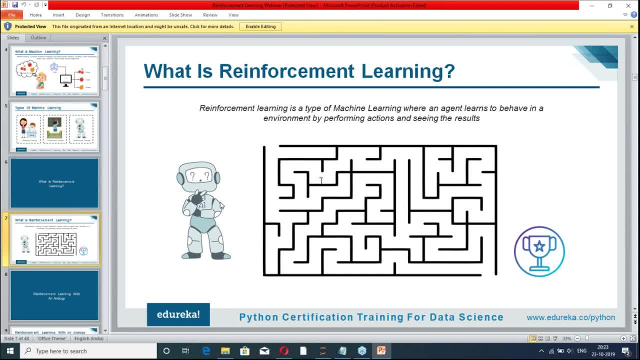 that is what reinforcement learning is. maybe we want this. so we let's say we give the major to it. if you guys might have seen during your childhood, if you leave a mouse into the maze they will find out the route properly. let's say, here you write something to eat for them and they will find out. 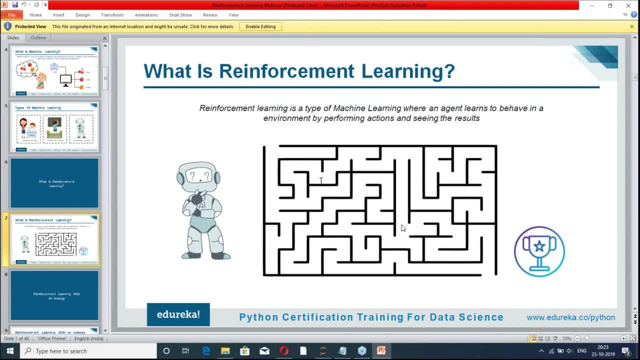 a proper route for them and they will be reaching to this particular route and they get the price right. so it will be learning exactly the path, not only just finding the- uh, you know the best the route reached first time to this, but it will also learn all the path, from which path it can. 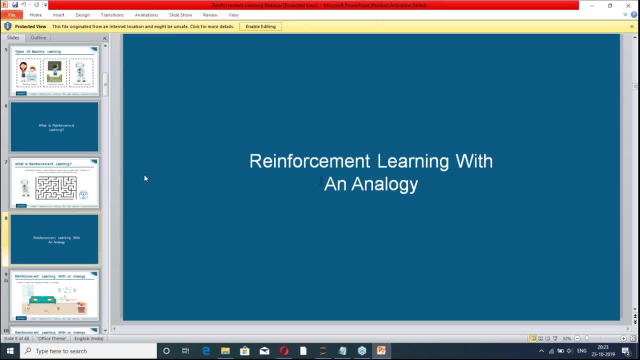 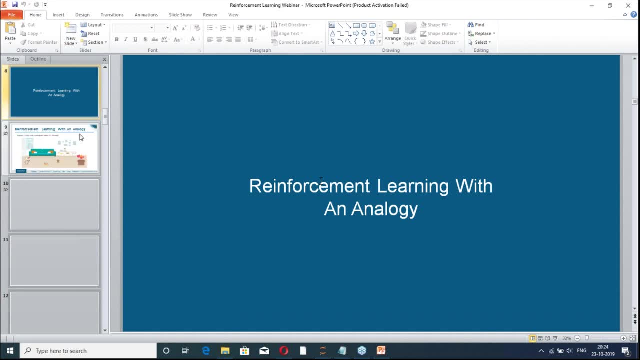 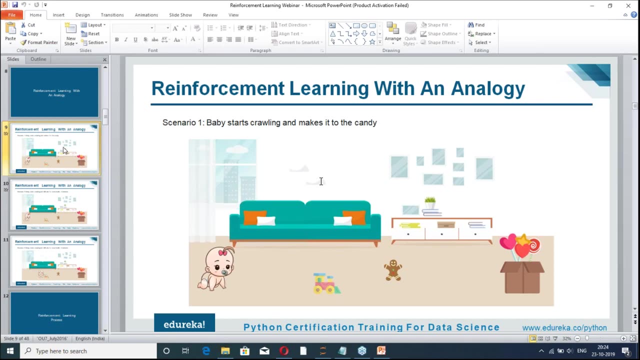 reach to which place? right, this is the very easiest things we are taking, talking about in terms of skills, right, let's uh see the reinforcement learning with some kind of analogy. so let's say, first of all, we want to, so how does it do it? so let me tell you one more thing. 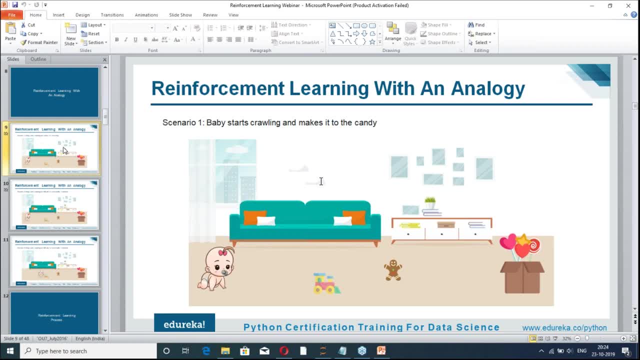 it do it on the basis of uh, feedback, it gets from the environment right. so like, if we talk about the human being, human being get the feedback from the environment. let's say: if a child is doing something and if he do it something correctly, you can get the feedback from the environment right. so let's say: if a child is doing something, 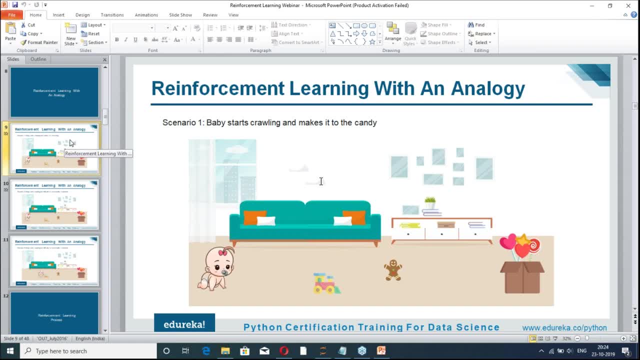 that parents will clap, may appreciate it, becomes so happy, may give some prize, anything like this. right, we are reward, rewarding them, our child, and similarly, whenever your children or child do something wrong, you become anger on them. right, you might beat them, give a slap on their face, just. 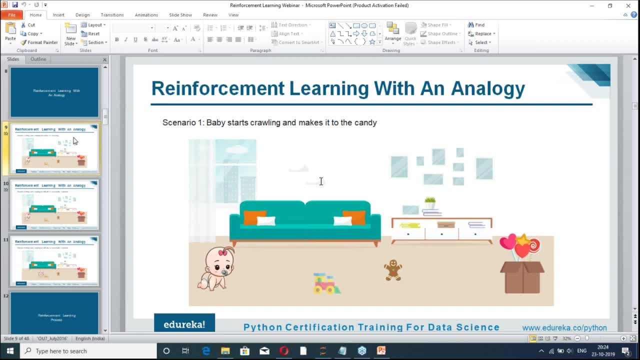 kidding, right, you don't need to be that much harsh, but you use here some of the feedback which, using, which your child is understanding: ah, i did something wrong, and they understand. and then they are learning that in which particular condition or context or the environment, what particular kind of action they are supposed to take, right? so this is like 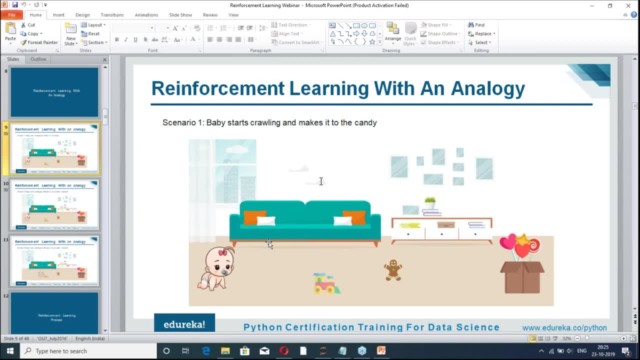 we are showing here one case like that: baby starts crawling and make it to candy, so initially baby might not be moving, but they start crawling and and they as they start crawling right, so initially they might be falling in between and because of some of the hurdles and so on, and so 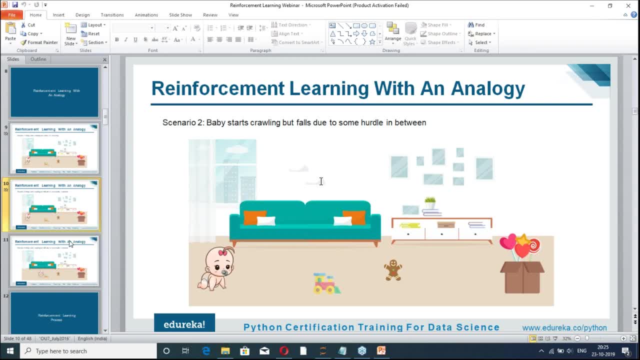 on, right then it is learning. when it is falling down, it means he or she is misbalancing. right then, slowly and greatly, then they, whenever they, you know, fall, whenever they are finding some hurdle in between, they might, you know, start finding, maybe weeping and saying: okay, this might be the 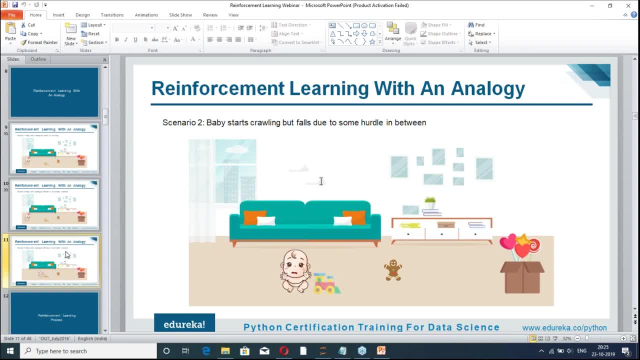 wrong path, i should choose different path. right or if they get fall down, then maybe, if you know, this is the beauty of the child, maybe the overage person, if they are learning- let's say, if a 50 year man is learning a bike and if once they get felled down he might never again. 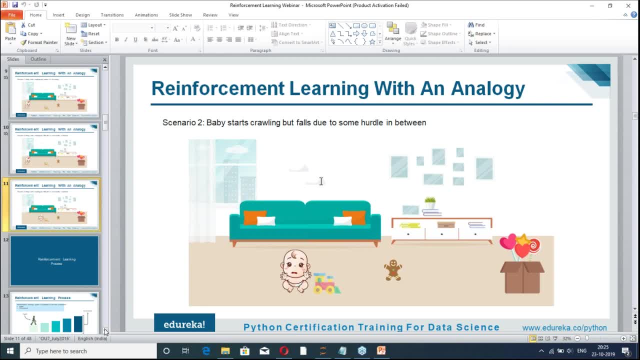 try to, you know, start the bike again, because he might. he might associate completely wrong way, but with the child they will not. they will understand that i did something wrong. that is why i fell down right and next time it will try to do something else so that it can improve. maybe it will try to. 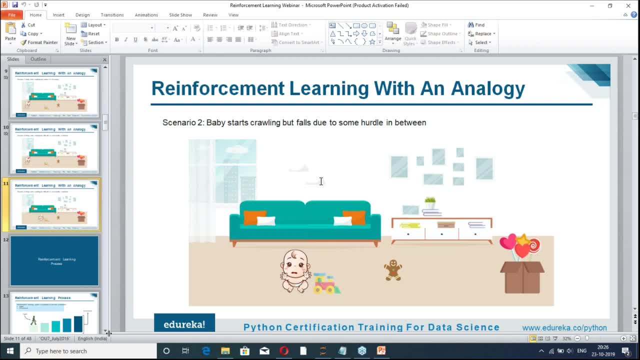 balance it back away, it might have put all its weights on the one side now in dv, or she will try to put her or his weight on the other side, right. so that is the beauty of the child and that is what we call as a reinforcement learning. once it makes mistake, then i try to find out how the 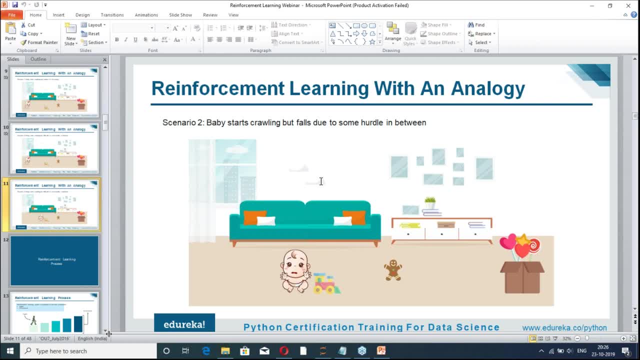 mistake is related to the condition, right, it's not because nobody knows, right? uh, without sitting on the bike, you might not know exactly how to balance it, but when you fall down several times, then you understand how to balance it. and that is what reinforcement learning do: that it falls down then. 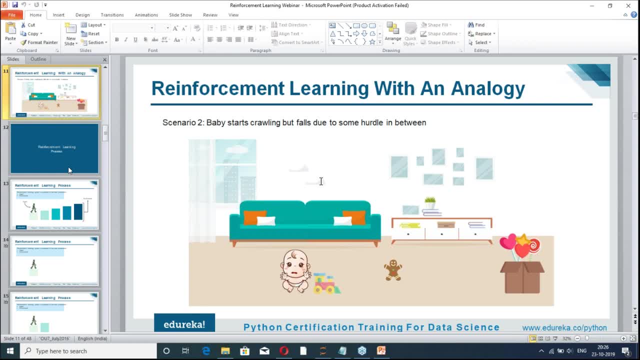 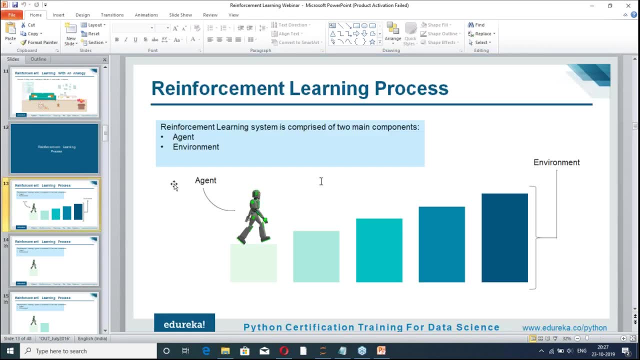 it understand: okay, this is not, i should not do this thing. then it do something else. then it again fall down then think, okay, this is also i am not supposed to do, right. so what is the process here? so we will understand that. first thing, we have the agent, right agent, like in the earlier. 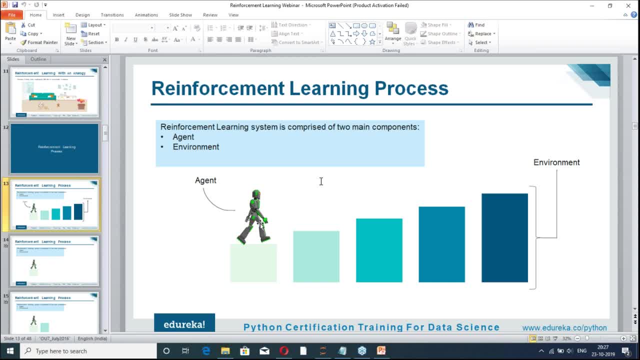 case child is the agent right, and if we are doing it in terms of programming, then the- uh, our program or software is an agent, right. who is going to take some action in the environment? right? so two things: agent and the environment. so if you are talking about the software, we need to define also the 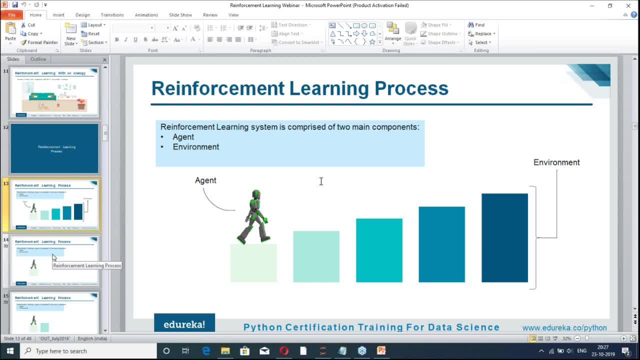 environment. right, so let's talk about further here. so we talk about this thing, we have the two components, one is agent and another is environment. then it's try to learn it is. it start taking the different, different steps, small, small steps it take and then it learns about the environment. 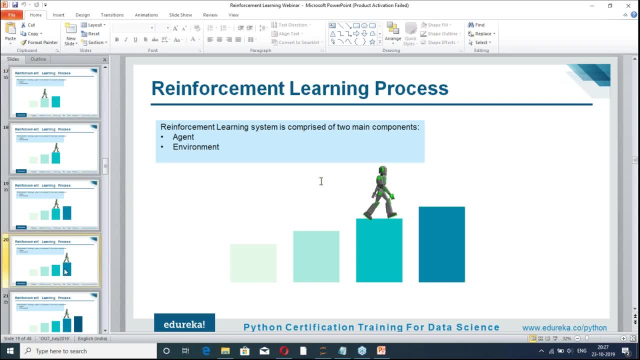 right. so as it keeps going forward, it keeps learning about the environment, right, so we have the environment right. so one thing definitely: and how it is attached to the environment, it should know. but when it takes some action, how the environment is behaving, then that is what it. 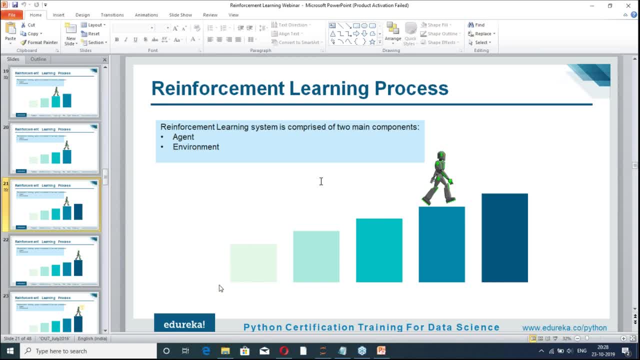 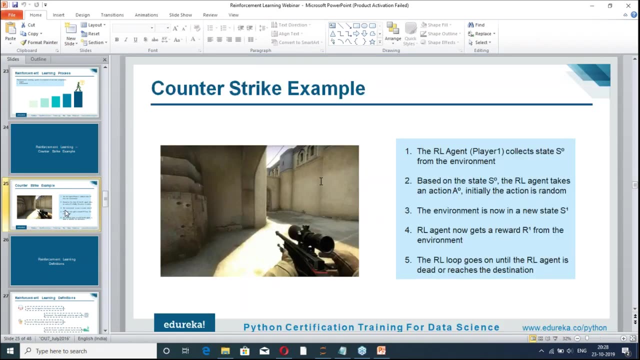 is learning, so it learns from the small small thing. initially it learns very small thing, then it start building. maybe with this small small learning it start building bigger learning, and so on. okay, so let's talk about here reinforcement learning, career, uh, counter strike example, right. so so here, uh, let me tell you one of the very good algorithms. uh, like like you can make the 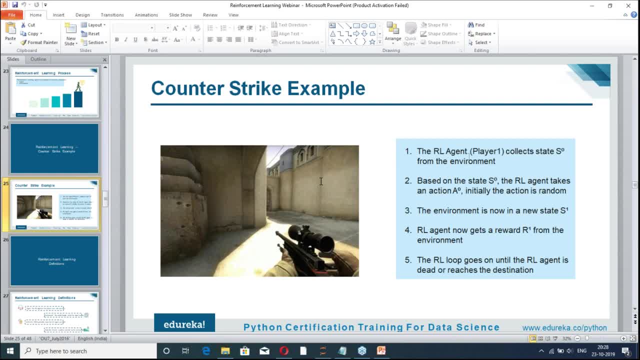 counter strike game players to learn on their own right. it's, uh, not about the human being, right? it's not about the human being who can play, but the computer can play also. pretty well, right, and you doesn't need to write it explicitly all those four, but you need to make sure that the computer can play and you don't need to write it explicitly all. 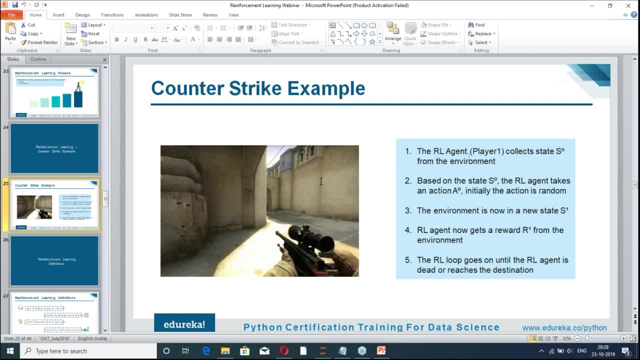 you need to make your system learn automatically by playing right. the way human being is learning by playing again and again, so same way the system can learn playing the game. so here you see this: uh rl agent player. one collects that state as not from the environment, so whenever. and so how does it do this game, how does it play or how does we behave right? first of, 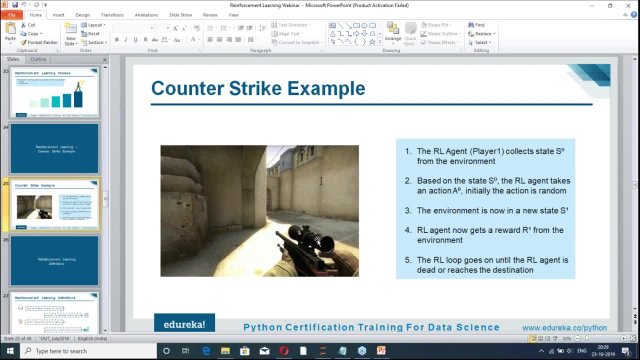 all. we need to look around us. what is the environment? we are collecting the environment first of all. right, we are seeing exactly what is the things are there in my environment because, on the basis of the environment, i am going to take the action. in different environment i take different 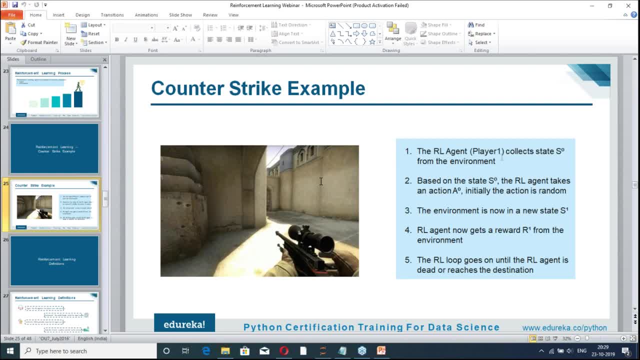 actions. so, similarly, here they are saying that the agent is collecting the state as not from the environment. that is correct. sorry, connect collect, sorry. current position of the environment: right, current position of the environment. and we are calling initial position of the environment as the s naught position. then, on the basis of this s naught position, or which is the which is we are, 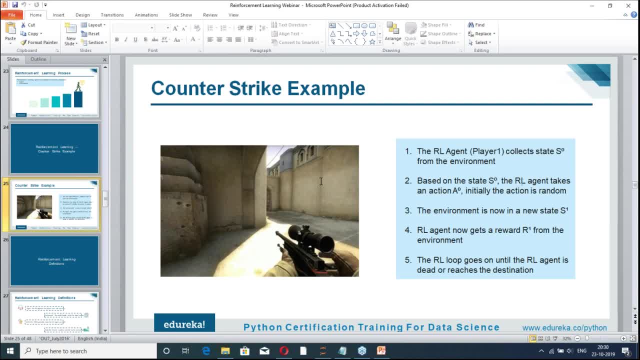 calling as the initial position rl agent, our reinforcement learning event, or software or the program which you guys are going to write, take some action, a naught right. and this action it is taking completely random. it doesn't know which action it should take, it is having lots of action. 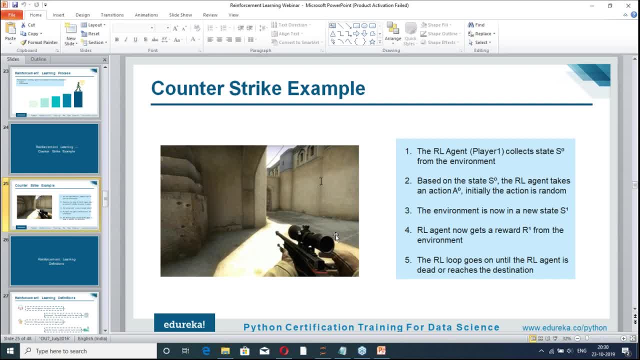 to take. it may move forward, it may go backward, it may take left, right, it can set its um, it can set its gun, it can fire the gun somewhere randomly, completely or maybe by pointing to some players. so it have lot of action to take in any position. so it does not know initially what action it. 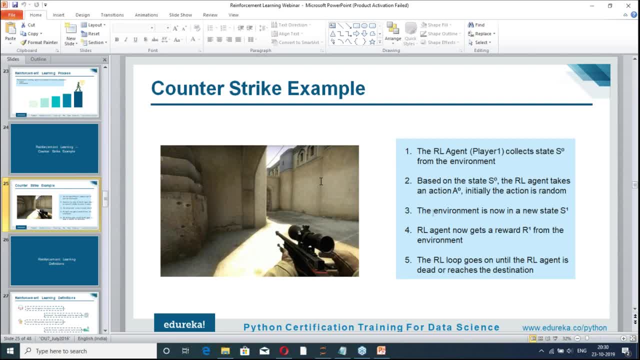 should take so randomly, take some action out of it and after taking this particular action then the state of the environment changes. right, it might happen. let's say, if you have moved forward, then maybe you will get different visual now. or if you move backward, maybe different visual if you write, take left turn, or even if you are staying at your position. this is again some. 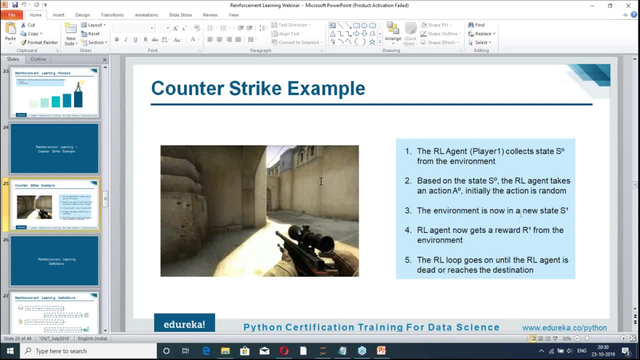 action right, that is, staying at your own position, and sometimes still the environment may change because the opponent player might come in front of you, maybe from the back or the left side right. so the state of the environment is changing, and as the state of the environment is changing, 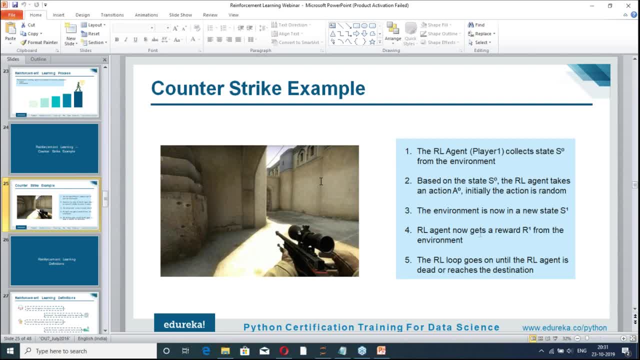 then again, really the environment is changing and the environment is changing and then again, really reinforcement learning agent is learning from it and with this it is getting some reward right- reward or maybe punishment right, or sometime reward might be zero as well. it may be positive, negative or zero. let's say: you stay there, nobody came from the opposite side, you didn't hit to. 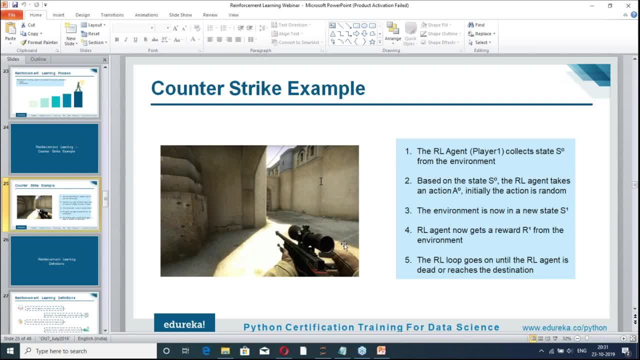 anyone. where, then zero reward, neither positive nor negative. but let's say you hit somewhere, your he shoot somewhere, then it hit the opponent player, then you got the positive, uh reward. if you has been hit by the opponent player, then you get the negative reward. so whatever action you have taken, on the basis of that, some reward you are getting. 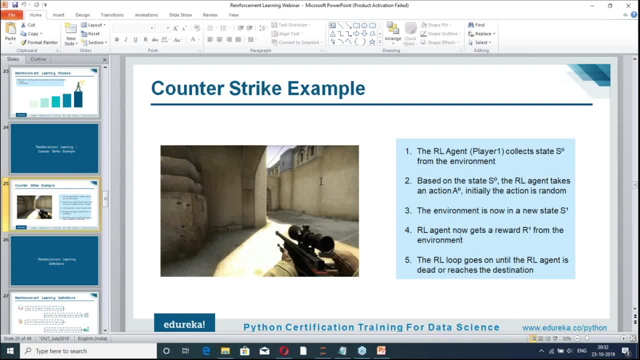 and then it gets that reward and on this basis of this report, it understand the action which has it has taken into this kind is uh, into this particular condition. it learns whether it's a right or wrong or it is neutral action on the basis of the reward it is getting. 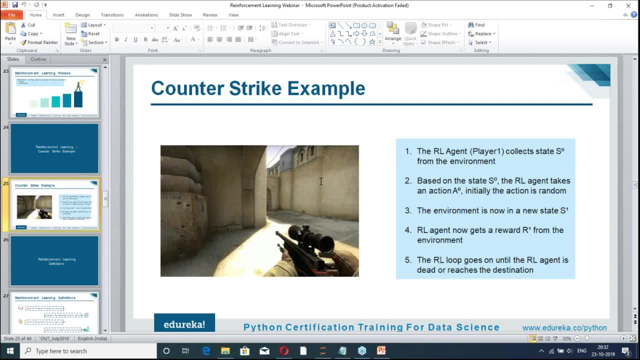 and it keeps doing this thing, right, it keeps doing this thing until the reinforcement learning agent is dead or reaches to the environment. so first time it plays it learns something. then second time it plays again, learn something little bit, limit little bit. so, after taking different, different action, it is learning and making the connection between the action and the. 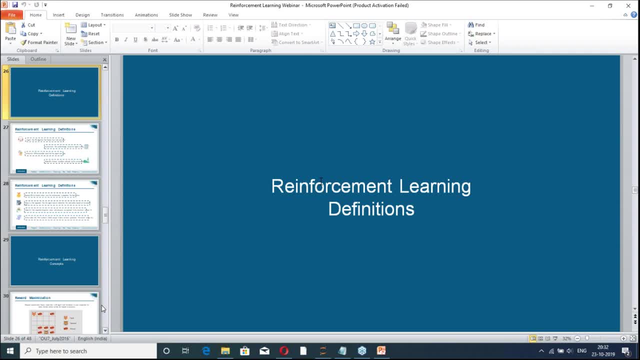 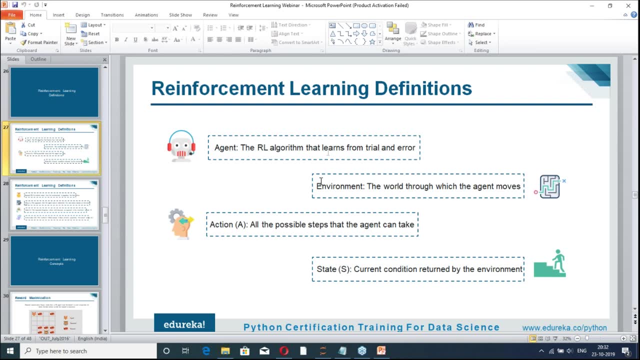 context. okay, so let's talk about the some of the definitions. so we have the have the agent. agent is the one which is learning. we can serve a software which is learning from trial and error. then we have the environment, which is basically our environment. only, like we discussed already about the counter-strike in 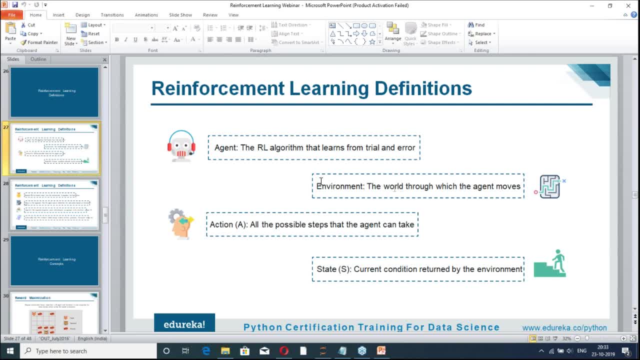 which the walls around the opponent player, everything where agent is performing, even the agent is itself the part of environment right. everything, action, all possible stuff that agent can take and that might be for different environment. different possible actions might be there, because it might happen if an will, if the back of the agent is involved, then agent cannot take. 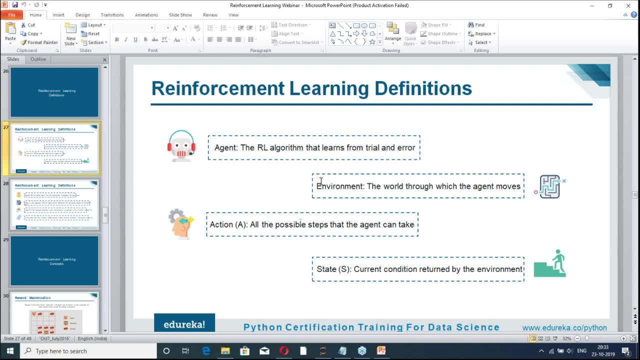 the action cannot go back side. so that is a different action in the different environment. but agent needs to know which action he can take in the different environment and then we have the state. that is how the environment. this is different. some architecture, like systems, can copy the lot. then we can. 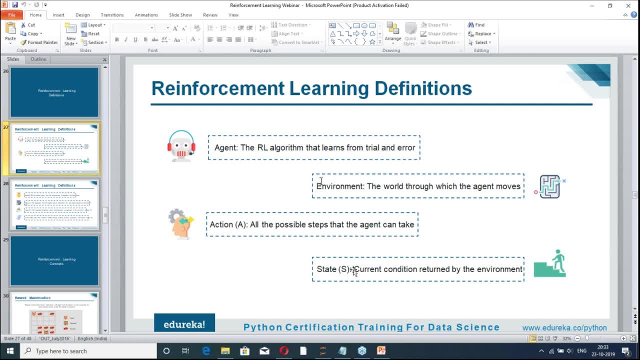 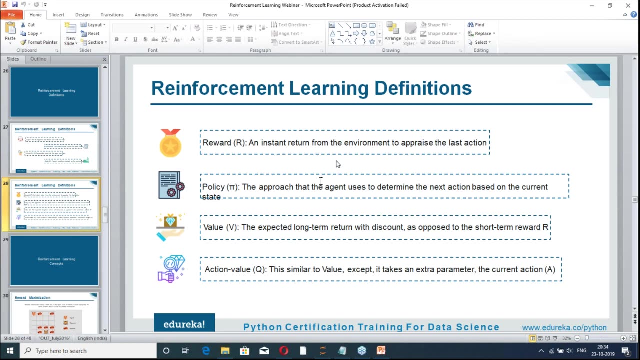 is every time is changing. then we say state is changing, state is something which agent is learning about the environment. and after that there are some more important things are there like reward, are an instant return from the environment to appraise the last action. so that is. I told you already. 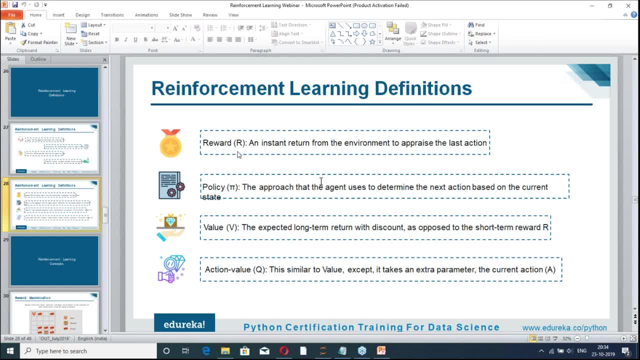 reward is the one which, using which it is understanding how good or bad action it has taken, right. so if it is being killed, that is a punishment. if he kills the opponent player, that is the reward. maybe he got plus one point for that. it's depending on. you need to define that mathematical function which would 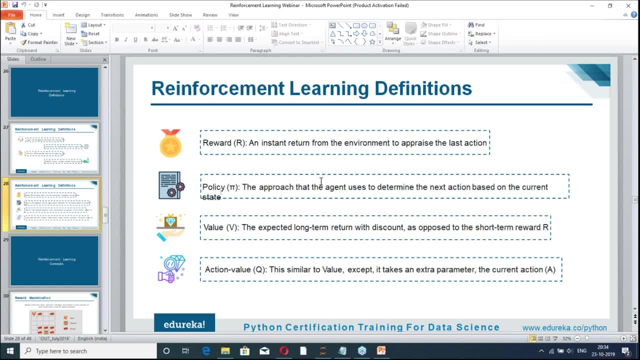 be giving the agent some kind of reward and after that policy. policy is something which agent is learning on the basis of reward and all right for policy decide in which context or environment what action to take. so what it is learning is policy, that it is learning. a policy is nothing but the but the: what action to. 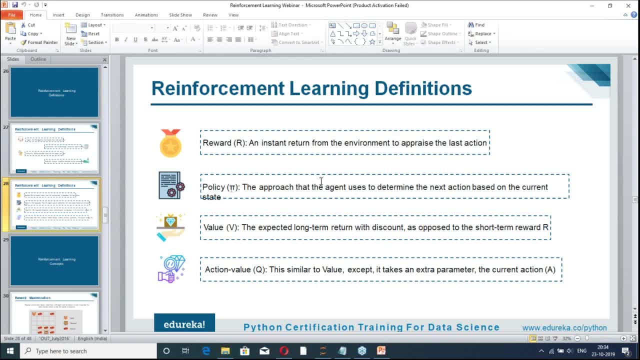 take in which particular condition, that in what policy? in each particular condition there might be multiple action. but when you learn which particular action to take out of all those given a possible option, then that becomes the forward. then we have the value function. so value function is all about expected. 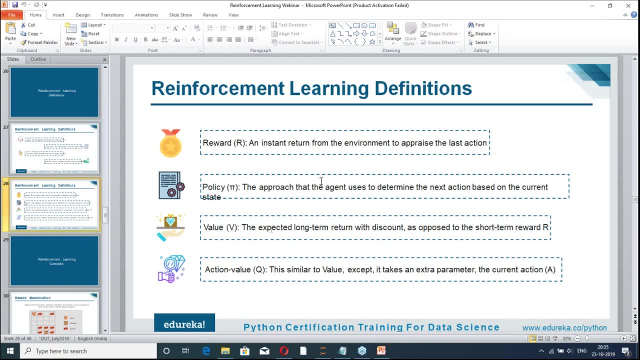 long-term returns with thisock, opposed to the short-term reward. so what we are going to say? this value is that in whichever current state you are, how good state it is means how much closer you are to your final destination right or to your goal. that is what decides. the value means in whichever condition you are. 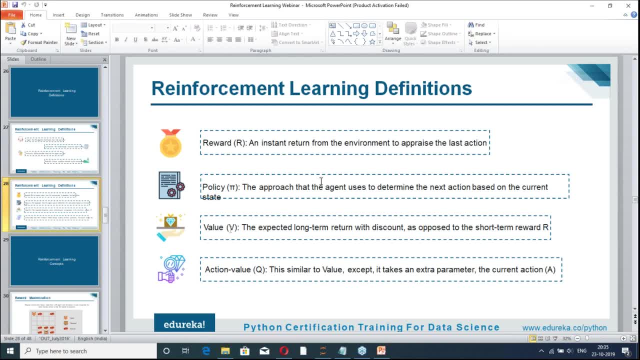 currently how good your condition is right and how much closer you are to your destination or goal. that is what is being defined by the value function. then we have the action value and we say it as a q value. q value says that in the current condition, or in any condition, if you take. 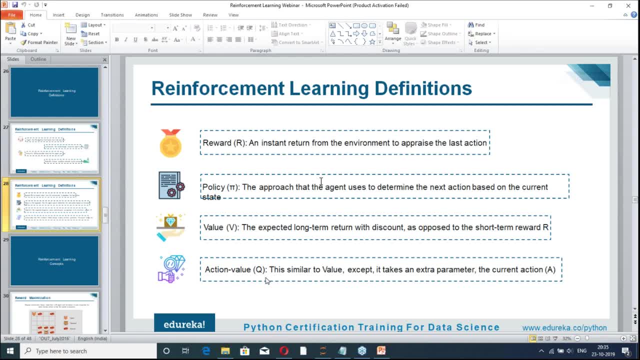 some action, how much value you will get from this right. so that is what we call it, very similar to value function. but here we are adding one more thing, that is action. that if i take some action in this current condition, then what would? i will reach to the next condition, where i will reach in the next condition. maybe we can say: 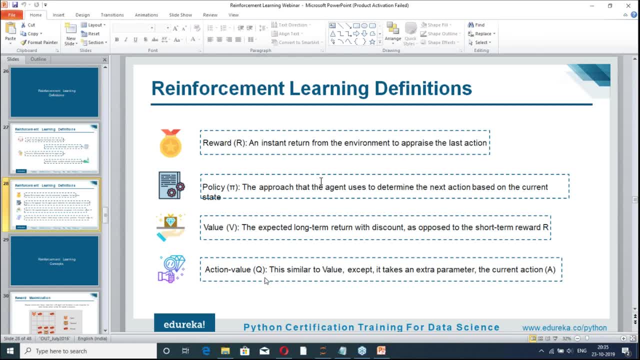 or we can say environment, and what would be the value of that particular environment? again, right. so here we are adding one more thing that is, a particular current action. so when we consider v, we are thinking the best way that is, in whichever current condition i am. if i take the 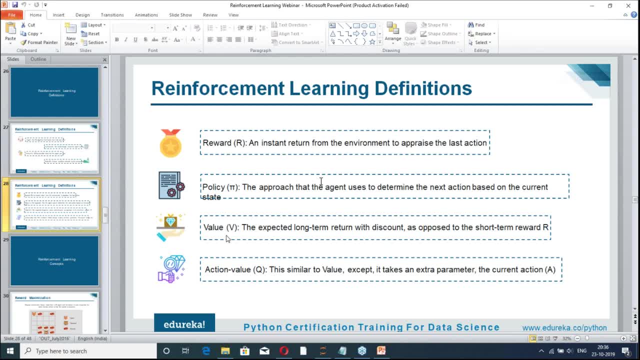 past action from now onwards, then how much reward i will get. that is value. and if i am talking about saying currently I am taking action a and action a may be passed on, may not be passed, there is no guarantee that action is passed or not, but once I take action a and to whichever state I need, 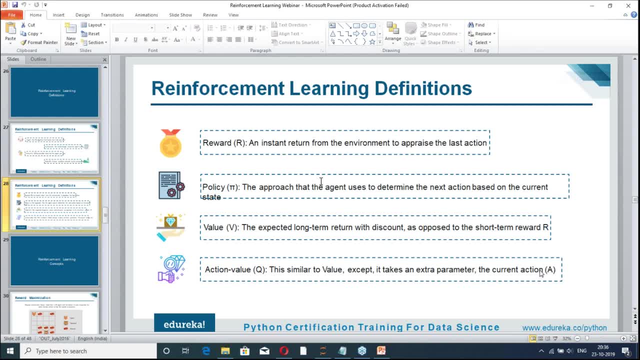 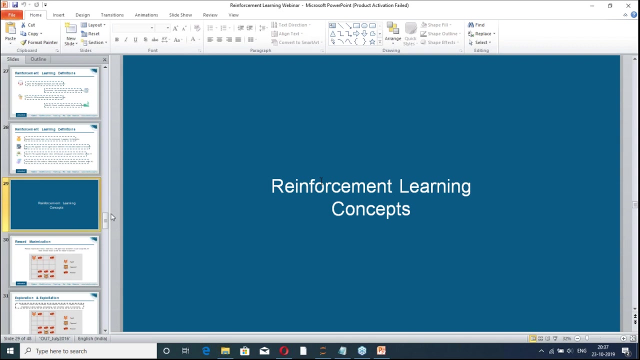 after that what reward I get, and after that, if I take the best action after that, then how much reward I will get. that is what is defined by the action value. okay, and let's go ahead. then we call as reinforcement learning concept. so the archit is asking: what is the agent doesn't learn after. 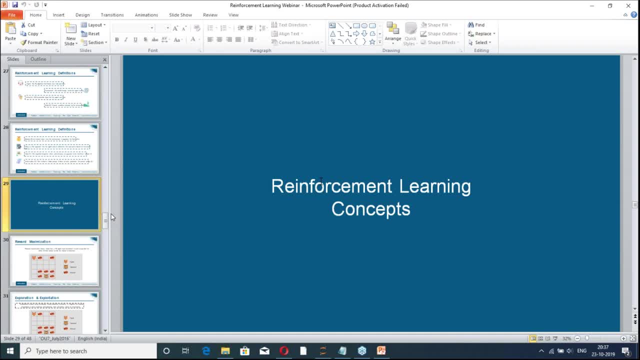 moving in the environment. takes it, take a james chasing, takes it as error. I guess no, by agent will not learn. first of all, first question is this: by agent will not learn. so the chance of learning is not learned. so the chance of learning is not learned. so the chance of learning? 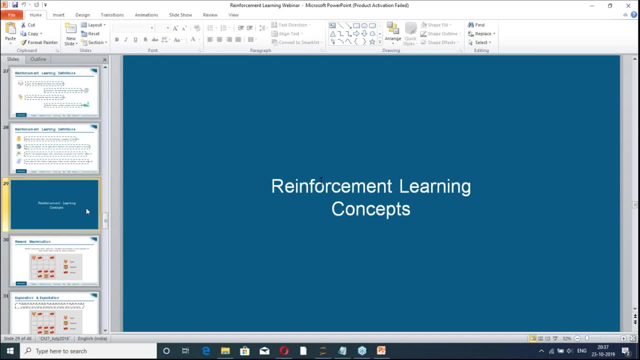 is that agent will see how much good the action is. let's say agent. let's say agent is driving the car right. so when it is driving a car it has multiple option: it can take the car backward, it can take the car forward, it can take left turn, it can take right turn and so on. so initially they 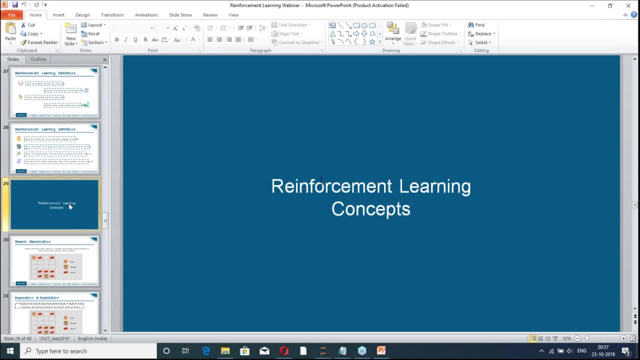 are teaching it in a simulation condition. it is not like in the real environment. they bring it initially. the car is learning into the simulation. now, when it takes action, whether it is going wrong way the action, it is taking the current condition or the right way. so if it gets it, 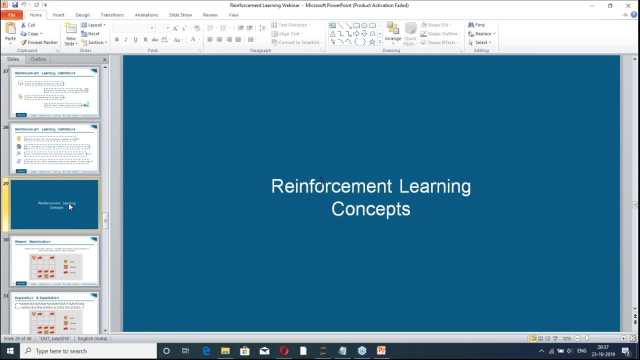 wrong way, then it unlocks, then this is not the right action. but if it goes the right way, then it learns. this is the action I need to take. so it is not. it is never going to happen that after moving in the environment, agent will not learn. agent will definitely learn above. it will learn. 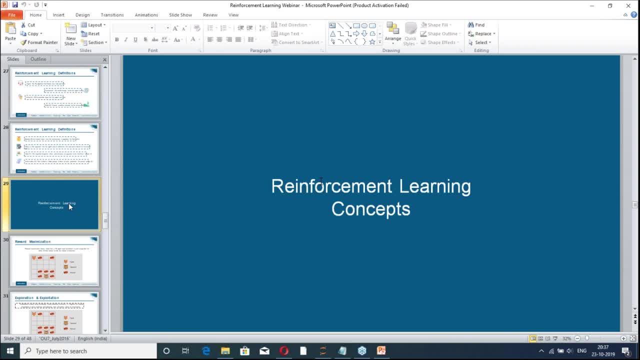 about the action which it has taken. definitely it does not know. it's still best action. it is equivalent like this: it is learning skills, right. so it is equivalent to this that let's say you want to learn some skills tomorrow, let's say playing badminton, and you go into the badminton court you find some. 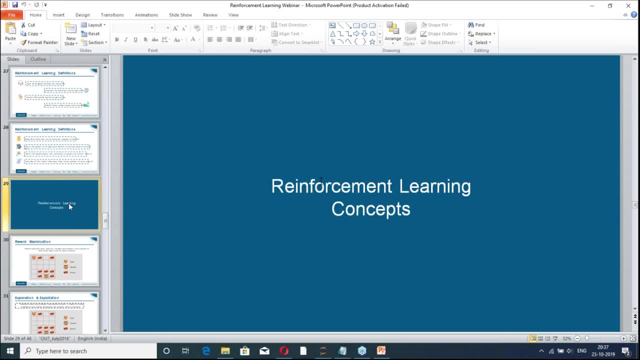 coach and you start hitting some shots. right, maybe logically you might be understanding what to do, what not to do, but still, you do not know until you do these things. so you hit some shot, let's say, and the power you put into your shot was too much because you didn't know initially how much power. 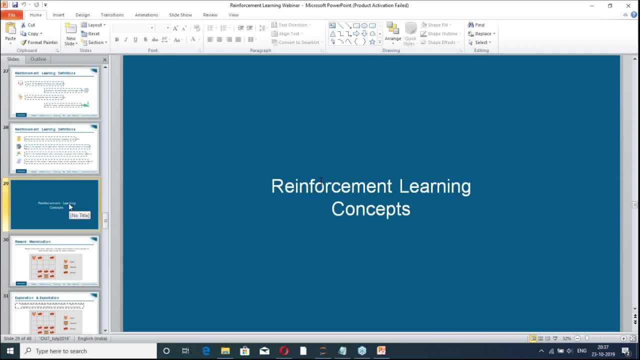 to put so as you exert your power into your shot and the shuttle cog went outside of the court now, even though action is wrong. but you learned one this thing: that i should not hit the shuttle with that much power, right and with this particular angle. so you are learning this thing right. so 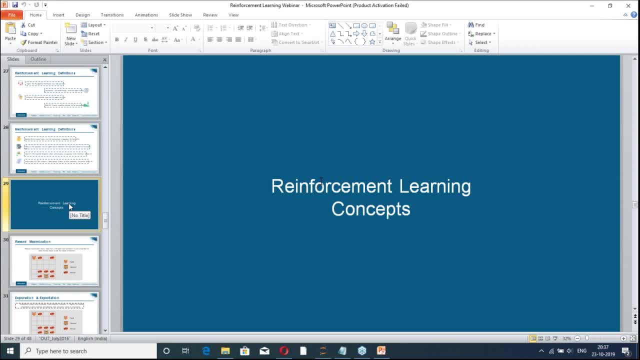 it never happened, even though it's. the power you put into your shot was too much because you didn't know initially how much power. there is a lot of possibility. you might not learn what is the best action to take, what is the best power to take currently, but you learn what not to do currently, right. so same thing with the. 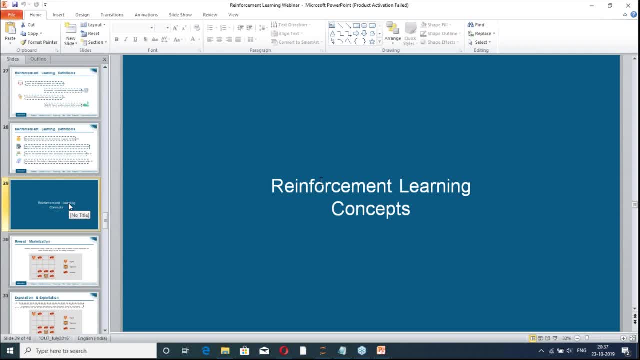 reinforcement learning. so next time it will try with this some different action right and how it is doing. as you are knowing from the uh- that is your reward system- that whenever your shuttle is going into the right place, then maybe your coach is appreciating or your eyes are looking at it. 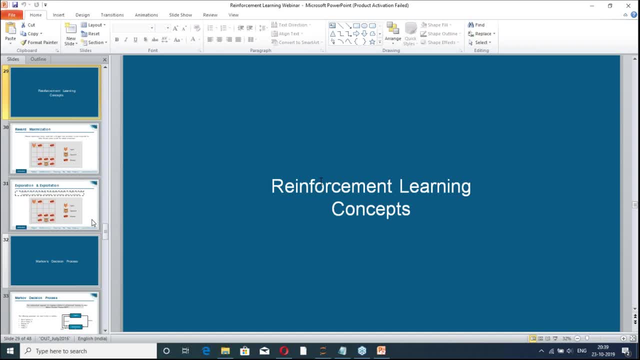 and you are understanding whether the shot was placed in the right position or not. right, so it gets the feedback. so it is never gonna happen that it will not learn, whether it will learn whether it's the right action or it's the wrong action. okay, the urchin? i hope so. 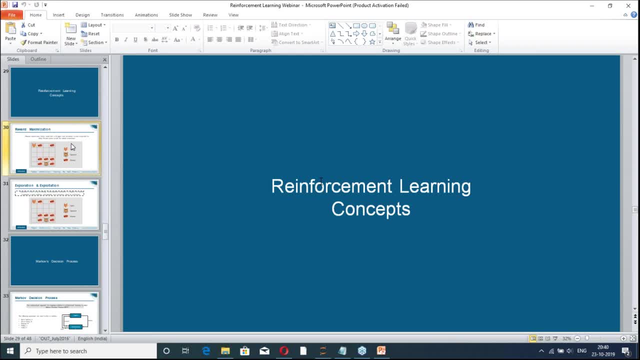 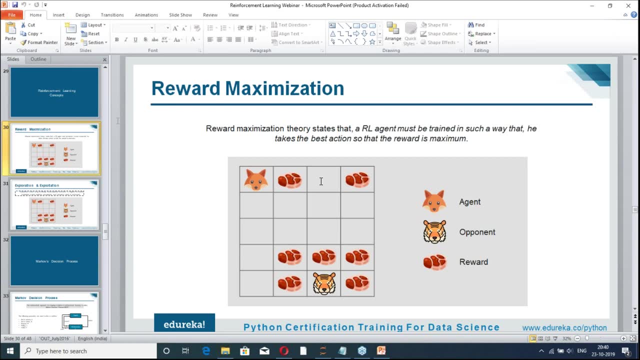 you got it okay, so let's go ahead. so one of the thing which we are going to do here, we want to, uh, have the to maximize the reward right. so there might be different. different paths are available. so what we want to do, we want to maximize the reward, so our agent should take such a path, or our agent. 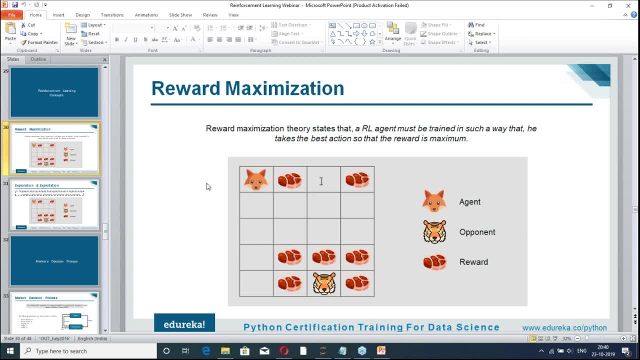 should take such action so that reward can be maximized. right? so this is one of the things- even it might happen- we can achieve. so how do we do the reward? so it is equivalent. let's say you are making your google. uh, let's say you want your google map to learn how to show the path, and all 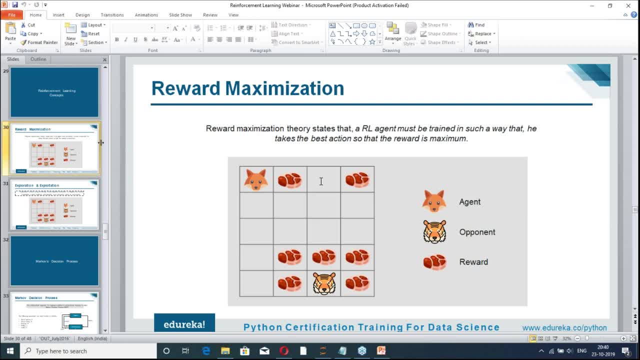 so here, even though you can write it completely explicitly, but you can do it using the reinforcement learning as well, where you attach- makes more reward whenever a user reach early to the destination, right. and whenever he reaches late to the destination, then less reward, right. so then what it will start is start finding automatically with the time being. 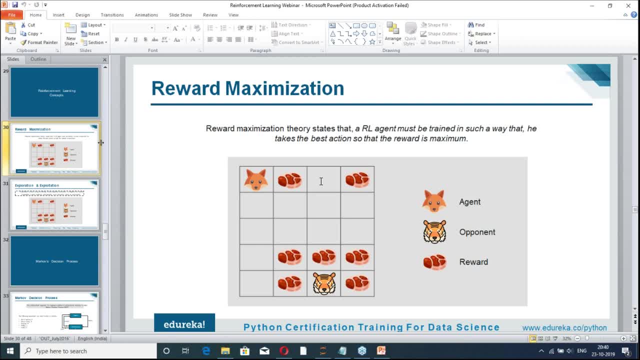 it will start finding that the path which gives takes less time right. so that is what reward maximization do, so you can bring out some particular kind of conditions, you can give some, uh, some kind of preferences for your game according by taking care of the reward, by adding. 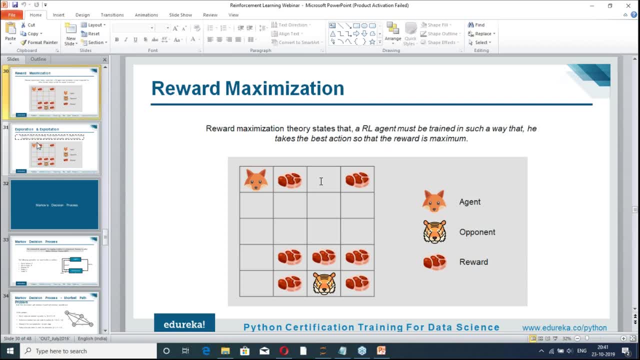 some kind of reward maximization maybe. let's say, you wanted to play some game, the lesser the time it takes to beat the opponent, better it is. then again you can do the reward maximization stuff there. then we have the exploration and exploitation scheme. so let me tell you it in a very simple way. 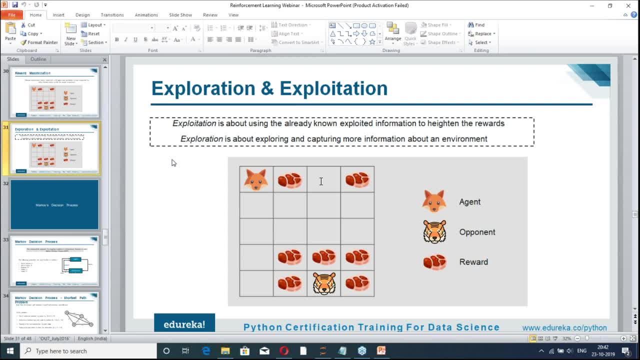 even though we can take a lot of time about it. exploration and exploitation is all about, uh, how to choose the particular action in a place, right? so currently, to keep it simple, let's say that it will take action randomly. right? so, first time it will choose some action randomly. next time, when it plays the same game, right then, it will take some. 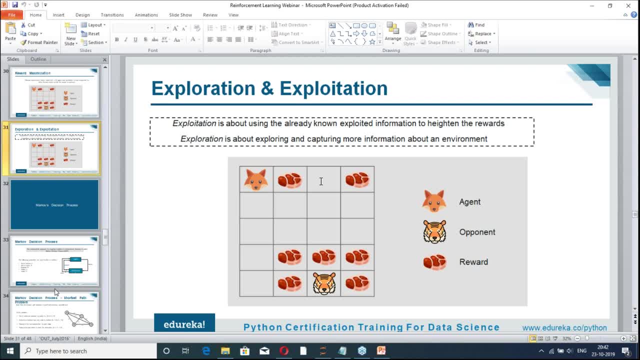 other action randomly. right, so it chooses action randomly. that, uh, what i can tell in the short form: exploration and exploitation. it is little bit more than that. but currently, to keep it simple, let's say there are lots of action available to it from which it can take, and it is taking it randomly. then we have the markup decision process on the 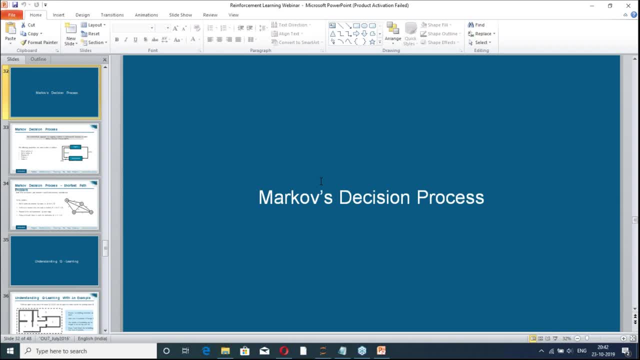 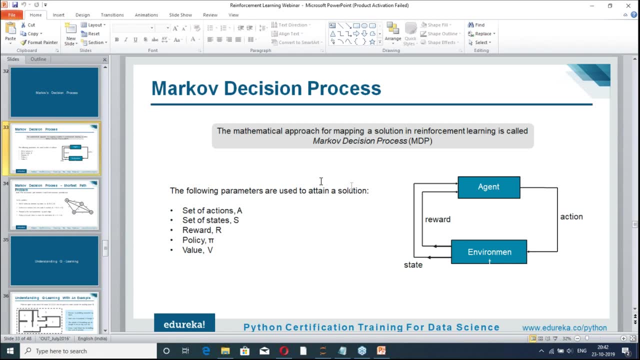 basis of which, uh, it takes the action. so let's talk about markup decision process. so mathematical approach for mapping a solution for reinforcement learning problem is called markup decision process, or whenever you need to apply reinforcement learning, the first thing which you guys need to do is to convert it into the markup decision process. 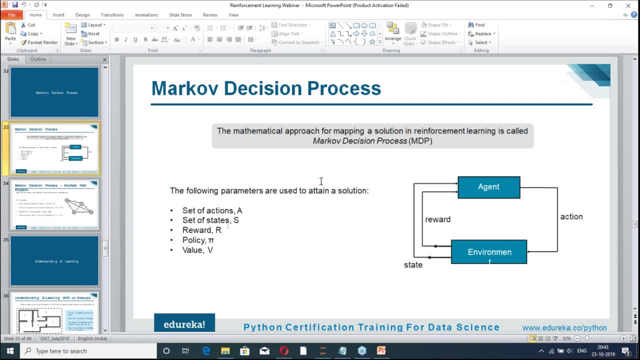 problem statement. so what things you need to define for defining your marker decision process? you need to define some set of the actions. a, you need to define some set of the states as basically, actually, what are the available action, the states, what are the possible state in which your system can be right, if we are talking about, let's say, chess right, so what? 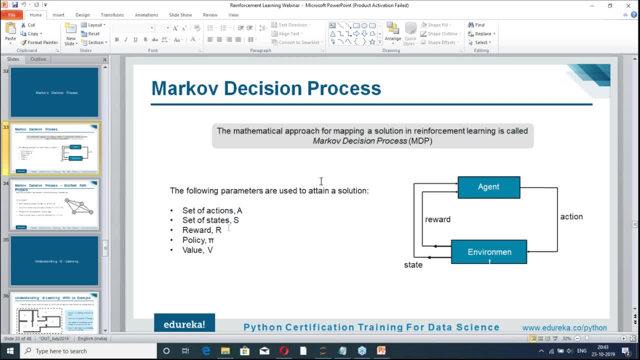 could be possible. state: your system can be right, innumerable, many- actually not innumerable, but still it can be many right. so like how the different players are put onto the environment. that is what we say about the states. right, then we have the reward. reward already, you guys. 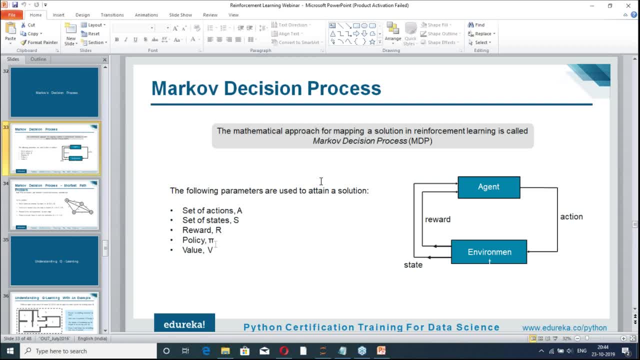 understood policy, pi and policy. we say that is basically our, that is mapping the and context or situation to the action, and the whole age is for the reinforcement. learning is to learn this policy only and then the value, which takes some part in deciding how good the policy is. 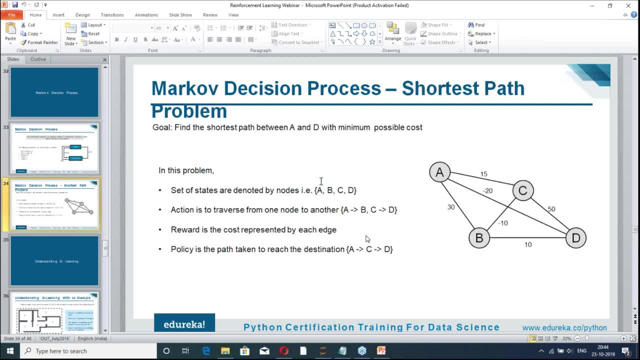 we will be coming to them, we will be discussing about them in a detail. let's say, this is our uh some graph and we want to find out the shortest path between the a and b right and these are the uh some values has been given. so what you need to define here, you need to define the set of states. 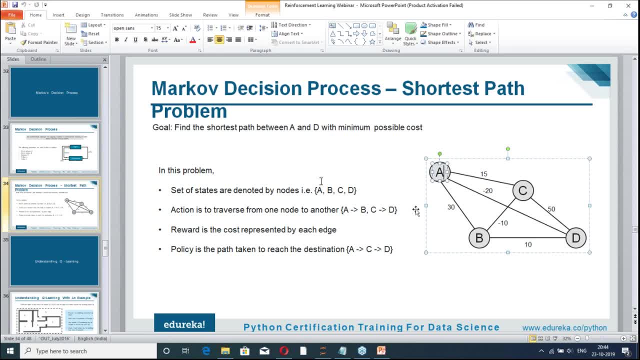 so whether we would be at state a when let's say: how do we define the state? that depends on us. let's say we say: if i'm at this particular place, i will say i'm in state a. if in this space, i will say state b, here state c, here, state d. so these are the possible states which we have into our system. 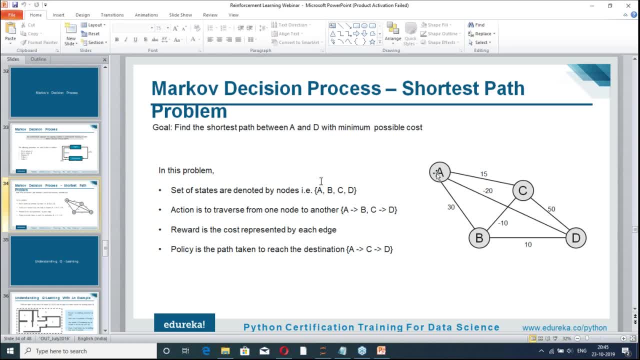 action. which kind of action i can take so when i'm at this state a. so what are the possible action i can take? i can take from a to c, i can take a to b or i can take a to d. right, so these are the three actions. 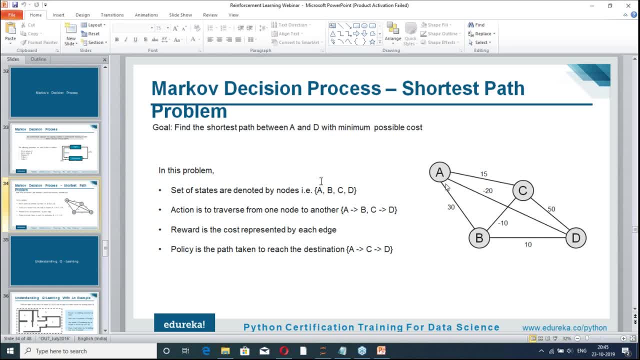 which are given here. then next thing is the report how much reward i take when i take some action. so if i'm taking from, if i'm going from a to c, the reward i will get is 15. if i'm taking action from a to b, i'm getting reward 30. if i'm taking action from a to d directly, then let's say i'm 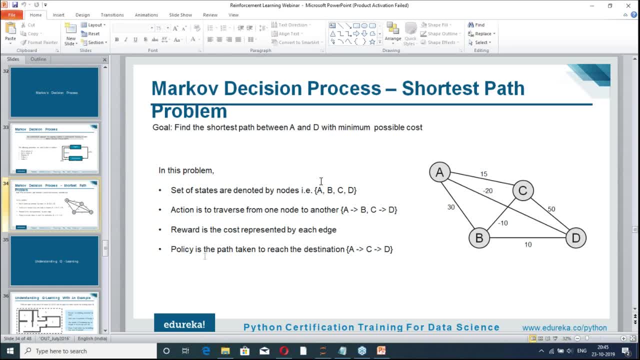 reward minus 20 right. and similarly we define the policies. so policy is basically how. so one of the pilot policy, if i'm at the state a is to take action c, so i reach to it as i reach here. then when i'm at the state c, i take action by reaching to d, directly, right even from the c. 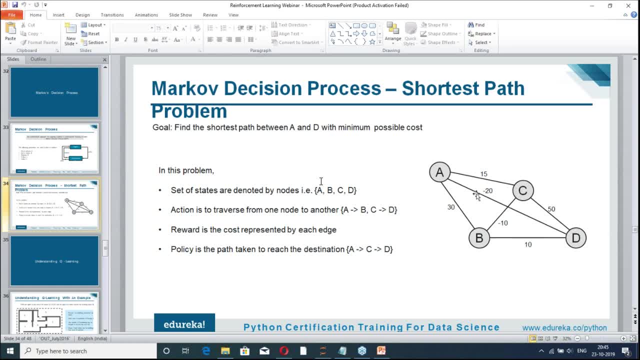 we can come to b, then we can go to d, but here how we are going to maximize reward. so what is the best policy? from a to c and then c to d, because that is where you are getting the maximum reward. you are getting 15 plus 50 right. that makes it 65.. if you go a to b, b to d, you get. 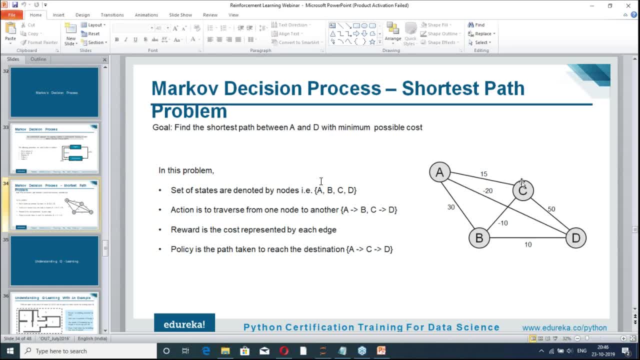 only 40 rewards: from a to d, directly minus 20.. a to b, then c to b and then further. then it becomes even more less right. so 15 minus 10, it becomes 5 plus 10, 15, you get on the 15 reward, so policy. 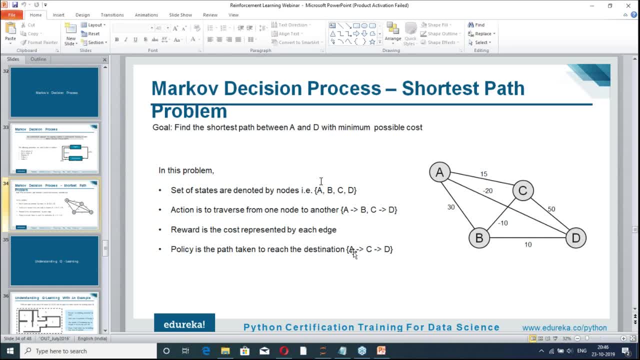 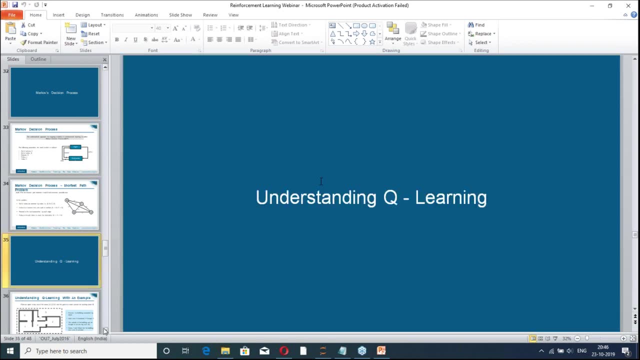 is all about what is the best action from a particular state. so here the policy. two policies are there. when i am stating, i will say, uh, action, go to reach c. when i am state c, the policy says reach to the d right. so that is our. now we are going to study. 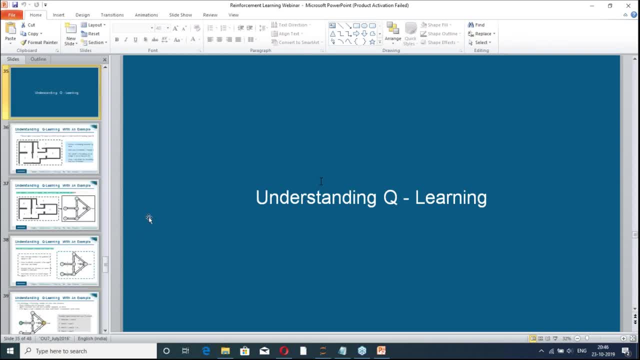 about the uh algorithm, using which we are going to implement our reinforcement learning, and the algorithm which we are going to study, one of the very famous algorithm which is being used, even though it it might look very simple algorithm, but it is very popular. it solves lot of problems in. 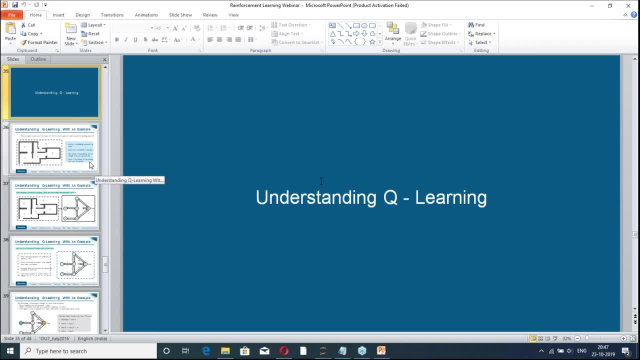 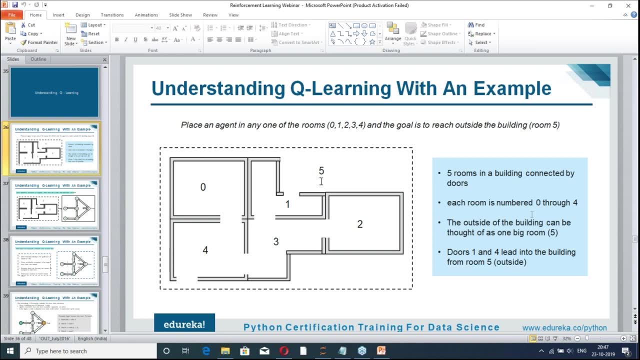 the real world? right, and sudhir was asking this question as well. right, and let's go to q learning, so understanding q learning with an example. so we, we are going to do this thing, also practically right. so we will see how to do it practically as well in a moment, and we will 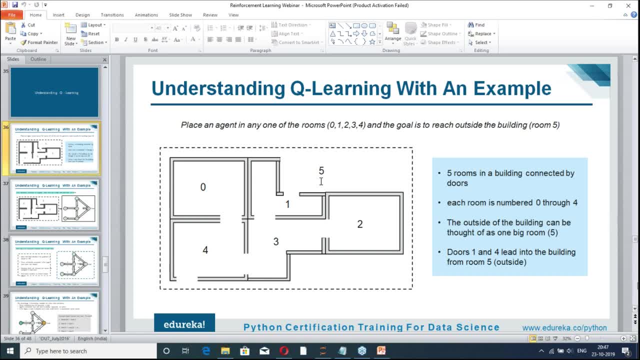 this is a problem statement, very simple problem statement we have taken and, even though the this is a very simple problem statement, but the things which you are going to do here, that stops which we are going to do here- you can use the same steps and there, and it will be a pretty cool, uh it. 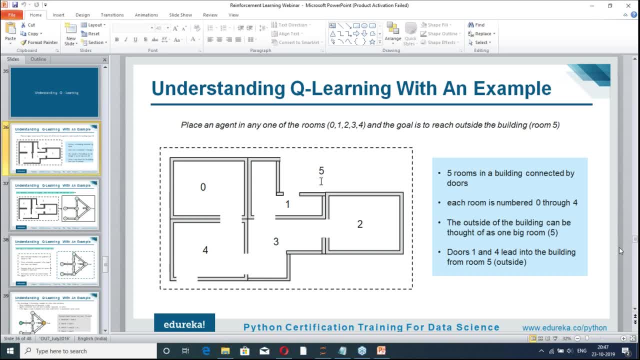 will be giving you very good results here. we will be seeing them right. so let's see, this problem statement which we are going to implement here is this thing. we will understand it with the example. so this is, let's say: uh, you have been kidnapped, suppose, and you have been in one of the room right and this: 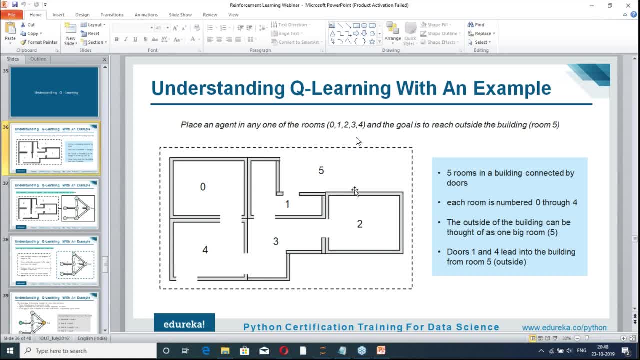 is, let's say, the bungalow in the bungalow in which you have been kidnapped, right and here, this is, let's say, number zero, this is room number four, this is one, this is three, this is two and this is room number five. right, and so room number five, we are calling as a outside of the building, right? so 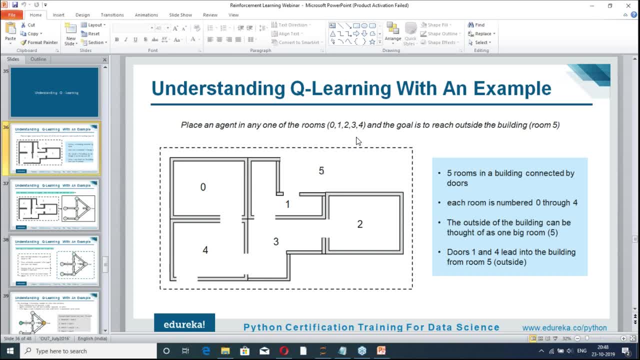 we are giving just any right. so we are giving it a surname for the outside and we are calling it as a room number five. Okay, and now. so each room is we have number that and we say this thing and we can see here: room number four. 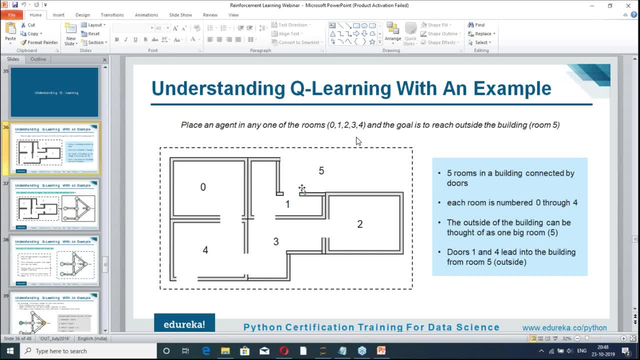 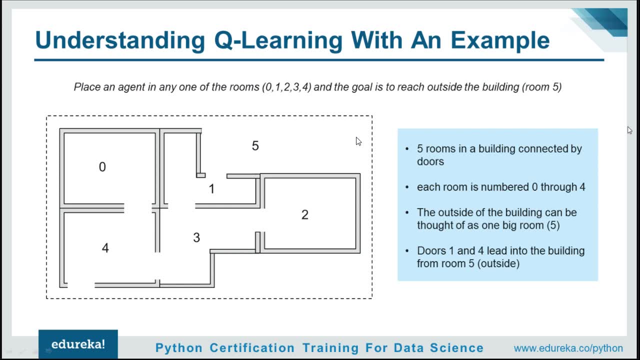 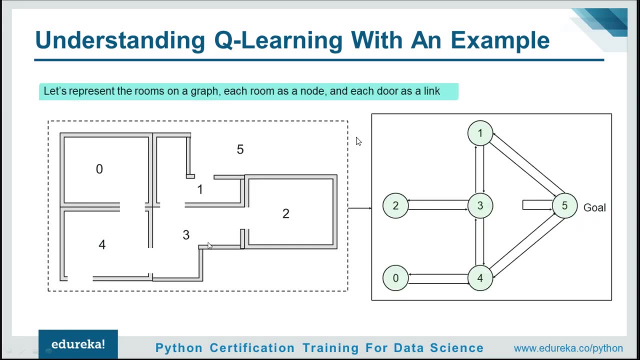 We can go from room number four outside world, and from room number one also, we can go to outside world. So only these two means are there from which we can go to the outside world. Right, so now, what we are going to do here? We are going to make it graph so that, using which we can make 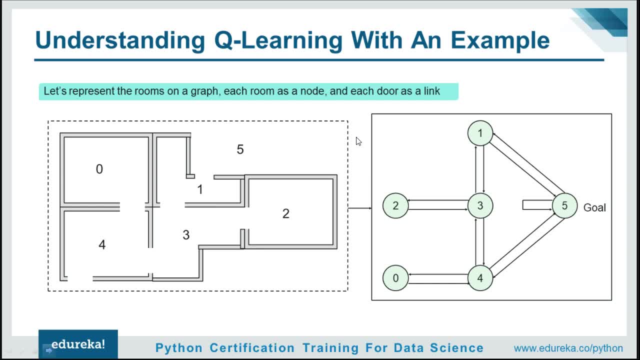 the state diagram, here, Right and here, if we see this particular graph, here we are attaching that, according to the existence of path, how the path is possible. That is what we are going to do. So here we are defining each of these room number. 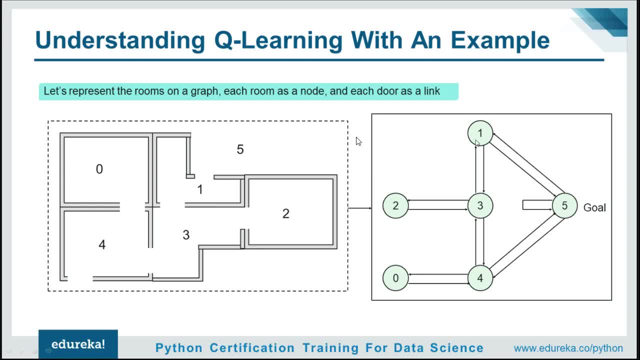 by the node of the graph. So here is 0. become 1 node. 1. become another node. to become another node, 3. become another node, 4, 5. right now We are joining them according to the path existing, so from 0 to 4. path is there, so from 0 to 4.. 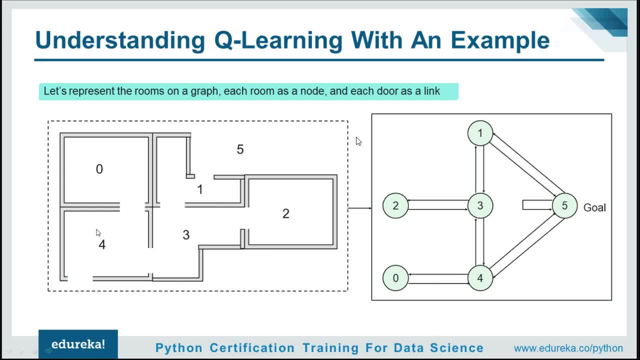 So there is only one path from the 0 right that is going to 4. so a person can go from 0 to 4 and he can come back as well. So that is why we have the pi direction path here. similarly, From 4 we can see person can go back to 0. 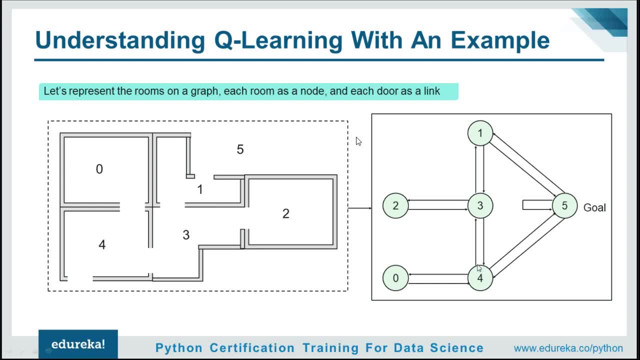 or maybe outside, or maybe to the 3. so that is right. from the 4 we can see it may be to 3, it may be to 5 or it might be to 0, right, So this way. similarly we do for the tool from the tool. 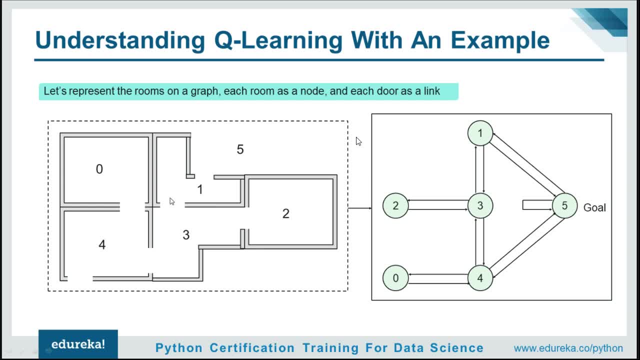 We can go on you to the room number 3, and from the room number 3 we can go to number 1 and 4 right, and from the room number 1 we can reach to the 5, and when we are at the 5, we can stay at the 5 as well. 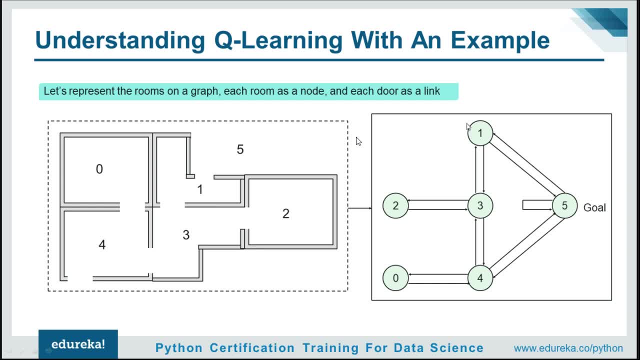 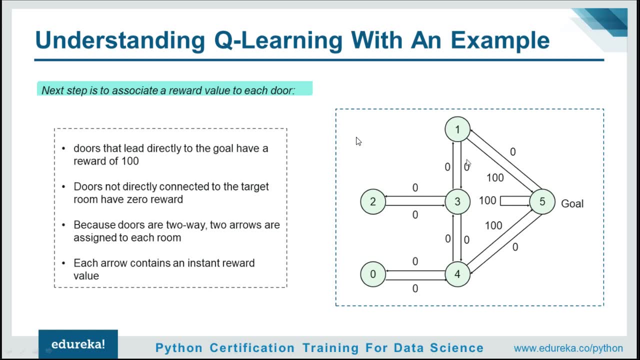 or we can come back to 4 or room number 1.. Now, what we are going to do, what is the next step? next step is to associate a reward value to each of these store. So basically, how we are going to associate here. Let's say, you are kidnapped. 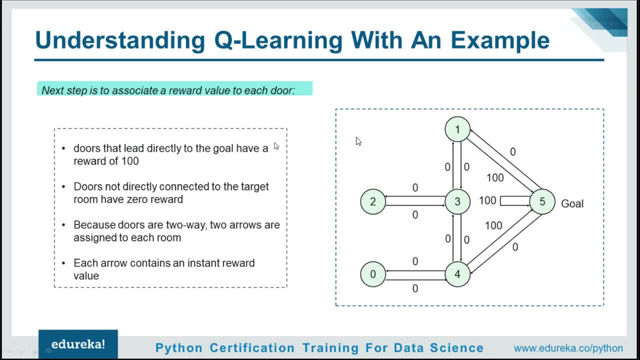 So what you really want to do is you want to go outside, right, That is room number 5, right, That is where you want to go. So, with each of the action, right? So what are the action? Here we have action is going from room number 2 to 3. 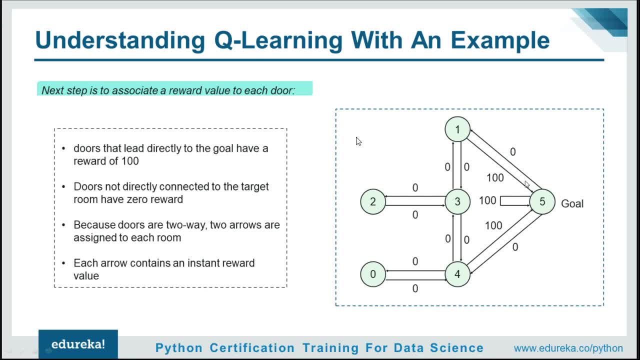 or maybe from room number 1 to 5 and so on, right? So these all are our action, right, and we need to add some reward for each of these action, right? So, whenever? so how do we want to give the rewards? So, whenever the whenever the action, it is like that: 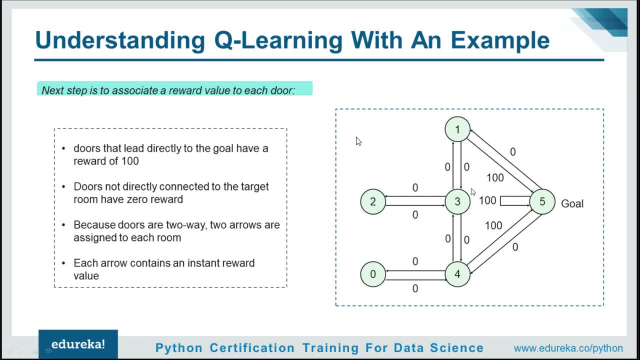 which is not taking you to the final state. Let's say we are giving hundred reward, right? So let's say we are at the state 2, right? So if we are at the state 2, and then if we go to room number 3, day. 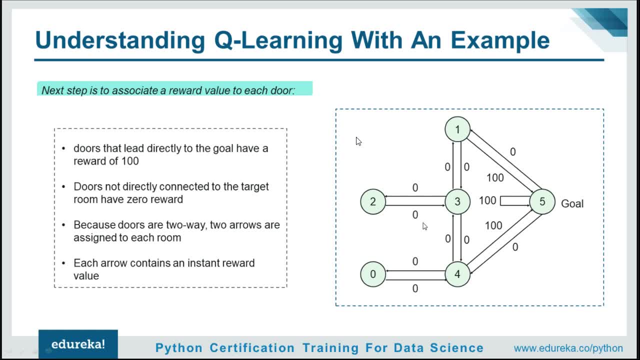 this is the only action we have, possible action. then the reward it is getting 0, because this is not outside room, but when we are at the room number 1 and it will go to outside, that is room number 5.. How much reward we are saying. 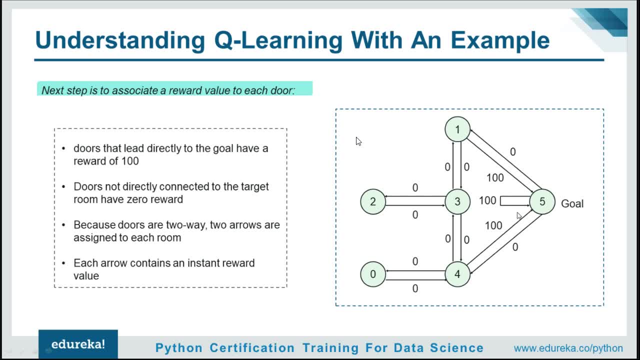 Let's say 100 reward. when at room number 4, reaching to outside, How much reward, we are giving it hundred reward. and when it is at the state 5, staying at the state 5 itself, then we say hundred reward, right, So this way we attach the reward here. 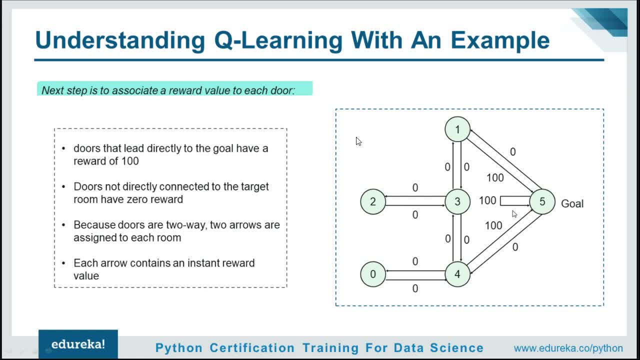 Okay now. so let's have the. let's discuss about the terminology here, different, different terminology which we are going to have here. So we have the initial state right. So let's say in which room number currently, or in which room number you are currently stored, right? 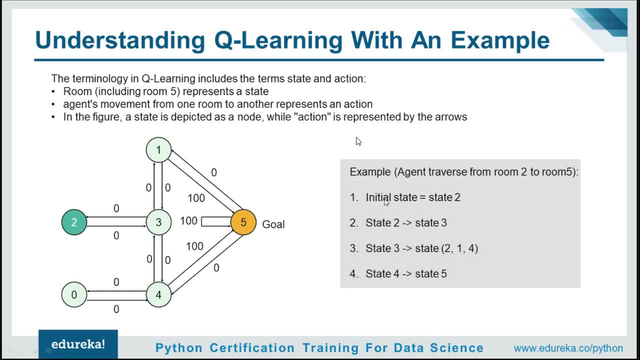 You are right. So that is we are calling it The initial state. So let's say initial state is room number 2.. Let's say you are at the room number 2 and that is what we are calling as a initial state, right? 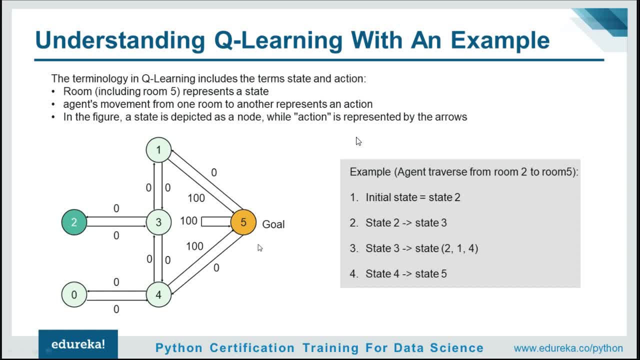 After that you take some action. Then you say action. How do we define the action? We say: from particular state 2 you can go to state 3.. So that is an action going from state 2 to the state 3, right. 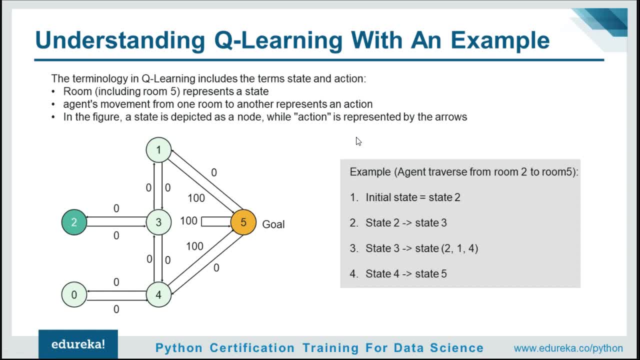 This is the possible activity you can do here. right, Then here we are writing. What is the possibility? that if a person is at the state 3, the possibility of the actions are to go for 214, right And from the state 4 here. 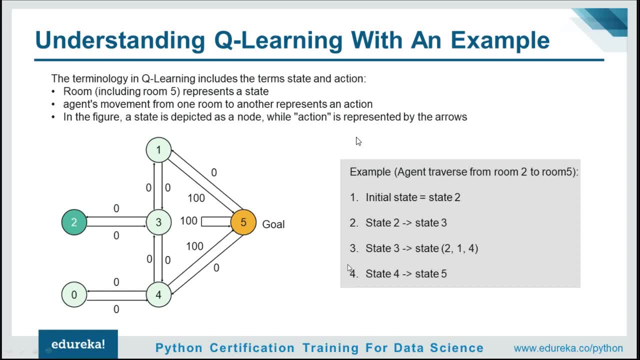 the action is showing, is is basically taking it to state number 5, right. So these are the some of the terminology we have. Now we are going to define first of all, the reward matrix: If a person takes an action, how much reward it should get, right? 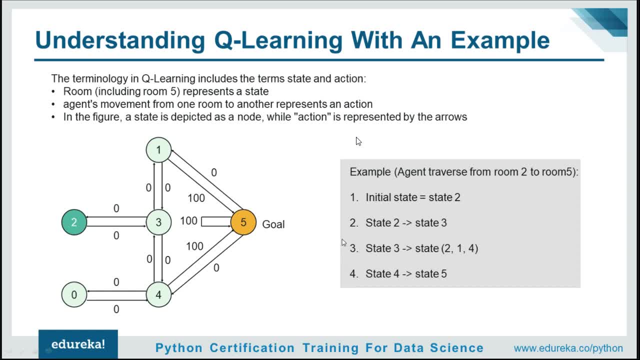 How much reward it should get, So that we already told how much more should get right And we say it should get positive reward 100 whenever it reaches to be outside, right outside of the room that is room number 5, and other places it is reaching somewhere. 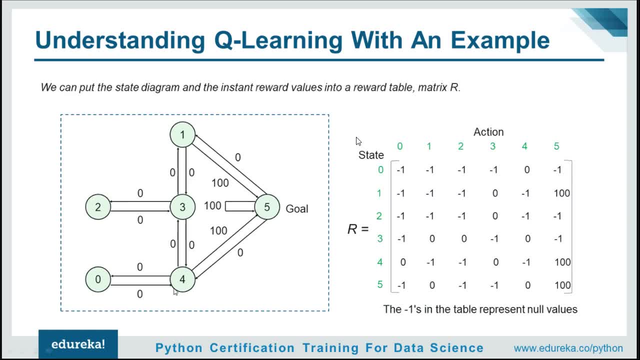 It should get the reward 0, right, So you can see here from the state 4 to state 5.. It is getting reward hundred, State 1 to 500, 5 to 500, right, So here we can see we are writing at these three places hundred. 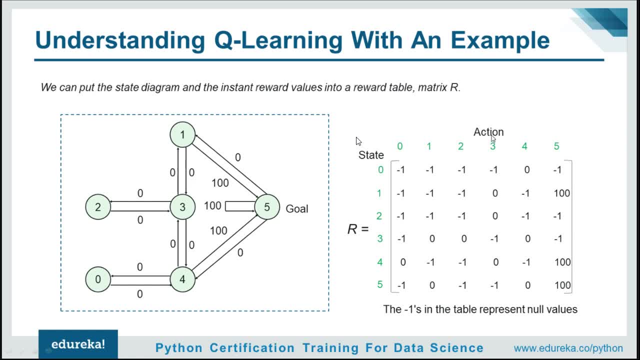 So basically these are same state. These are showing action. action is reaching to which particular room number right. So from 0, if you stay at 0, you will get minus 1 by a minus 1.. We are writing this specifically. We are writing reward as minus 1 where our action is not possible. 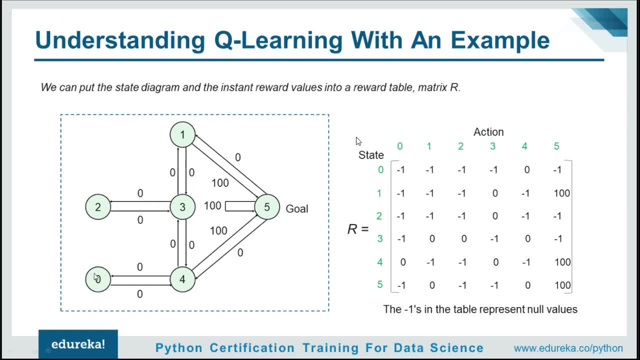 Let's say: right, So if you are in room number 0, you cannot reach to room number 5, right? So is that is right from 0 to 5, right? So here you look in the row number 0 and the column number 5 here. 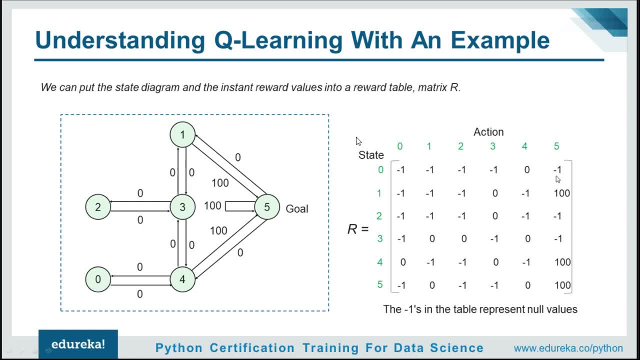 We are giving reward minus 1. that is on the basis of this matrix itself, We will see what are the possible action. So if you have to see what are the possible action, possible action are those only which are positive reward value, like whether it says non-negative active. 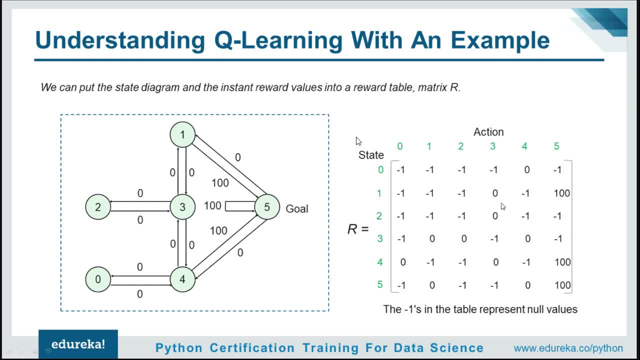 whether it says 0 or Greater than 0, 0 or right there about minus 1 is written, It means this is not the possible action. So using this reward Matrix, we can also know which action are possible and which actions are not possible. right, 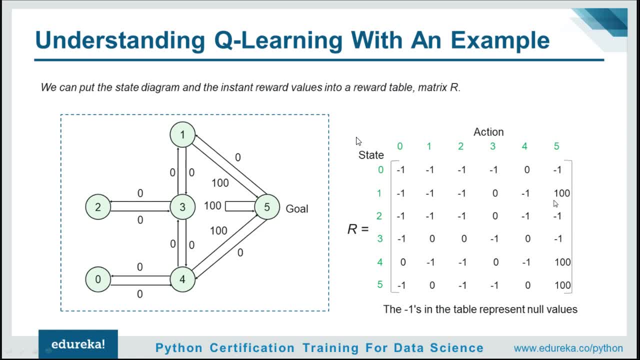 So let's do one more thing here itself. We will do by reading these things, We will implement this also, right, So that you guys, so we can do it practically as well at the same time, right? So let me just so that I can see if there is any query on YouTube. 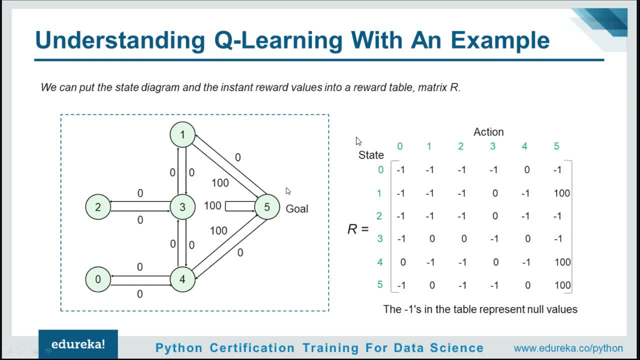 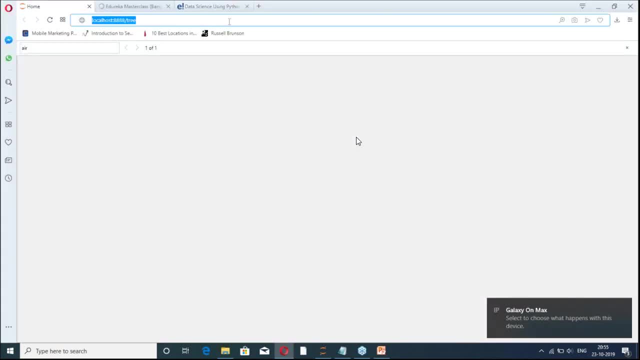 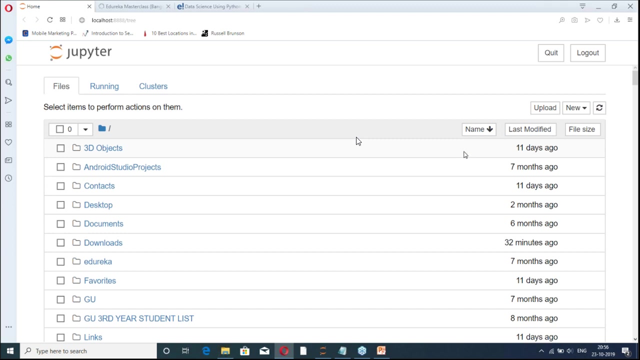 Okay, so let's, let's open the here. We open this thing. Let me see if it is still online or I shall. okay, This is still on my grade. So you open the Python 3 here notebook. It's not opening. 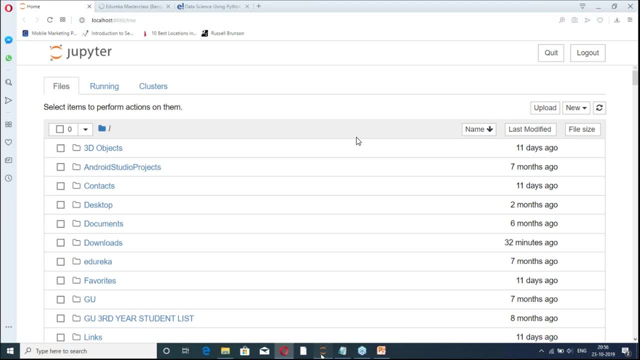 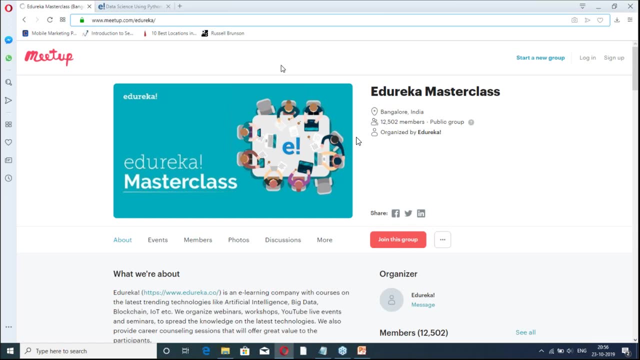 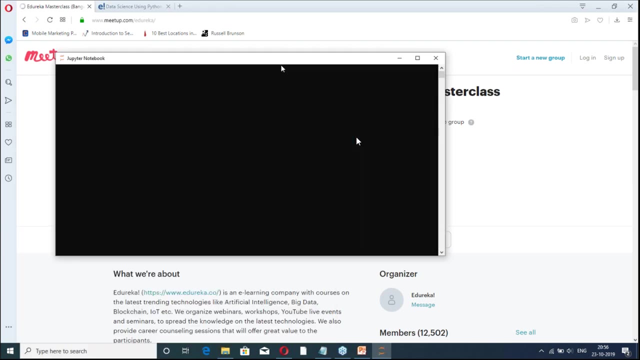 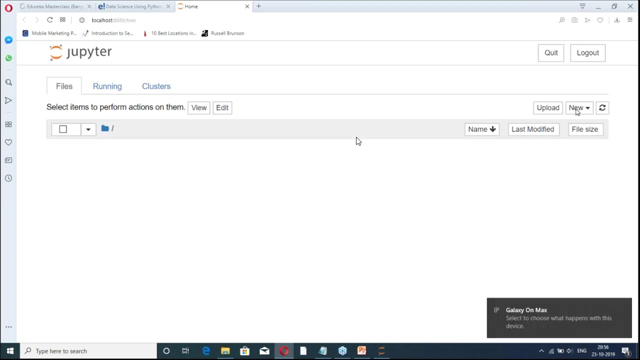 I think there's some issue with the server, So I will clone this server. actually, first of all, I will close this server, I will close this thing and again I will open the notebook server. So it is starting, the notebook and our notebook started. 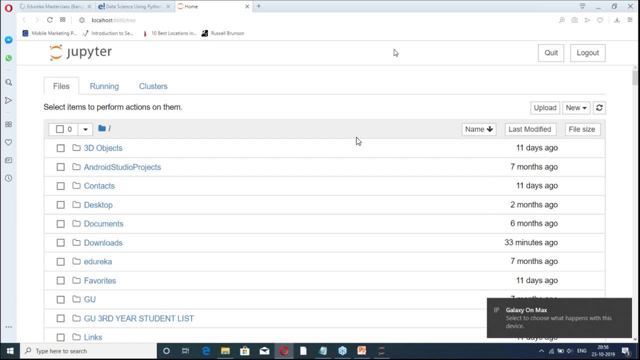 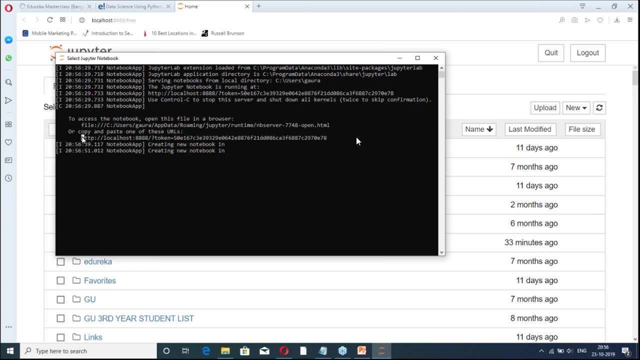 Now we can click on new Python 3.. Oops, seems like some issues with the notebooks. Okay, there is some issues, probably with this browser, So I will open this. Open this into using this particular link in some different browser. Right, So let me open the Chrome. 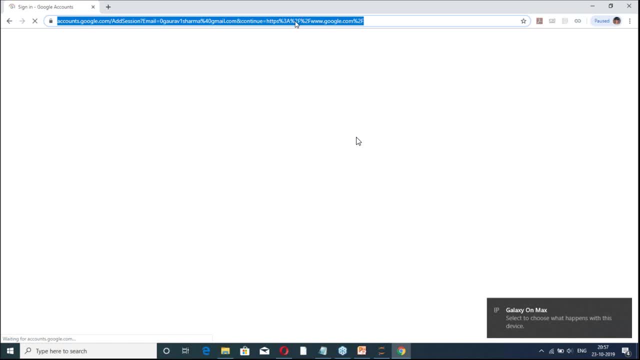 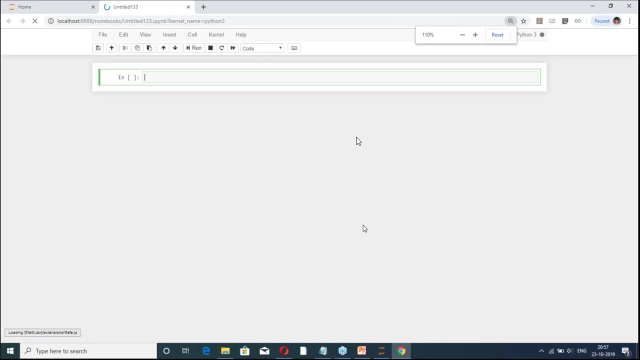 Let's see if we can open it in the Chrome. Yes, it is working fine here. So there is some issues with the Opera today. Actually, I was unable to open the your webinar as well using the Opera, So let me just increase the size little bit more so that you can see it properly. 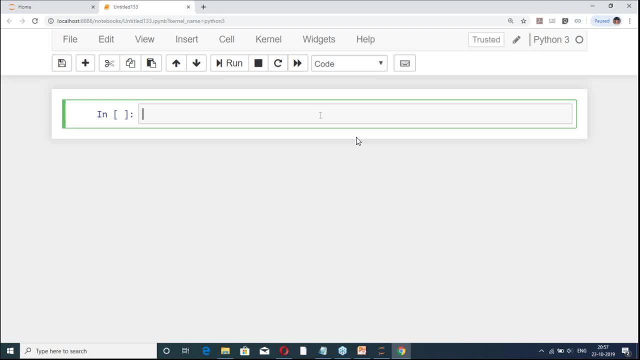 Yeah, that should be the enough size, Okay, so let's go discuss about it. So let's import first of all the library which is numpy as NP and let's write here: So we are going to make the matrix, So we call it NP dot matrix. 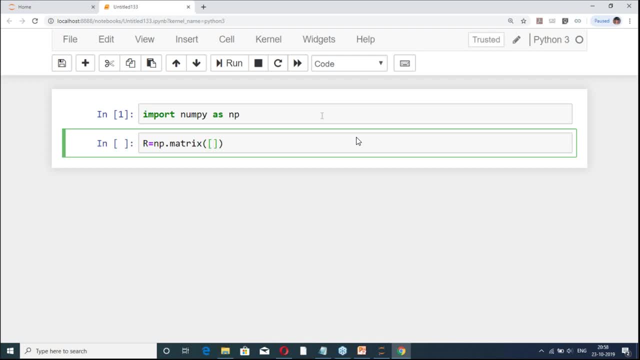 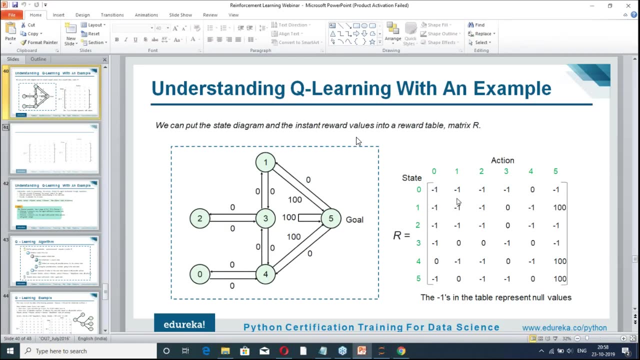 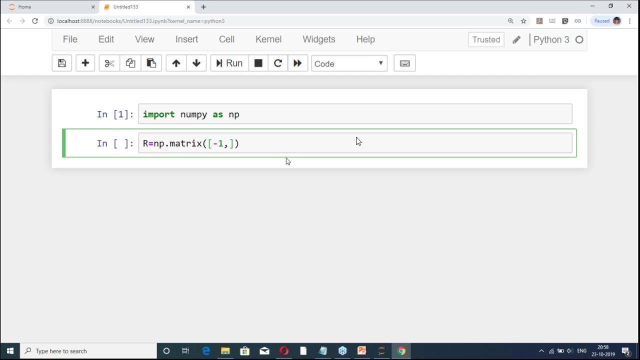 And here we guys are need to define this thing which we had here in our PPT, right? So this is four minus One, then zero minus one. here We have four minus one minus one. Let me just copy it so that we can quickly two, three, four minus one. 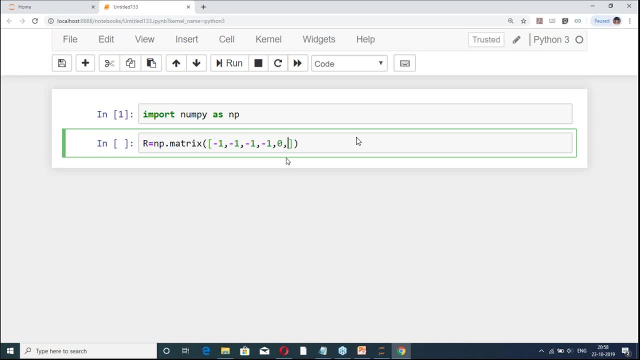 Then we have zero and we have again minus one. This is our first row, right? So how many values? we have one, two, three, four, five, six, right? That is the first row of our matrix. So let me make it two-dimension matrix. 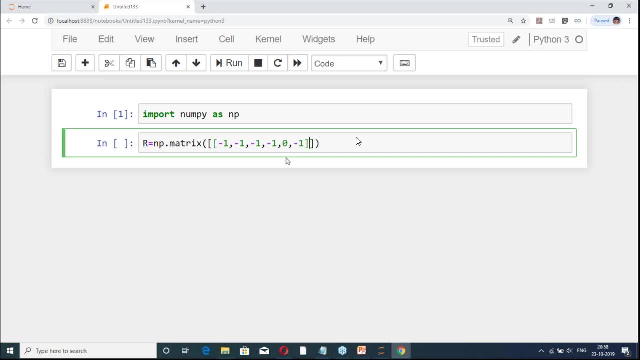 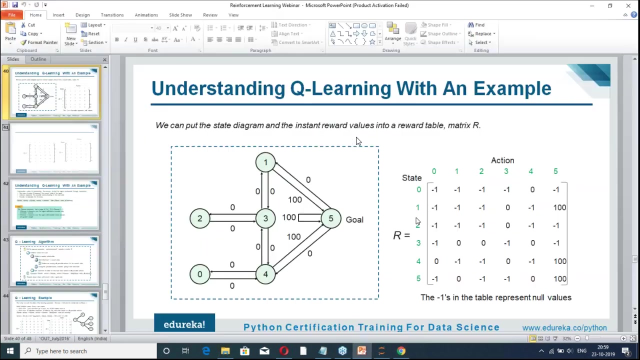 Then we have the second one and we see here: triple minus one, zero minus 100.. So we write the second row, minus two, three, triple minus one, Then we have the zero, the minus one we have, and then we had the hundred right. Then we have this third one: triple minus one, zero, double minus one. 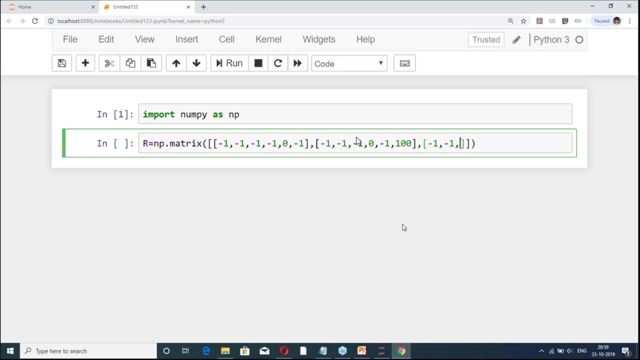 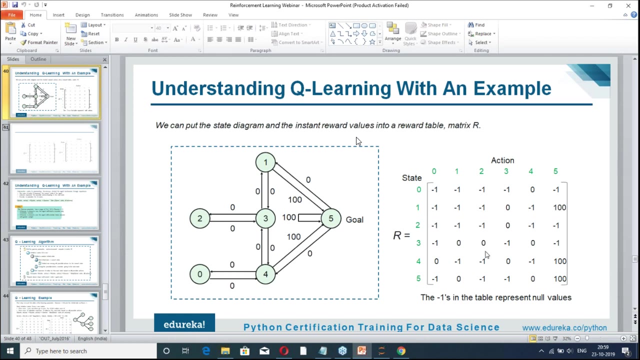 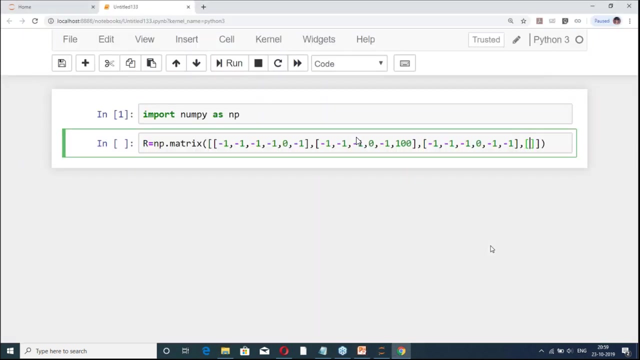 triple minus one. after that We had zero. and then we had double minus one, right, So we got top three: zero one, two done, Bam, This is. and here we have minus 100, and then minus 100 minus one, Right, So we have minus 100, and after that we had minus 100. 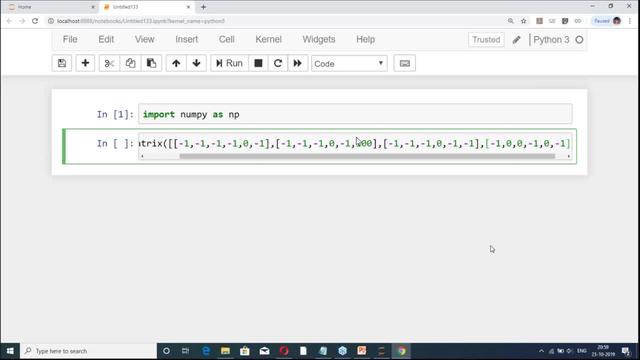 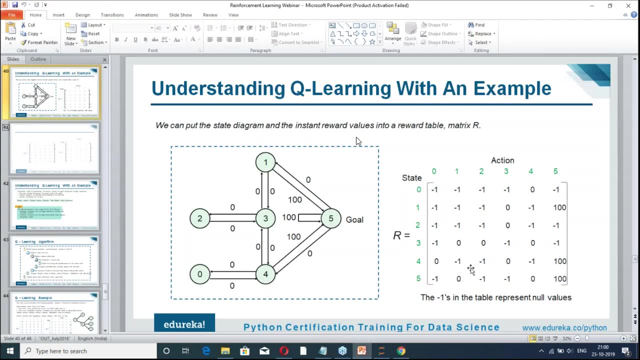 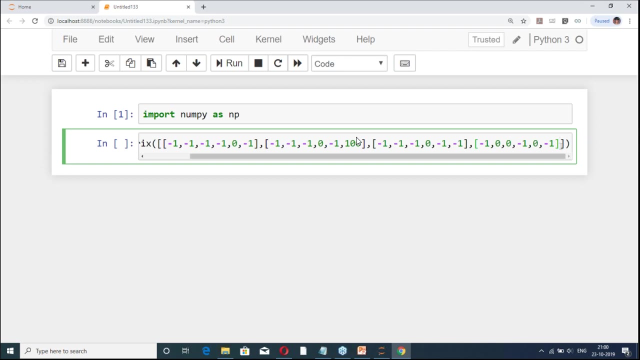 minus one. Right next here We have zero minus 11, 0 minus 100.. Right, So here we will add it next row and say here What zero Minus 11 it was, And then it was zero again, And then we had minus one, and then we had hundred. 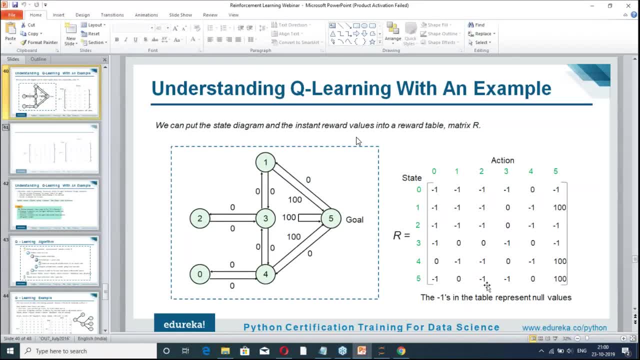 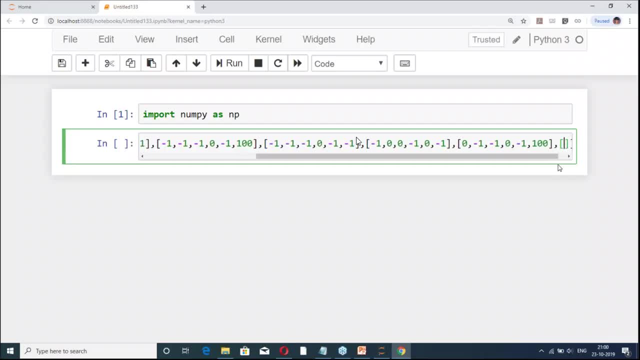 Right, So this was perfect. Then we have minus one, zero minus one, And then minus one zero hundred. So here we write: minus one, zero minus one, and then we have zero and then we have hundred. Is it correct? One, two, three, four, five, one. 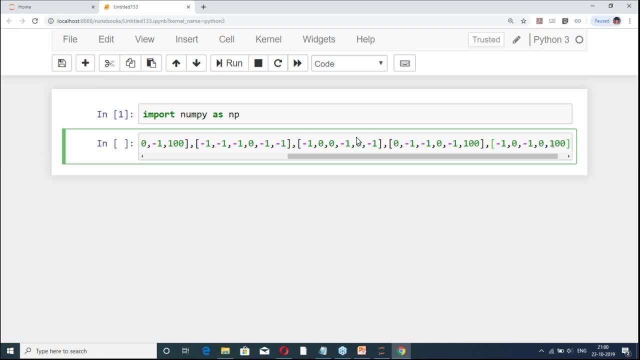 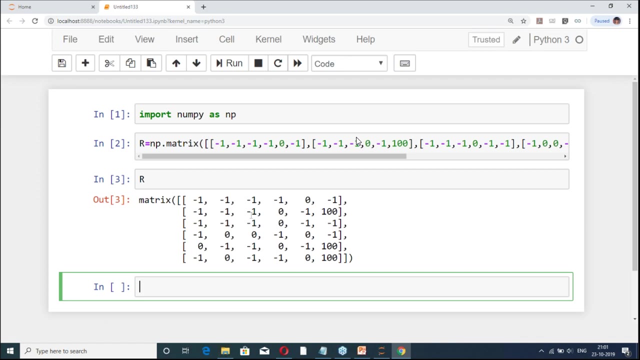 When we are missing here, We have double minus one. actually great. So we have created this matrix, are so we see? this is our reward matrix We have created, and wherever minus one is there, path is not existing. and wherever zero or hundred is there, path is existing with the reward value. 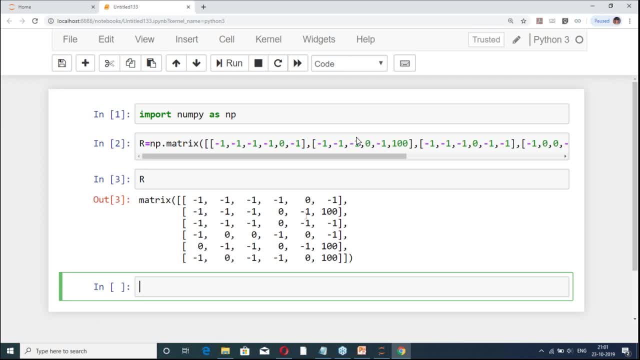 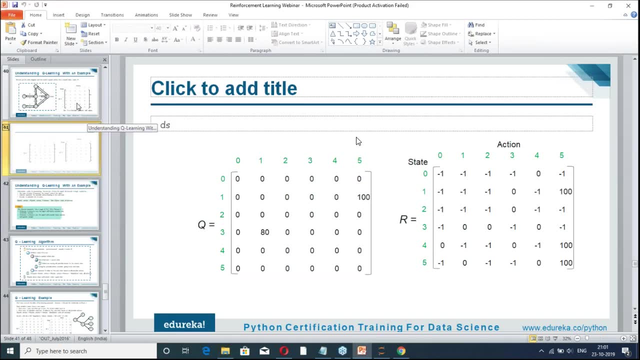 We are writing this thing Right. So after that we are going to have our Q matrix. as we will discuss about this Q matrix as well, How do we get this Q matrix Also? you see, but initially we are going to initialize Q matrix with the value of zero. 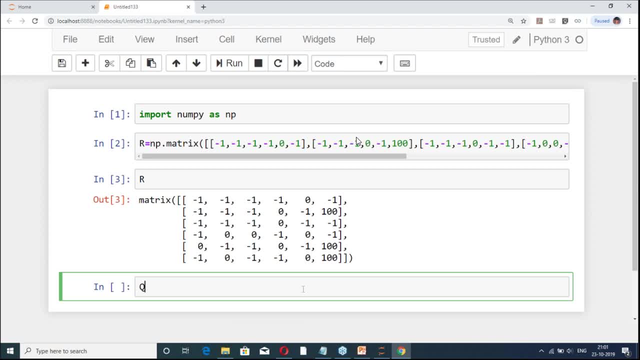 right, Because we do not know how much values need to be attached to each of the state, each of the action on the state, right. So that is why, initial, We are defining our Q matrix Right, So our Q matrix has a zero matrix. 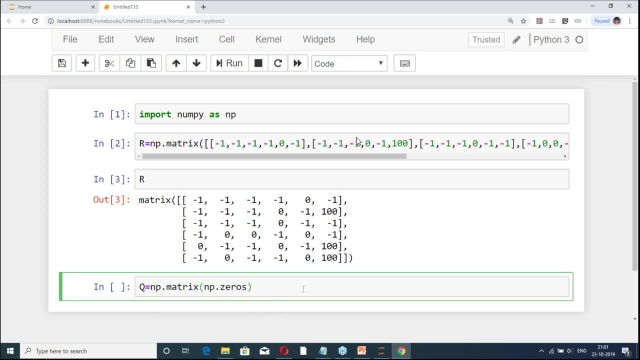 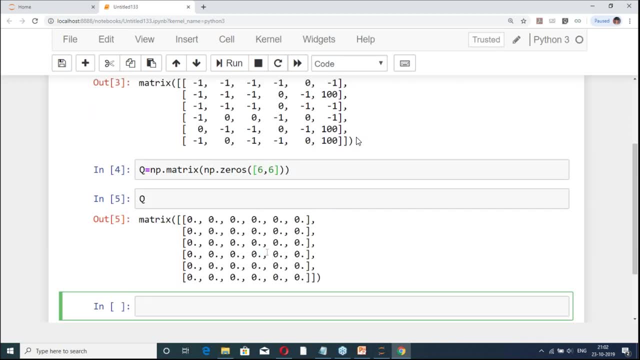 So we write here NP, dot zeros, and within this we write six comma, six right. So if we see Q matrix, so for each and every, on each and every state, for each and every action, we are initializing its value to be zero, right. 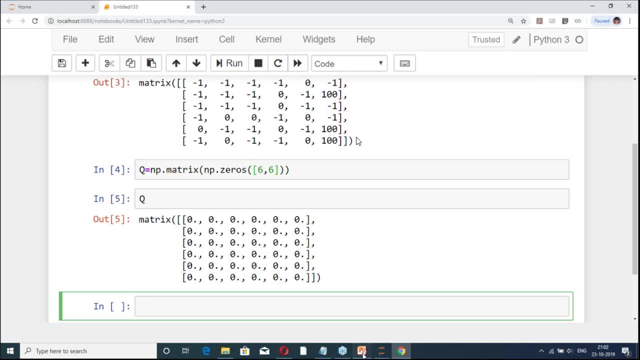 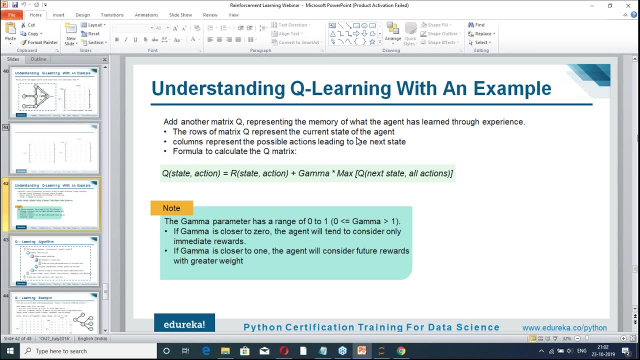 And how we are going to have this Q value. So our Q value depends on this particular formula. There is a whole, You know, there is a what we say, there is an whole proof for this formula, But currently let's start take this formula. 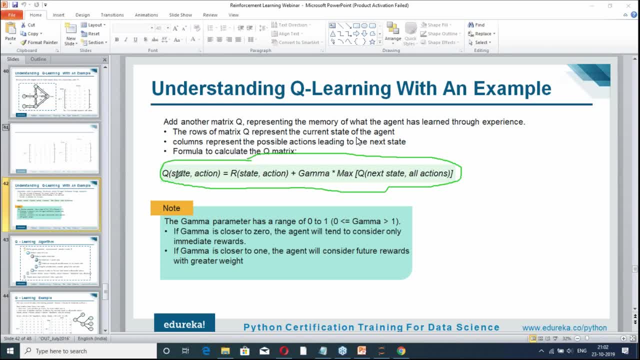 What this formula is. here We are saying that for Q, state action seems to be. Am I audible to you guys? Am I audible? Am I audible to my audible device? Am I audible? Some scan someone, right? Yes, Okay, great. 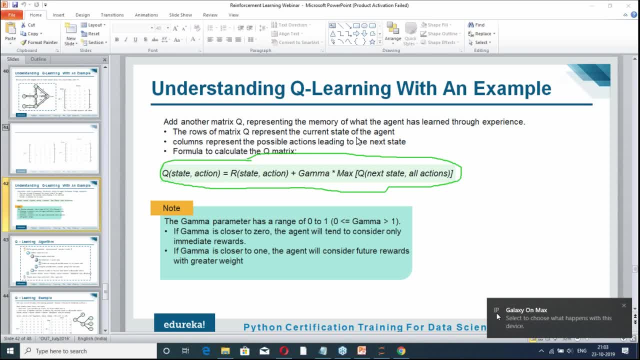 So go ahead, Okay. okay. so we were discussing about q, state action here. so we are saying that when you are at this particular state and taking this action, so what would be the value, right, how good action this is at this particular state? how we are going to find out? we will find it out on the basis of recursively. 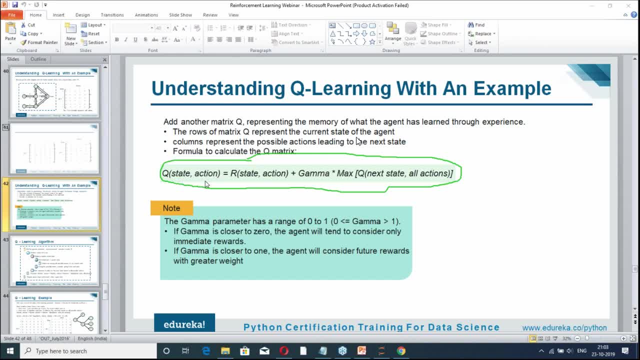 equation, we will see how recursively it is. so for finding this, a formula for this is that at this particular state, uh, for taking this action, how much reward it will get right? so how much reward it will get if it takes this action at this particular state means how the 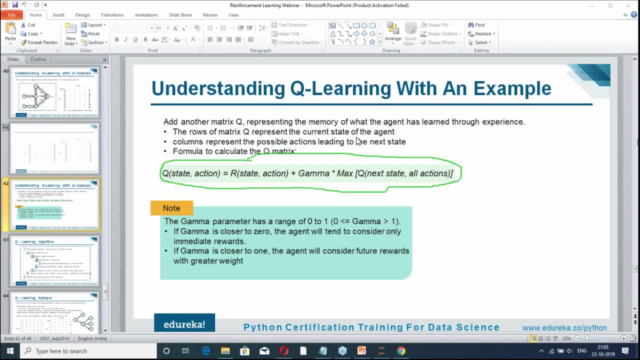 environment is behaving on it, plus gamma. here we are writing. so gamma is basically: we call it as a- uh, we call it as a decaying factor. why we are adding this decaying factor? because we want it to work at the earlier. so because of the decaying factor. let me just connect it. 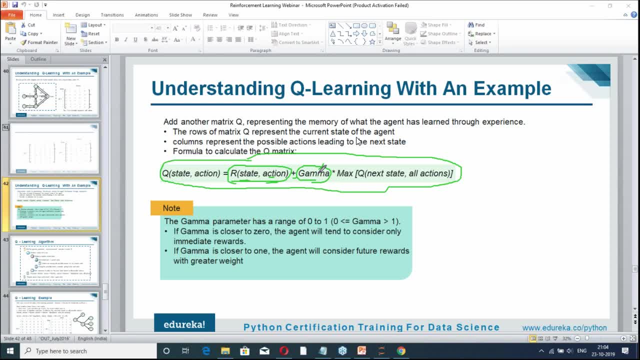 so we were discussing here about the gamma, which is decaying factor, and multiplying it with the decaying factor, actually, because we want it to reach to the uh, reach to the final reward. yes, right, so earlier it is, this will decay. gamma is basically less than one value, right, so it's so more later person reaches. 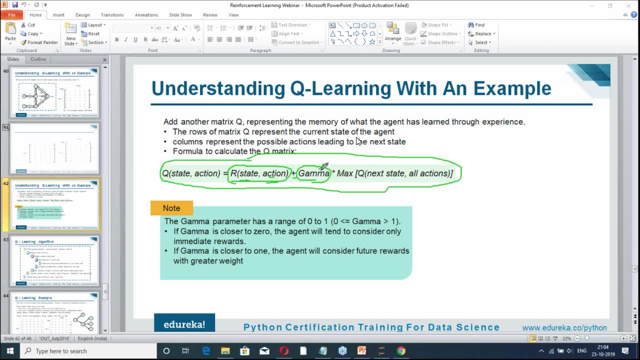 more value it would be reduced. so in formula is coming to maximum value we take. so we take because what action it takes, right? so we are saying it that whenever it takes some action after reaching, after reaching to the state for which it has taken action, then it looks, uh, what would be the best possible value it can take. 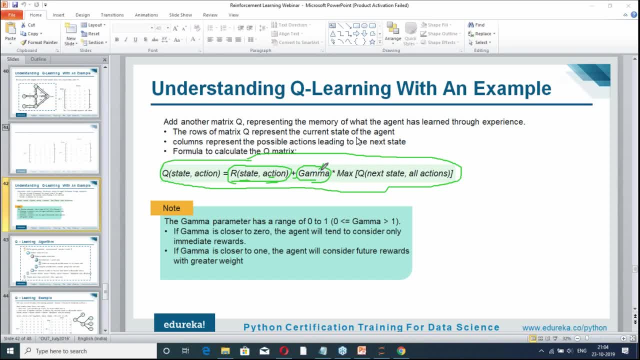 that is why we take from, which is the maximum value it will take from next state to all action. right, basically, we are saying here that currently it is in, in, in after taking this action. suppose if it takes all this action, then how much will that then? we? 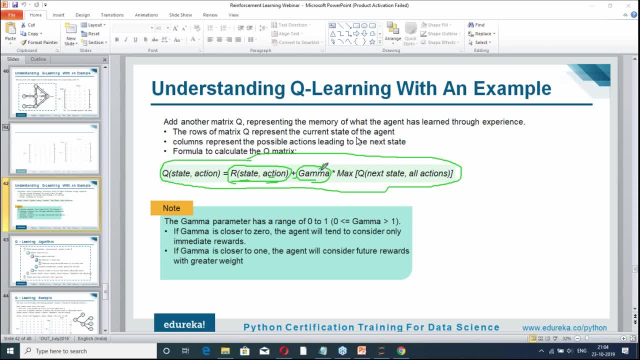 are copying it as maximum one. we will take it here, okay, as i told you, gamma value is in between of zero two, because it is a decaying factor. that is why we always keep it smaller than the one right. so let's see here: how does this q learning algorithm use it? what are the steps here we have? 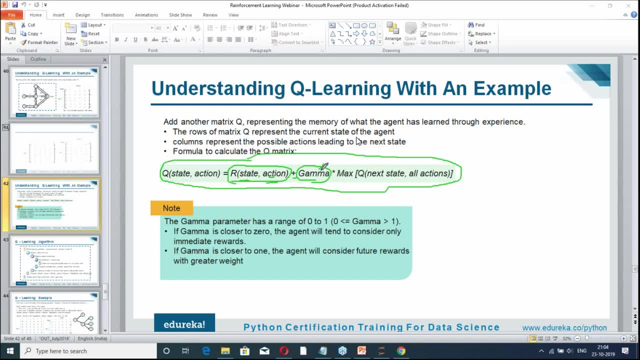 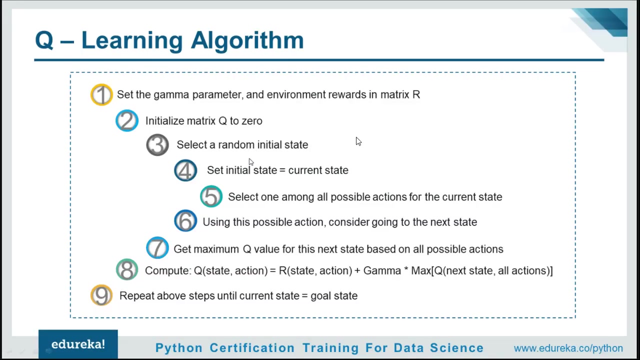 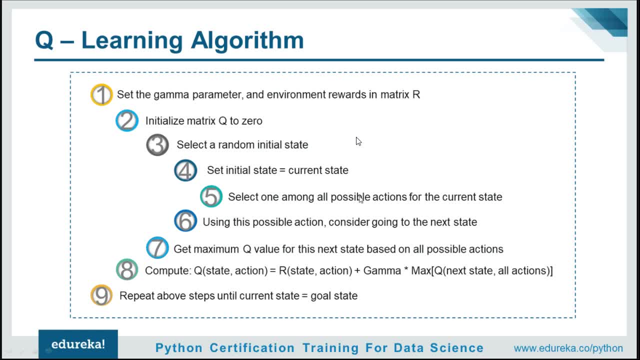 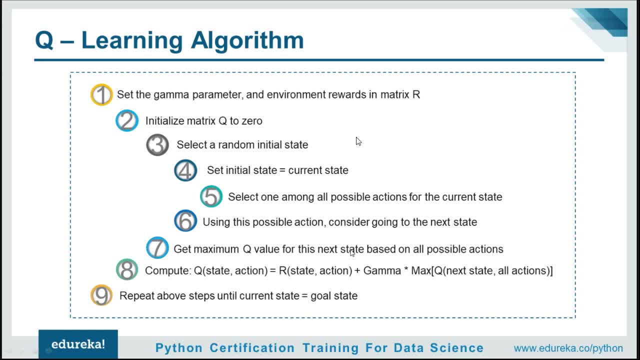 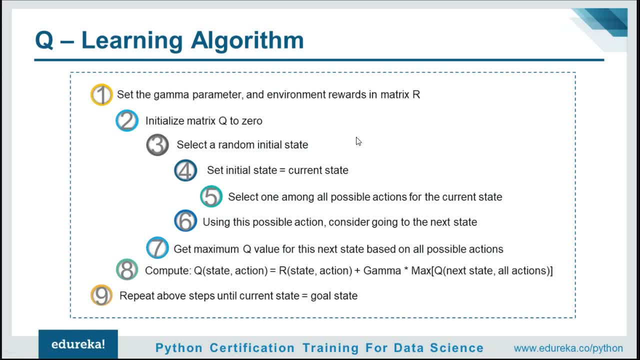 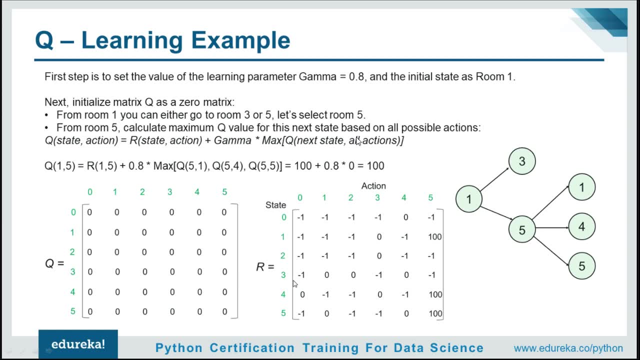 and it will find out new, new state, right? So here we are. we did this thing. Let's say initially: Q value. is this our value space, right? So let's say we want to start from the room number one, right? Let's say the initial state which we took was room number one. 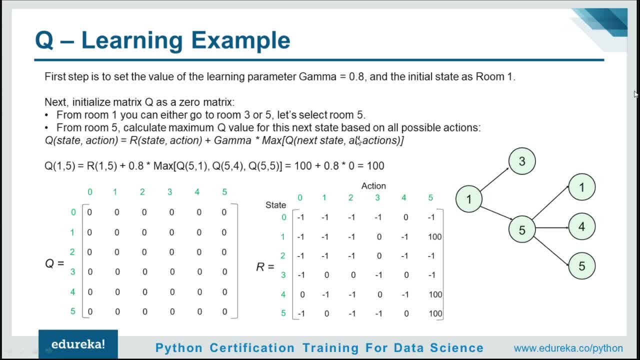 So you can go either to room number three or five. How does you know it? So if you are in the room number one, so you take care whether you can reach to the number three or you can reach to the room number five, right? 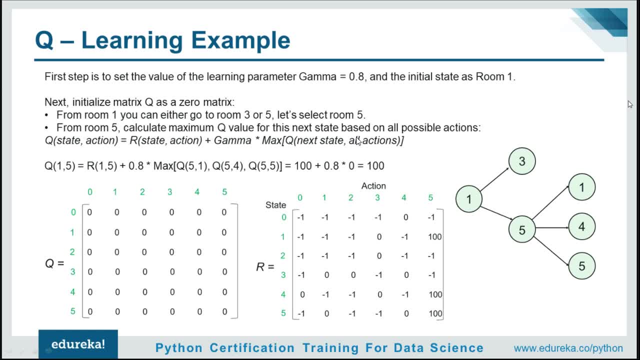 So these are all before. so how do you do it? You randomly select at the action because you don't know currently which action is past action. So currently you select randomly some action. next to the action which you selects here is, let's suppose it is room number five. 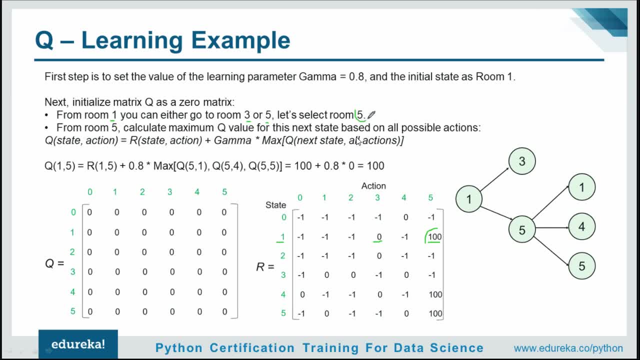 So from room number five. So once you reach room number five, so room number five is basically reaching here, right or here. So how much reward you are getting when you are taking action from one to room number five hundred report, right. So that is here. 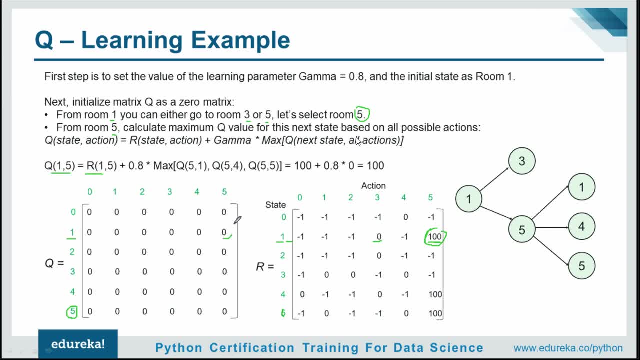 We are writing that Q 1, 5.. So we are going to update this value. We are going to calculate it that Q 1: 5 is equal to R 1: 5.. That is how much reward it is getting, hundred plus. find a point. 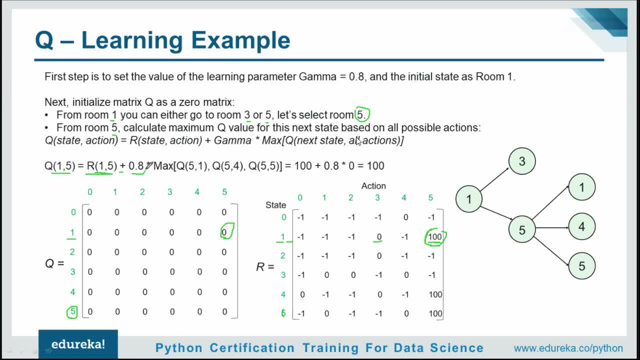 It is of. we need to decide this gamma factor which we are saying it's appointed, So you get it pointed into maximum Value for Q 1.. So we will see what is the maximum value here. right, That is in reality. you will be seeing which are the possible action. 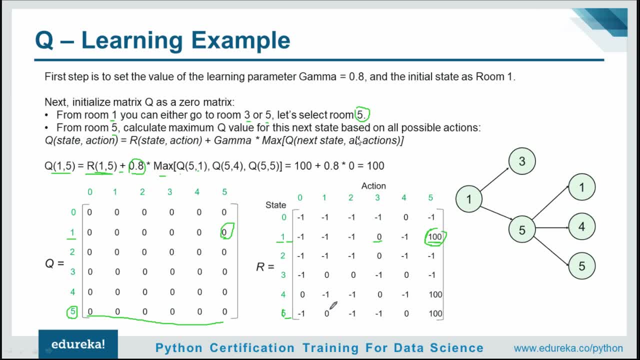 So from fifth state, the possible, whether you go to take one or you go to room number four or you go to five. That is why we are writing here: Look for maximum: Q 5 1. Q 5, 4. Q 5, 5. 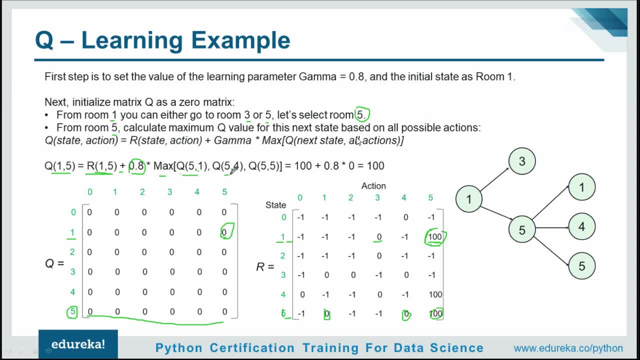 or you can look directly into this row itself, right, So the maximum value is 0 only. So it would be fine 0. so you see what become Q 1, 5 is hundred plus point taken to 0, which will give you hundred only. 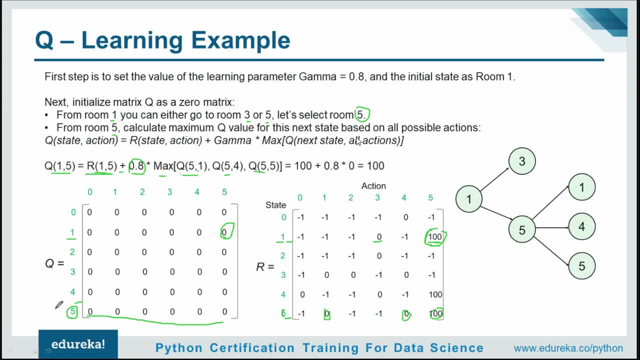 So we will update this particular value as a hundred value ready. So this is the audition we get Right. so here you can see it has been updated to hundred, right. and then again you take from further. you take, let's say, this room number three, right. 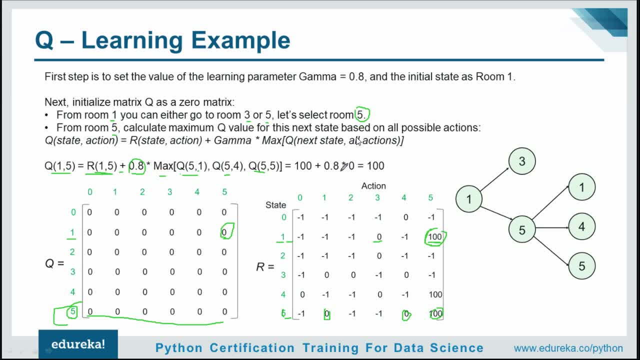 Let's say this time you are choosing the room number three, actually Right, and from room number three you can go either to room number one, two or four, right, So you go to here. from room number three you go to one To right, so you selecting some room here. 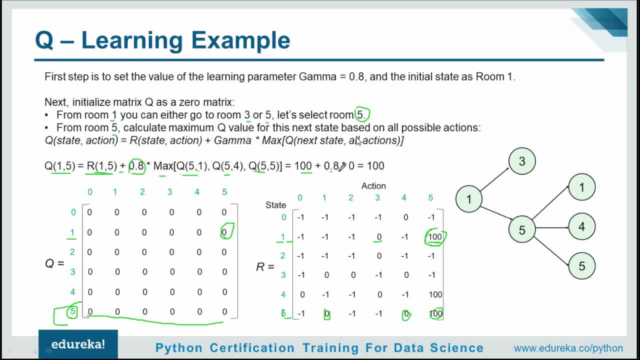 Friendly, stay number one. So you are selecting this number one You are getting about is see number one- What is the maximum right? So you can do this row. I think it is under right. So what is the formula It becomes is reward 3 to 1 plus 0.8 to value of Q and Q, and this is maximum. 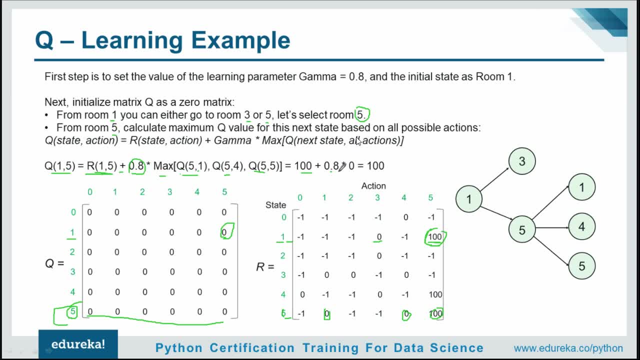 It is coming as hundred, So we get 0 is rewarded to get here here Plus 0.8 into hundred, which becomes a right. So this way you updated value And so that is 3: 1 right. So you keep updating this value and this value ablation. 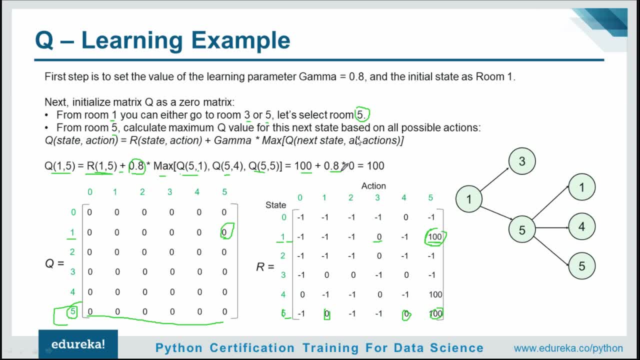 Then you will be teaching to some final state. So let's see, Let's do this thing and see where we change Right. So we created the queue. So now what we need to have, We need to decide our gamma value. So let's say, gamma value is our 0.8.. 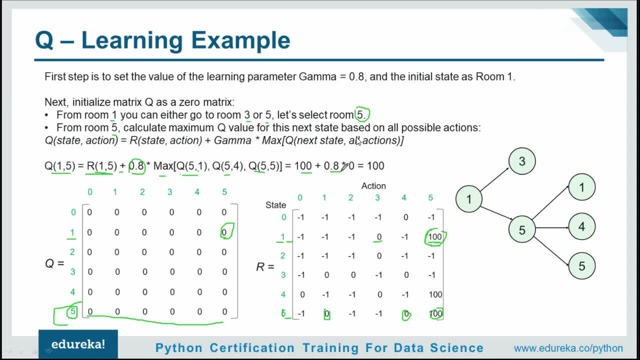 Right, We need to divide the size initial state, Let's say our initial. It is one We can choose any randomly, which will be doing earlier, Which will be doing random, but currently, for keeping something to show few things, We are taking it as a state, as one. 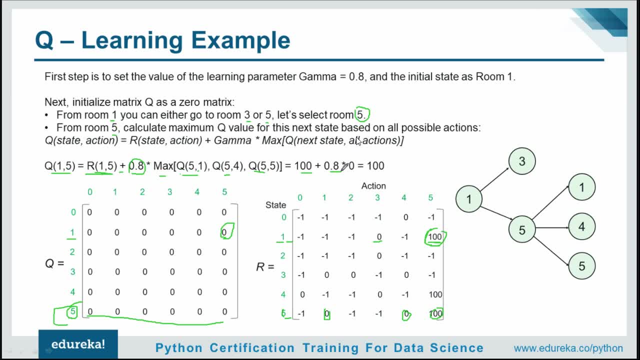 Right, Then, what we need to do? We need to take sections. for that, We need to find out which are available. So for that we will define one dysfunction which is available: action. And here we are defining this state, And here we are writing. 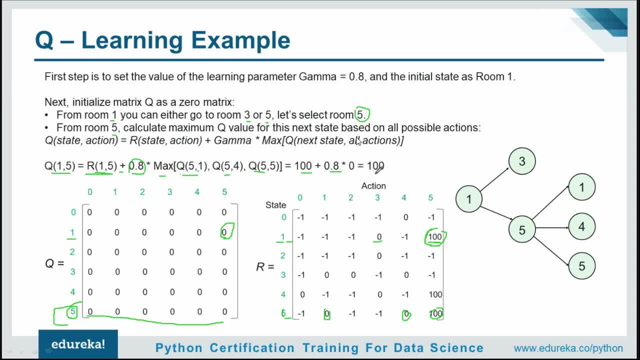 It's a row right, So we'll be taking first of all row, will be taking here row Right And here And we will take. so let's say, if I want to check from this, let's say if the state one, then I will be taking this row. 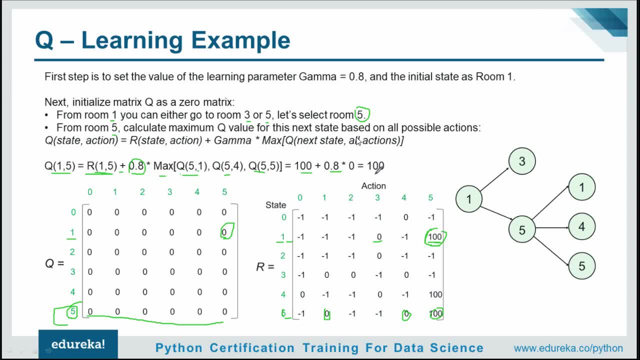 so that I can find out whether it is objection, I can take right. where it is for non-negative value, I can take the action there Right. So that is what we are selecting here. current state row. We got our state right. So that row we get. 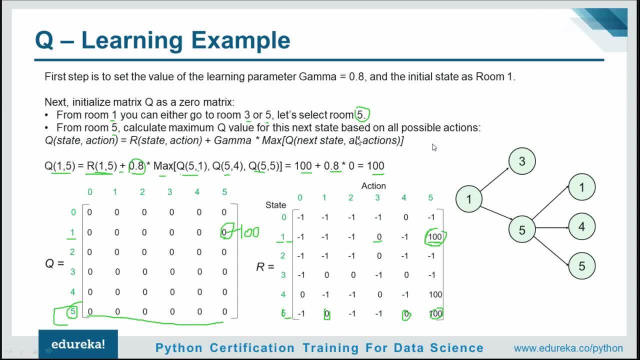 After that, we can then take the available action. So how do we take the available action? We say: all the action there and we got there. Our current state row is greater, equal to zero, right, Non-negative value, and then we are writing here: one. 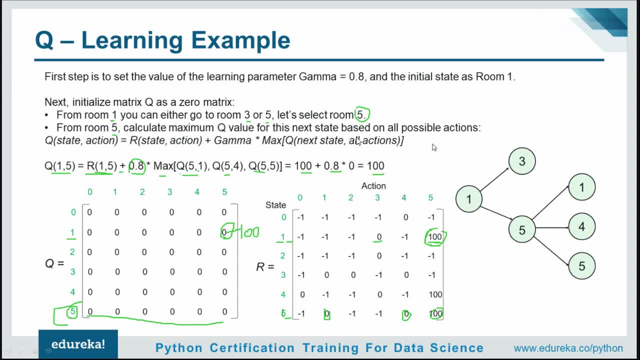 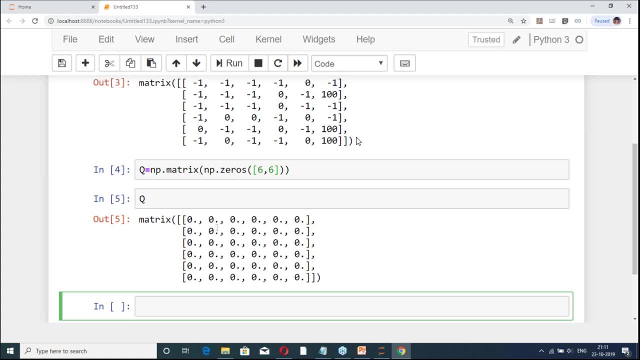 I will be showing why we are writing this one actually, and from this we will be done this AV act right. So these actions will be returning here. So let me Say, if I write it here and if I do this thing, so let me write here, as in the 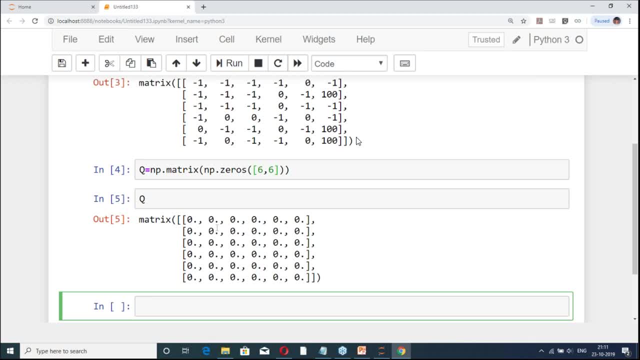 Right. So if I print them then you can see it has a particular row right, Which is our row number one, showing where it is right, And after that We write here that We write here in between this, Yeah, and we take this thing right. 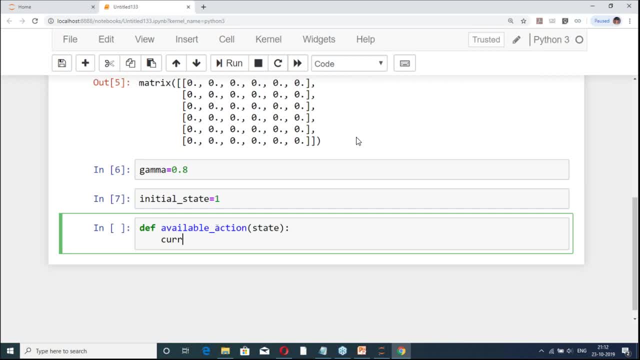 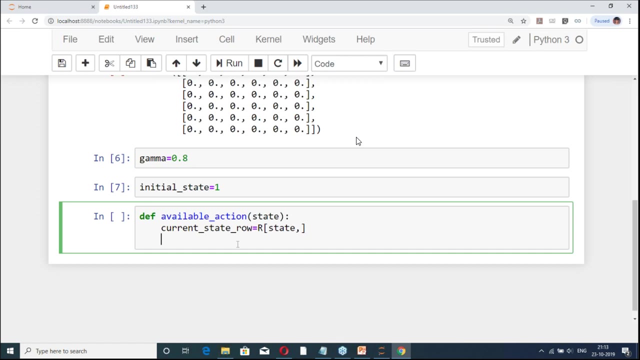 So what does it return us? So we this will be returning us. there. The value is greater than or equal to 0, right. So it is saying the it is your only because this become a matrix. it is taking- So they think you're a throw- only for both of these value. 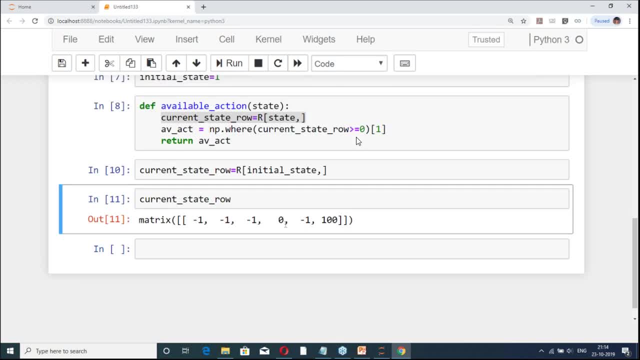 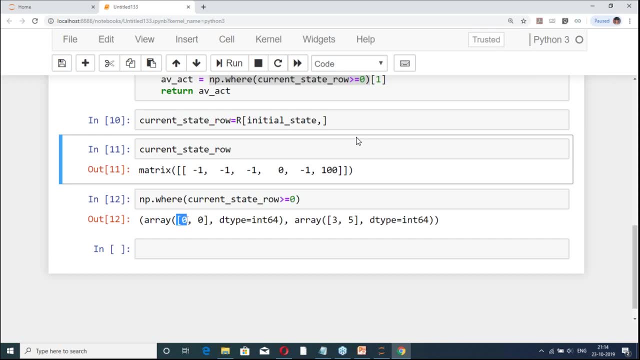 It is returning column number is 3 and 5, right. This is for number 3, column Number 5. So, in which we are interested in these column, only These are available action. If I write it, you can see this is 3, 5, right. 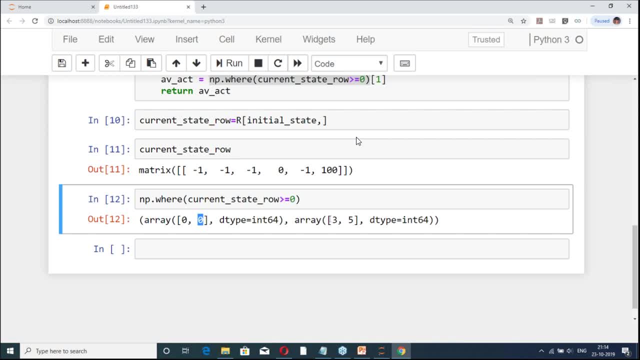 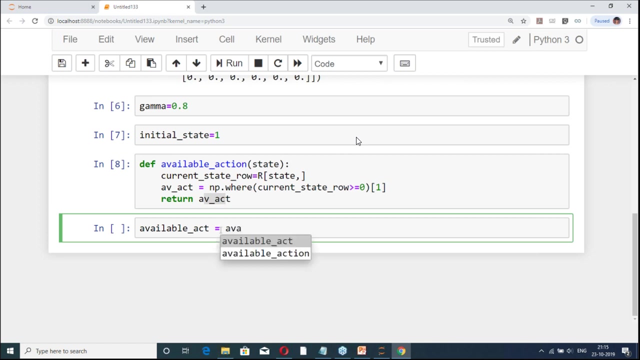 So this is what is being written by us AV act, So let me just delete these code So this will be returned by the AV act, right? So call this function and it. So let's say available act is equal to available action. 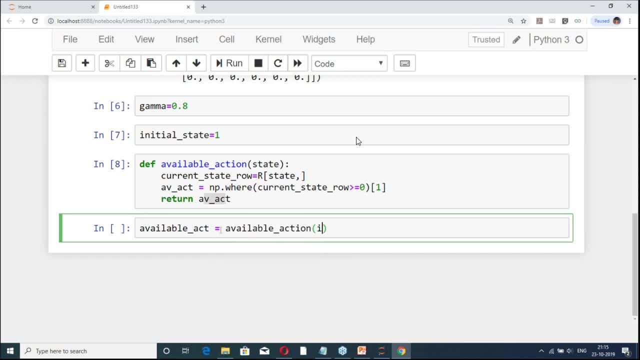 And here we pass our in. So if I show you this available act, then you can see, as expected. 3 and 5 are the possible actions which you want to take now, what we have to do. There are two possible action out of these possible action. 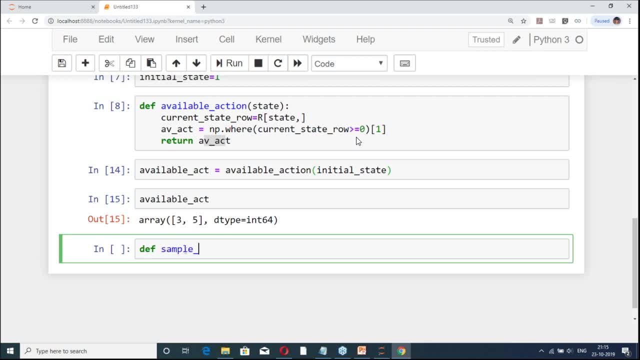 We will select them randomly. So we are going to make a function which is, let's say, sample next section, which would be our next randomly action which we are going to choose. So within this function, let's say, we are writing available actions range. 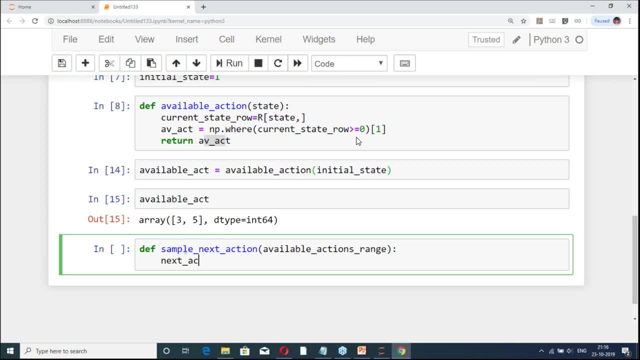 And this will do what it will choose. next section: randomly. So we write here We'll be converting it into, because it give us the array We need to convert it into integer. So we take empty dot, random dot choice. So randomly we will select some of the value from the app label action. 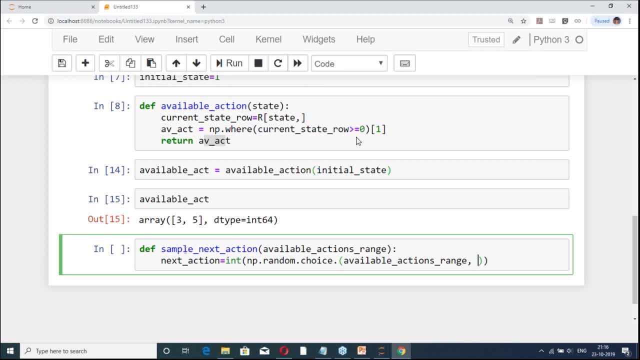 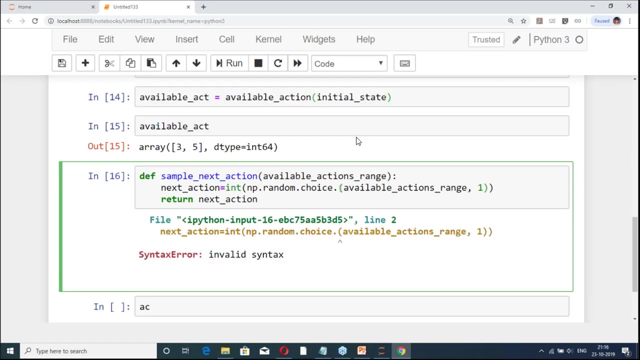 which our actions are possible And how many values we want to select. only one value, So we write it and then we return this next action. So this, so one second. here I have written dot, So if I call this function right, 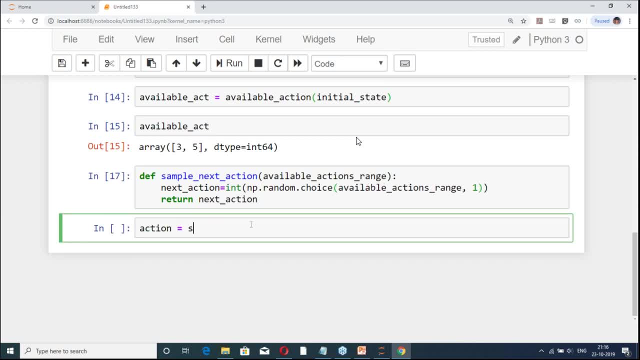 so let's say I am writing here This action by calling this sample next section, it will act. I should use this action So you can see that. only it has selected this file And if I re-execute it you can see again. 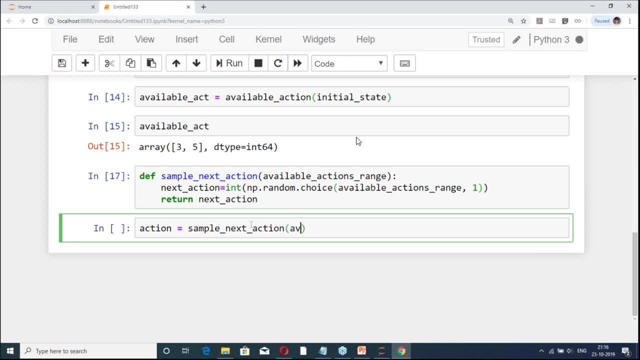 It is taking five be executed this time. It is taking five only night and you will see, it takes three as well, right? So it is being taken completely randomly. Okay, Now, okay, now, okay, Okay, values. right. So, as we show, similarly, 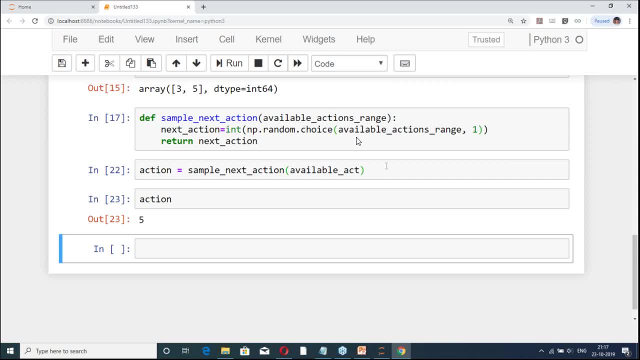 we need to have right. So how do we have this Q and E- the same formula only. So for that we are going to make the function update and here it will take the current state And after that it will take some action. come right. 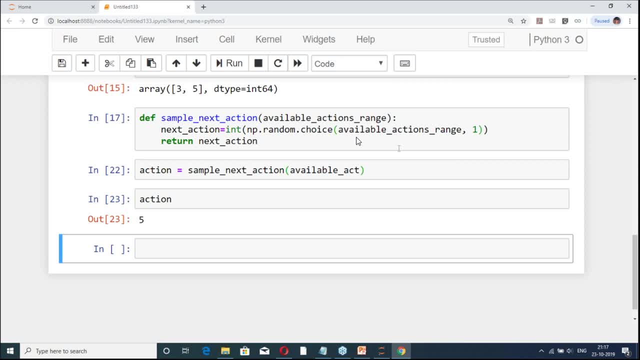 So we'll pass current state will pass it, action will pass in gamma value And then it will be, first of all, what it need to do it. as you Remember, the formula formula is this: Q state, action is equal to reward and this maximum value. 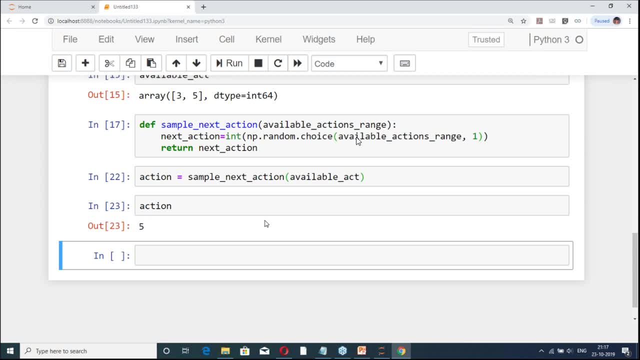 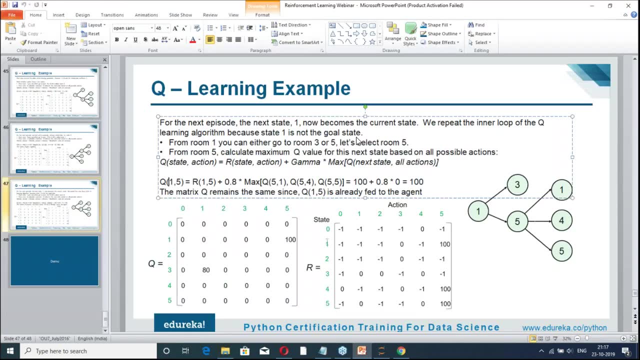 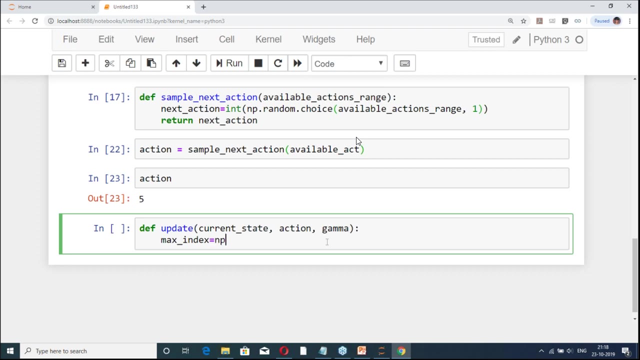 So let's calculate this maximum value first of all. So let's find its index. Max index is equal to, and P dot there. All right, So what would be given to us? Right, Let me show you this thing. So what would be given to us? Q action is given. 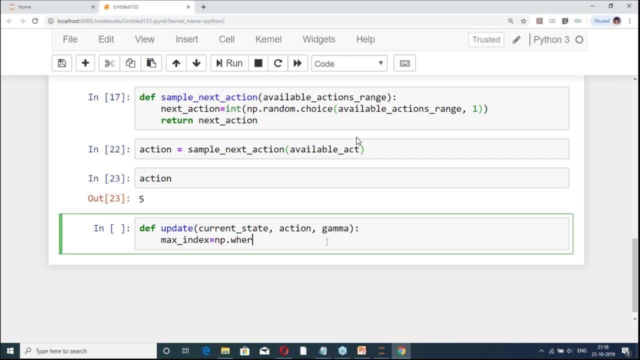 Right, So particular row. let's say this is some particular row, right? So if I want to calculate Max, if I write here Max out of it, right, So what it? sorry, we do the and P dot max, right, So we get the maximum value. 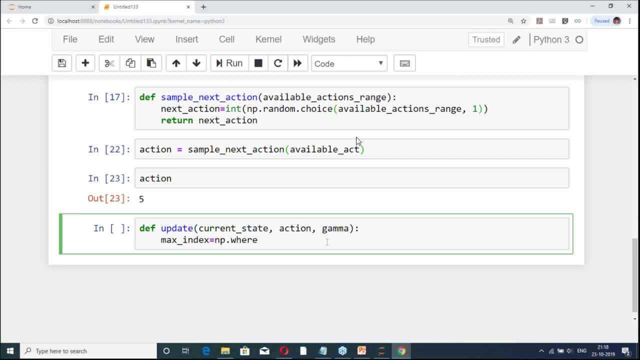 So one way is that we can use the entry dot where, where, and then I write: the maximum is straight, or I can directly choose this amp dot Max as well. I can write this thing So, rather than I will write directly here: Max value is equal to our and P dot Max. 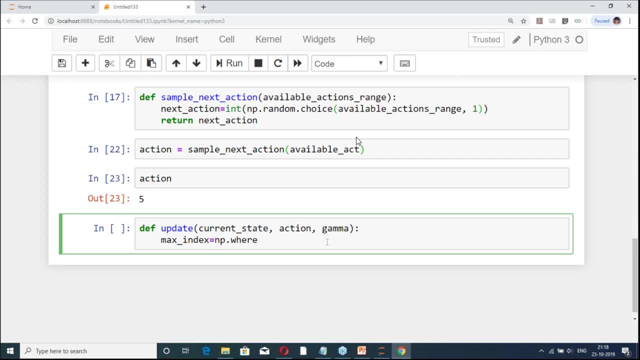 Right, And it needs to take the maximum value from this particular row. right, Take this maximum value And after taking this maximum value, what we need to do is to apply our formula of getting QL to write Q- current state, That's whatever current state was given to you. 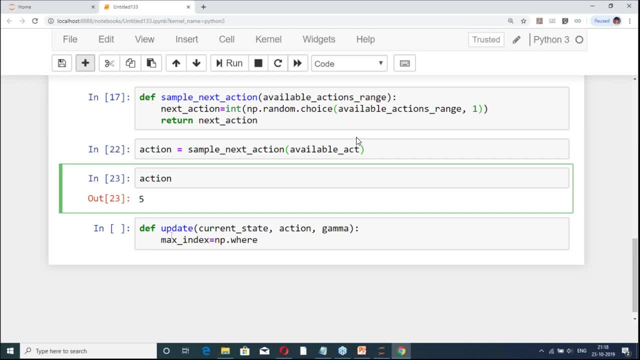 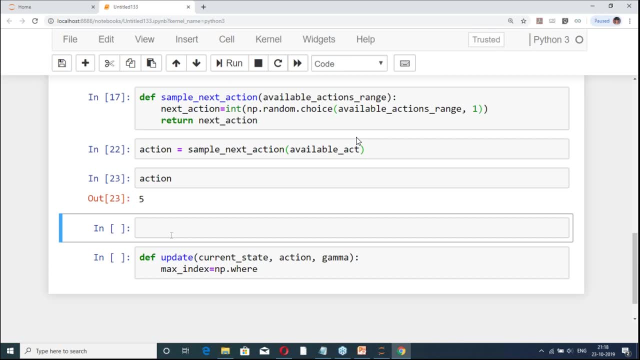 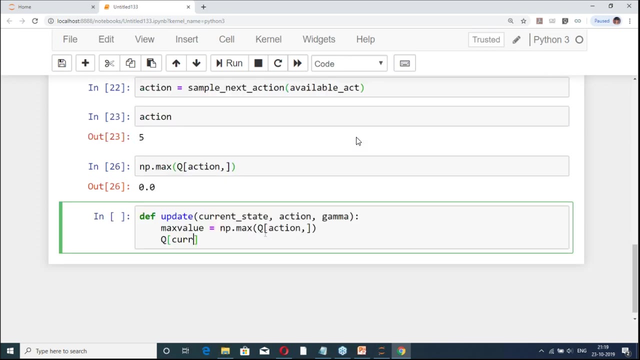 Then we write action here, whose formula is reward. from the reward We take sorry, current state, right, And with this what action it has to them. plus we multiply the gamma with the max value, Right. So this way we will write the Q value. 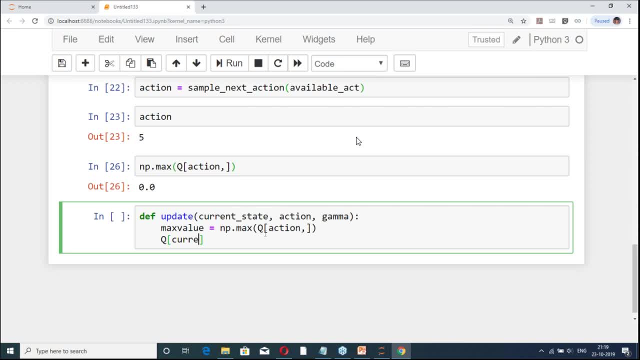 right. So let's see how it is. So currently our Q value is zero, zero, zero, right. And we have chosen some action as well, right. So, like five, action we were to them. and at the state we? at what state? viewer, initially, initial state we took. 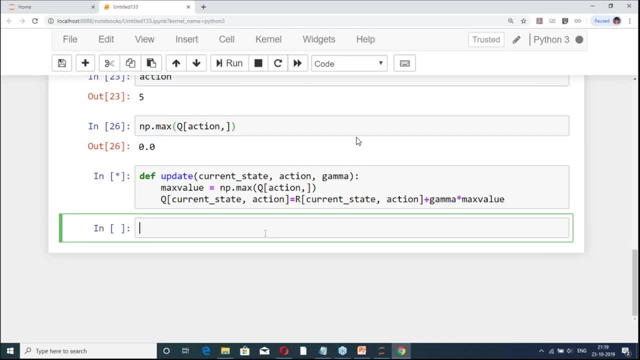 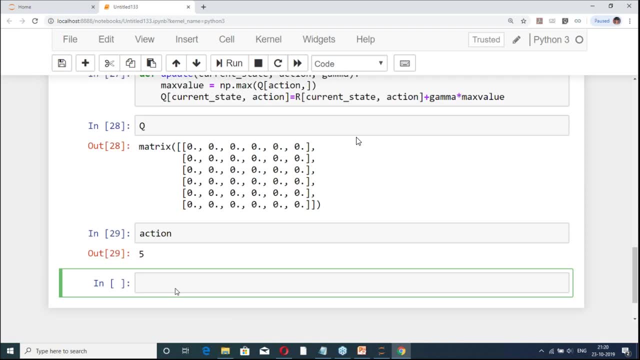 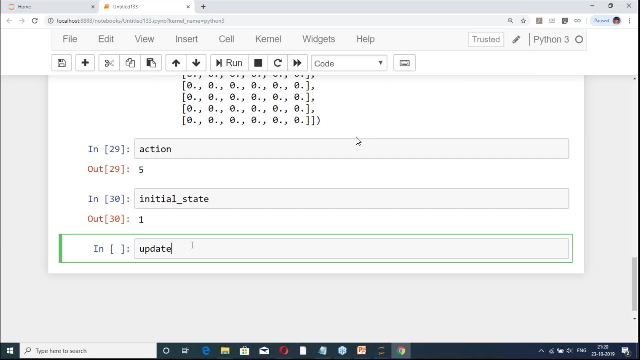 as a one right. So now, what we are going to do, we are going to call this update function And here we will send our initial state, will send our action and, other than that, we will send a gamma value. So we write it. and now, after calling this function, 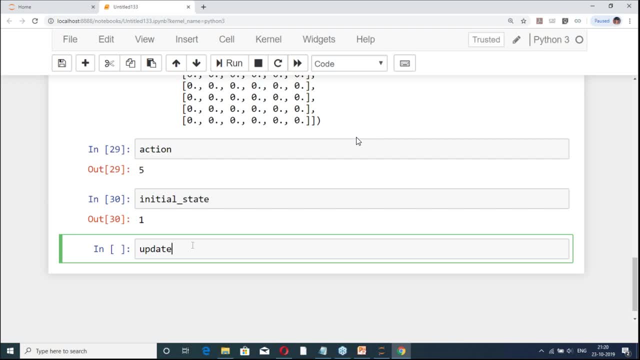 we can see as a spin 50. We saw that the value at this place has been updated 200 right now, this taking particular action being in particular state. So what we need to do, taking different, different action in a different, different time. So randomly to this action. 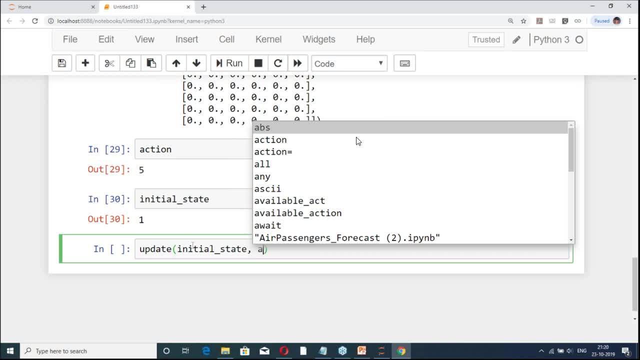 right? So here we can see. And then it is knowing how good some state values. So what we are going to make our system is, we are going to make it play this game 10,000 times, right? So it will try different friend, 10,000 time. 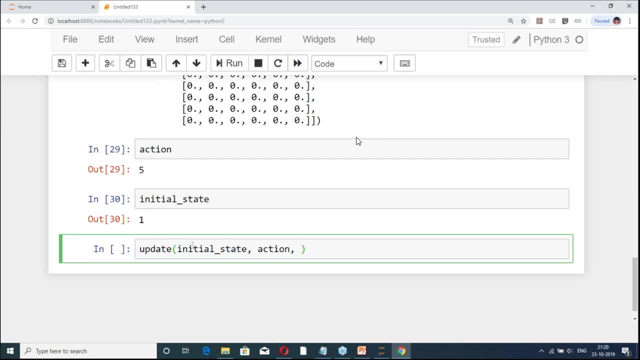 It will play. and every time you give different state- thousand, 10,000, and here we will choose some current state randomly, We will put it Into any state, right. So we write: and we got random dot rain int that it goes from random it in between of 0 to 6 rights. 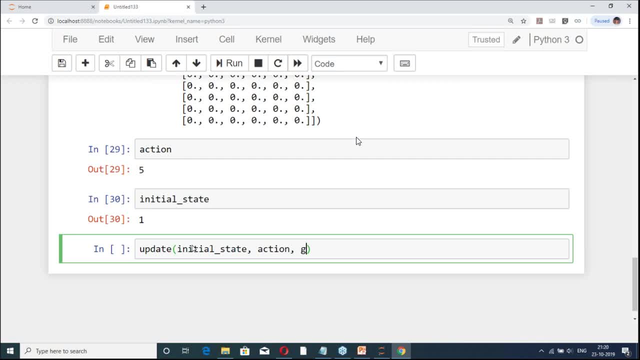 So randomly, say from 0 to 5. So we write out this one greater than that And after that it will find out the available act, right? So randomly we are making our this system, our This agent to be in any state, right? 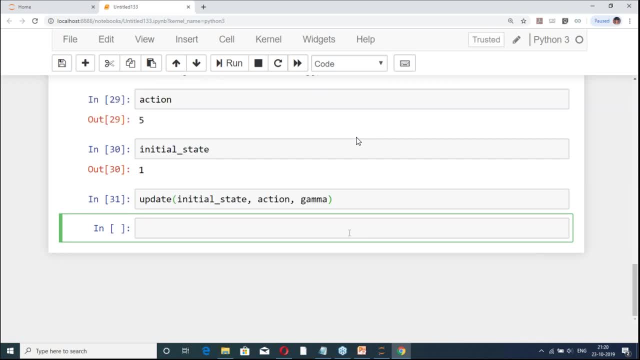 And after the it will take the action. So here we write: available act is is equal to available action. So we can create the avalanche action as we take the function, the current state, and then we select. so here available act, So we are finding out how many actually can take there might. 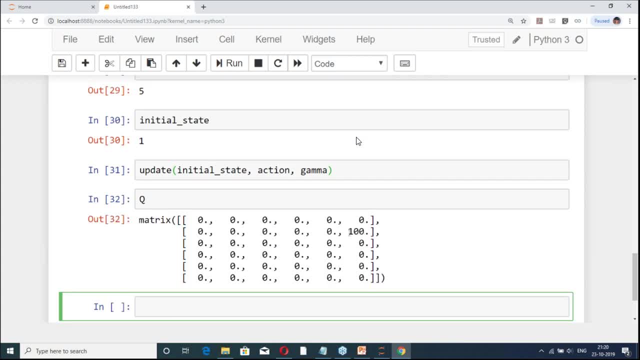 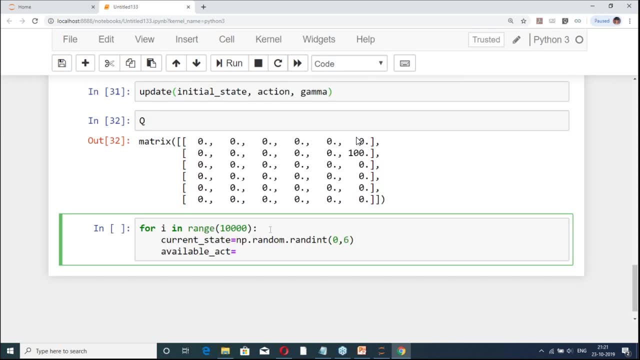 be more than one, then we are choosing one as a final action By calling the sample next, next action function and here passing it, all the available action actually, And after that, once it gets it and we need to update the value of Q right. 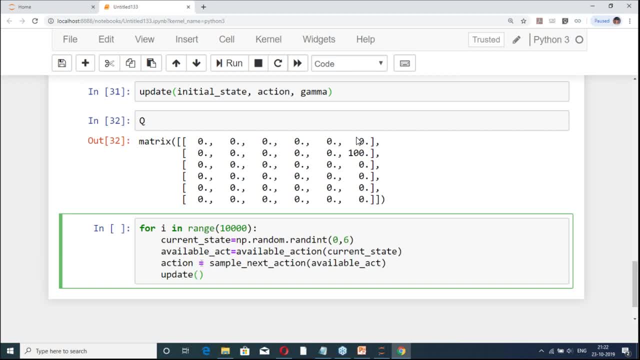 So we send it current state, We send action, We send gamma It here Now we can execute it Right. So if we execute it, so it is being executed 10,000 times- Now we check Q values and we can say it has been updated, this value. 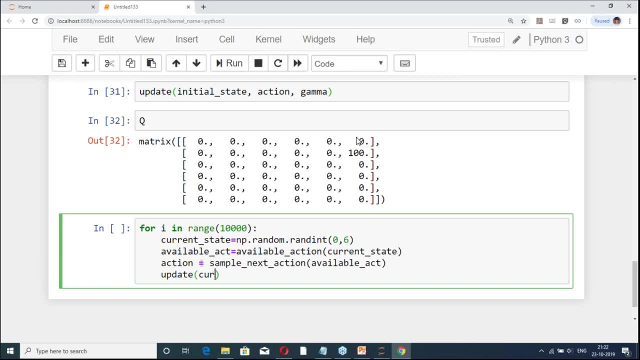 right. So you can see, this is the Q value which has been created Like this is 320, 400, 400, 256.. So these are the cubes. So it is showing how much. what is showing that in this particular is, in this particular, this is state 0.. 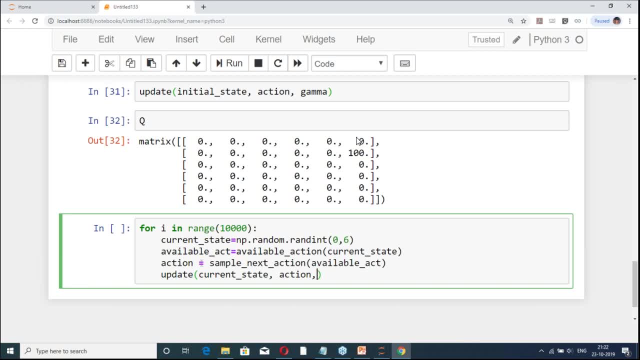 This is 1, this state 2.. 3, 4, 5, right. So, in this particular state, if we take this particular action, which is 0, so 0 for it is value 0. if we take this particular action, worth is 0. if we take this particular action, worth is 0. 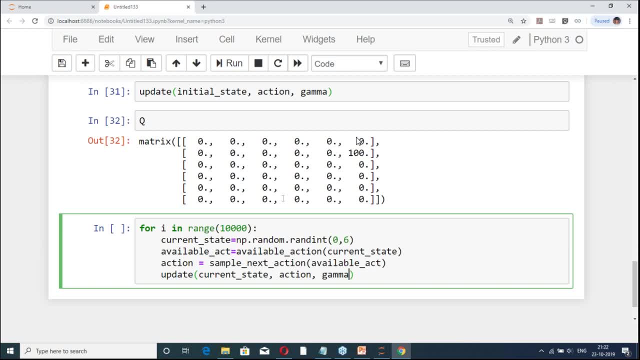 because also here, but we take this particular word- is 400. So it's become a policy right. So, being in a state 0, what is the frequency that I will take this action where I'm getting the taxi on board? So when it is in state 1,? 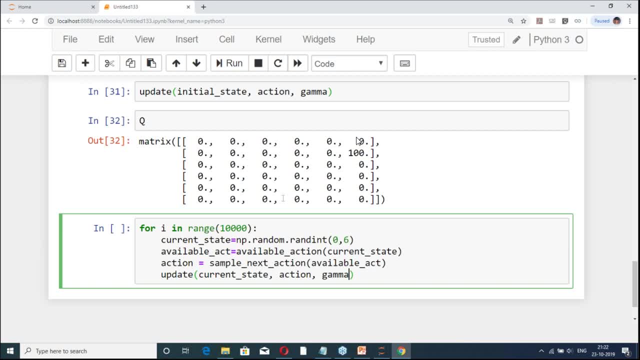 then it will see that if we take all this action, we get some positive values. But so which one is the maximum is the 500.. So the policy will become so that it can get the maximum value, which is 500 in this case. similarly here, similarly here, similarly here. 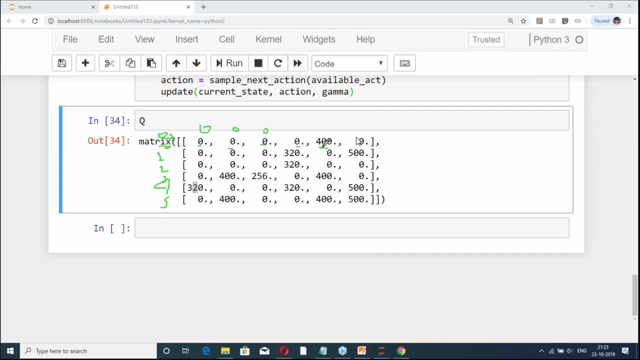 So let's find out some path. Let's say after learning the path, So it has learned the path. right, It is equivalent: that Mouse has tried different, different action and it has learned The complete path of the business. Let's say this was a miss only. and now, after learning this complete path. 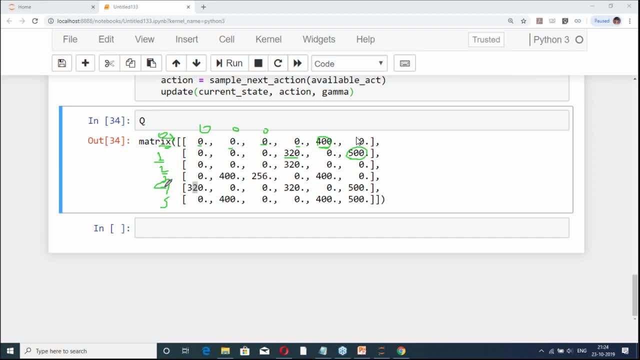 let's see how it is going to reach to some particular. what action will take in a particular state? right, Let's say we, as we said initially, let's say our. you were kidnapped and you were stored, Let's say, into the room number two. 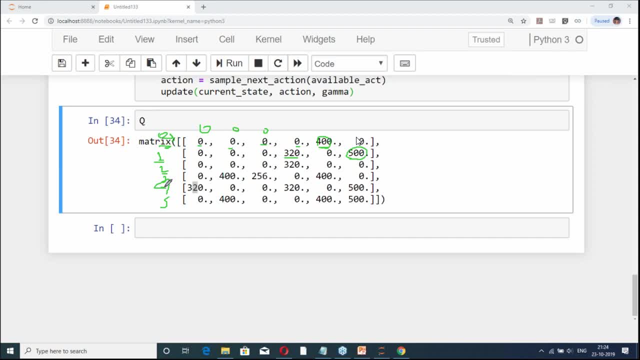 right, Let's say you were stored into the room number two, room number. This is this one, right? So how you will be going from two to five, right? So you need to make sure that you do not get lost in between of them. 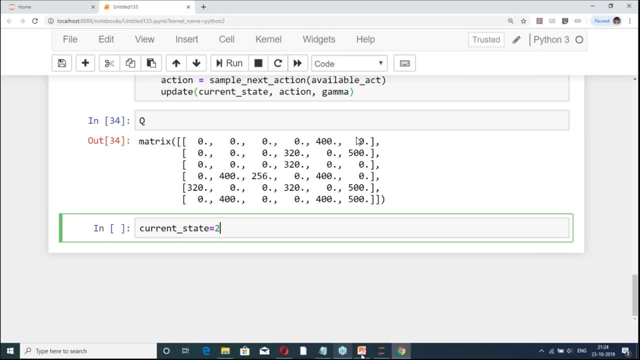 into some kind of circle and all. so that is why, once you learn this stuff, you can use these policies right. So let's say the path which you guys are taking you will be writing into this staff's list, right? So let's say he shall things that you are in current state. 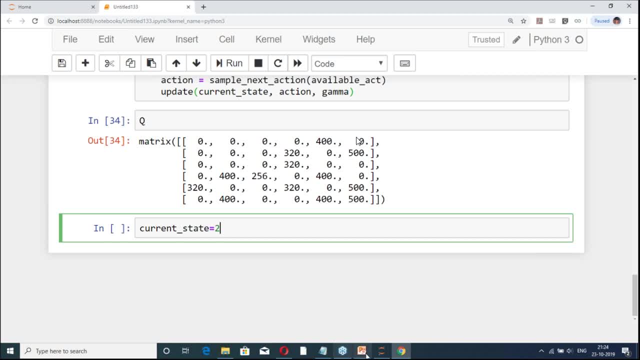 That is. we are here. So tell you value: keep moving till your current state is not become file. you reach to the final state. So we have done it, It has learned that it, but now it is going to play the game right. So it is going to reach to the outside. 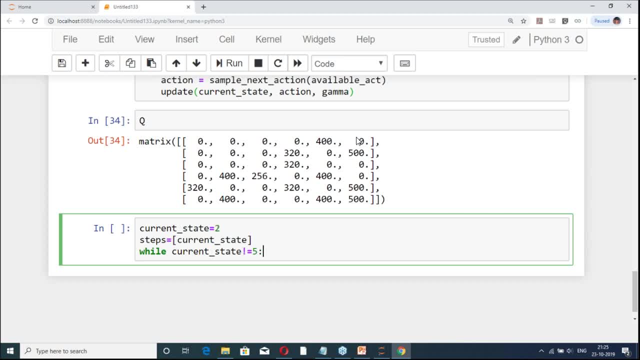 You have that team in the state number two- Now it's age to reach to outside- and state number five. So what you will do first, you will do here. You will find out. next step: index. What is the index of the next? which? the value, the action? 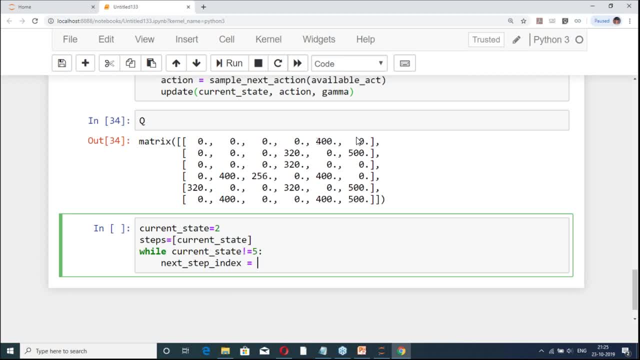 which you will take. right, That is the maximum, like here. What is the next step you should take is taking reaching to this particular action, right? So that is what we are writing here next up index. So how you will do it: You will calculate without where which is going to be maximum value. 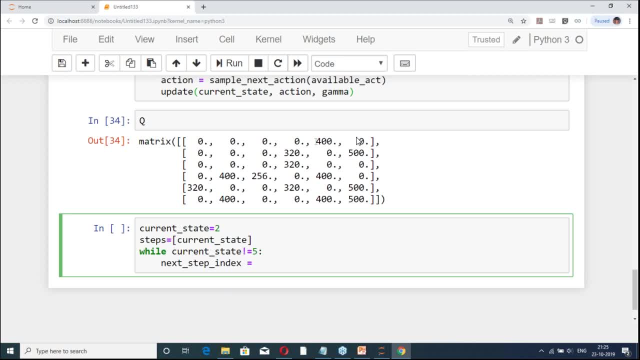 right. So you write here Q, the date within this particular row Right, And here this particular rule is equivalent to your max. So here is going to be, and we thought, X value. So what is the index of the maximum value? That is what we are finding here. 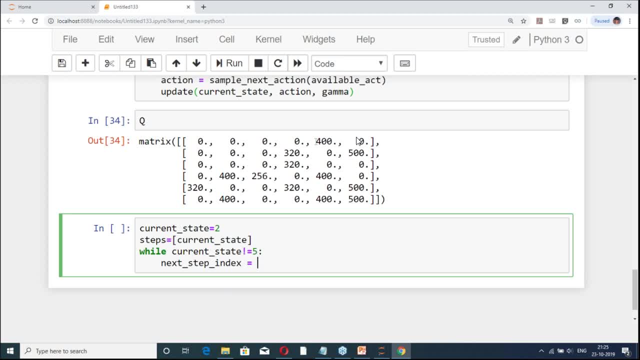 right And again we will take here the column number, So we write here one. So after doing this thing again, there might be few places where, like this place, If you see, this is 320.. This is also frequently. So what does it mean? 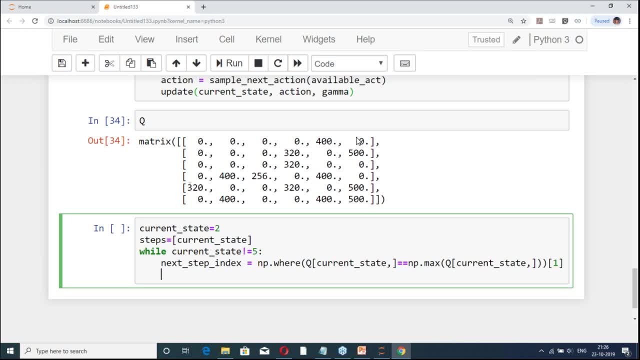 So whether it can go through this path and choose this action right. So whenever it gets more than one, it has to choose randomly one of them. So it will not in this. these two are less but it will choose this 500, right. 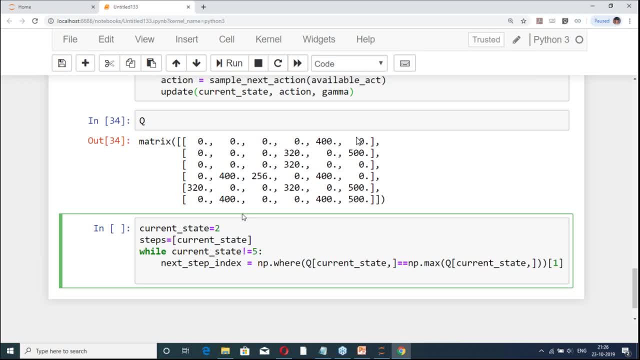 But in this case, like we have 400, 400, it has to choose only one of them. So here it will be in within the next step. index to value: in this case Only the one value. So we need to check if max in tax is restoring more than one value. 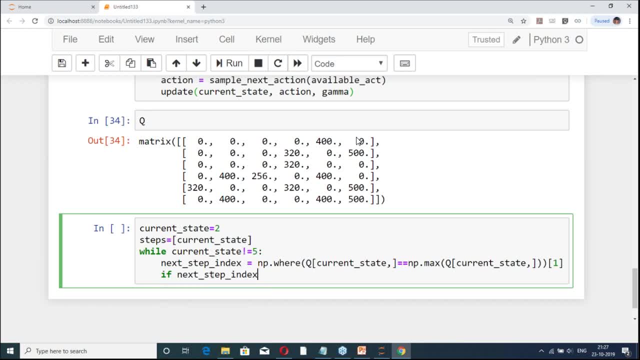 So we look into its shape, that is, how many values it is having. if it is greater than one, more than one values, It is picked up and randomly we will choose one of them. So we say in and to empty it or random Dot choice randomly. 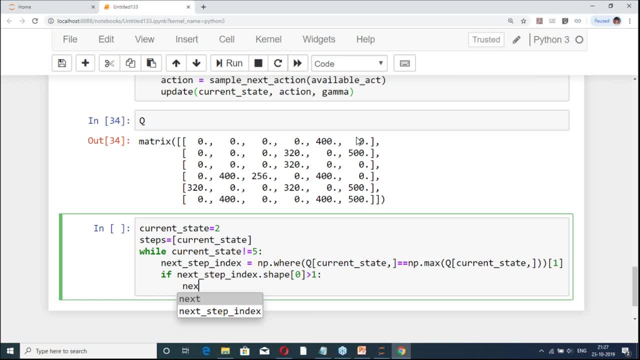 We choose, We value, next stop, index and how many values you want to do this. only one value, right. So we randomly choose this thing and after that we write next up in the hex, because it would be arrayed, even though it would be one thing. 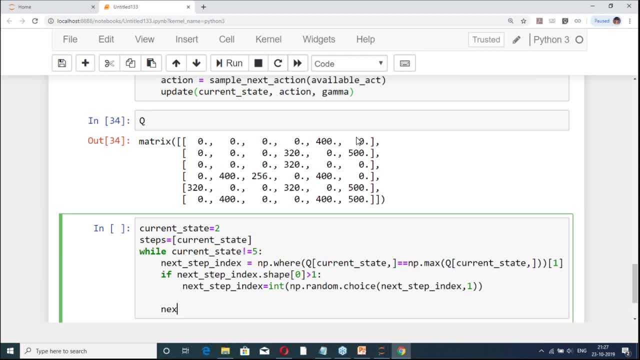 but we want to convert it into integer, So let's take it integer and after. so, basically, this is the action It has taken. so we'll do staff start append So we can see what action It has taken. that is our next step: index. 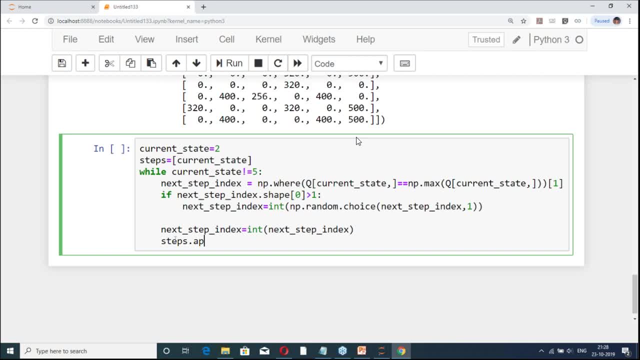 and then here state: basically, now, after taking this action, It's current state reaches here, right? So how does what is stated to be clear- Yeah, that's right, This thing is our, that is our index- become our current state now, right? 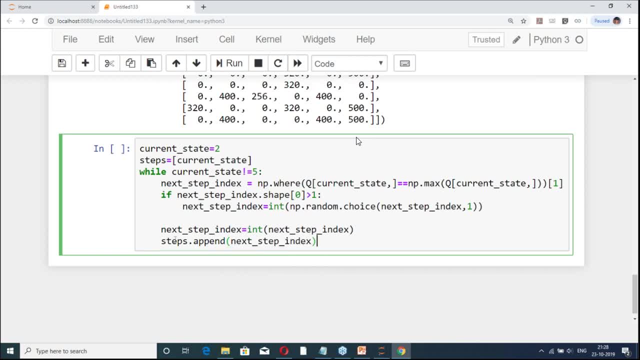 And we keep executing this thing. Executed now. Now let's see what step it has taken exactly to reach from room number two to outside, That is, room number five that we have into this class. So here, from the two, it reaches to number three. 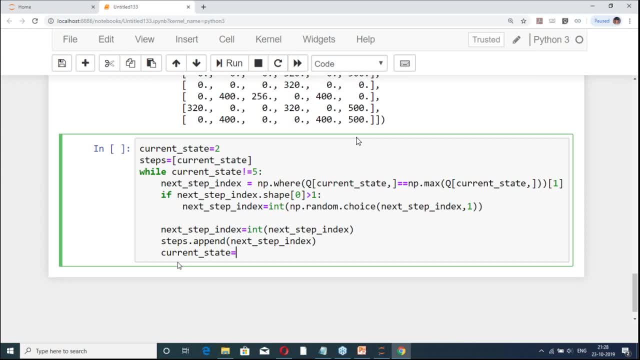 then number three reaches to room number four, then from room number four it reaches to room number five. So if you see here: Yes, sorry this one, So we also let's print the Q state Q matrix as well, right? So you see here Q matrix. 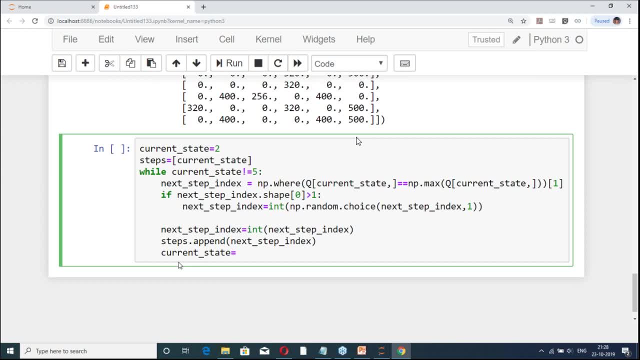 So how we started. we say initially it is in room number two, So this is zero to. so what action it has taken from room number two? It has a piece to number three that is the only available room, So it goes to this room number. 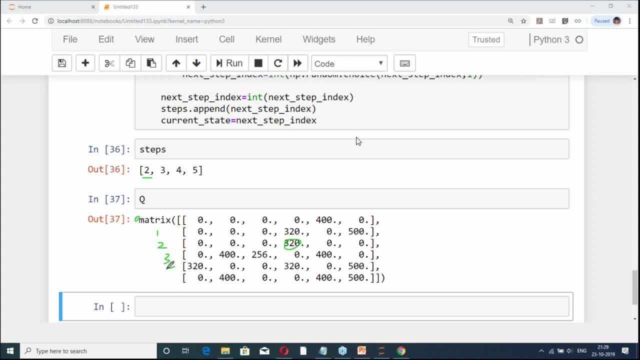 Let me write it here: three, four, five as well. So once it reaches to room number three, what is the next action it has taken is the four. So it has the two options: have number one or room number four, but it has taken the room before randomly. 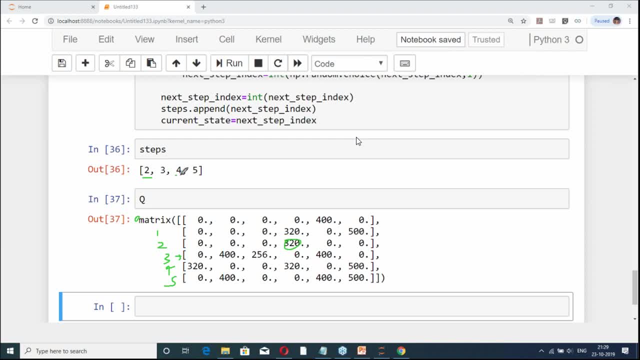 So it goes to room before. now It looks. the maximum value is this: that is reaching to room number five. And finally, it has reached to the room number five, right, Even? if you want to see this thing from the figure of this graph, then you can see from this figure as well. 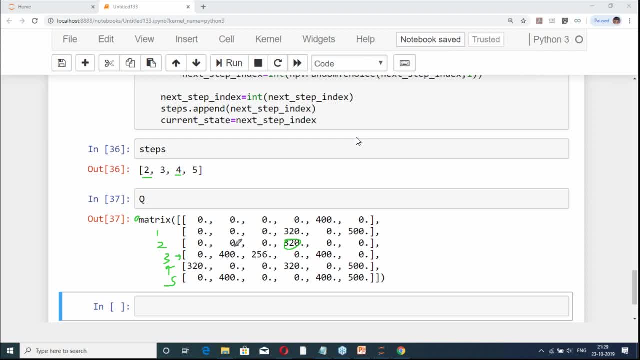 So how it reaches? is that in? it was in number two, Now it goes to room number three, Then it goes to room number four and then it goes to room number five. So you can see it didn't take the first towards room number zero. 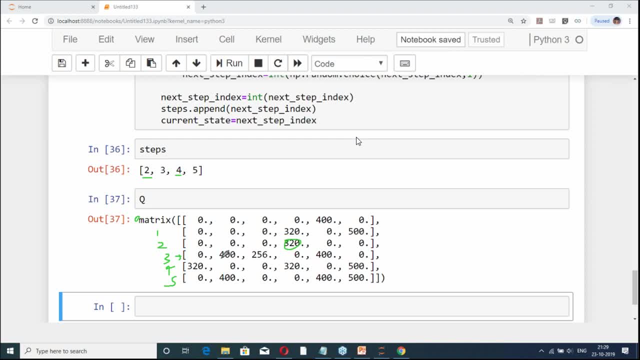 then come back here. right, All this trial has done, while learning right, using the Q learning algorithm. It already done. What is the best route? it find out already What is the best right. So same thing you do with the game, same thing. 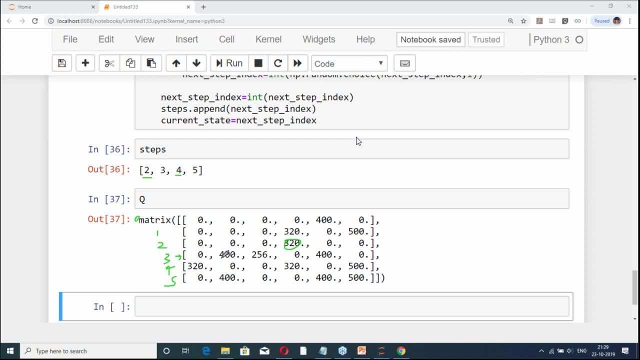 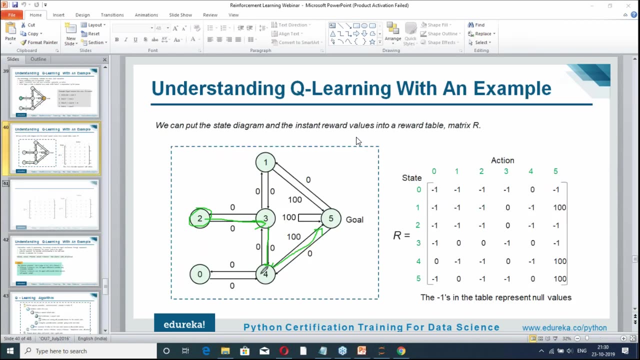 You do the driving we try to find out. it plays when earlier it was in room number three, So reaches to room number one as well as for when it was in room number one. It tries going back to three as well as to five, So it found already those things and accordingly it is the value right. 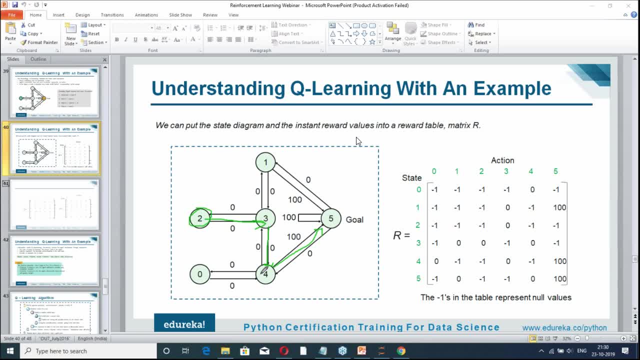 That is how we reach to this final value, Right. all these things Okay. so that is how the things are happening, right? So I hope this is clear to all of you guys. Let me know if any guys have any doubt Before we finish this session. 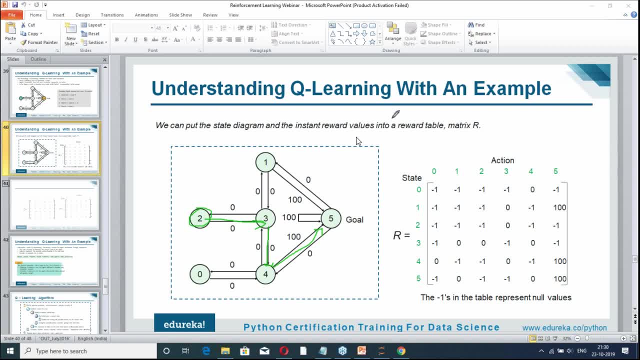 Okay, great, All of you guys Great. so We need to need session and let me do it. You guys can enroll this post. I told you right: If you're in school, you get a certificate and you will be knowing all these topics in very much. 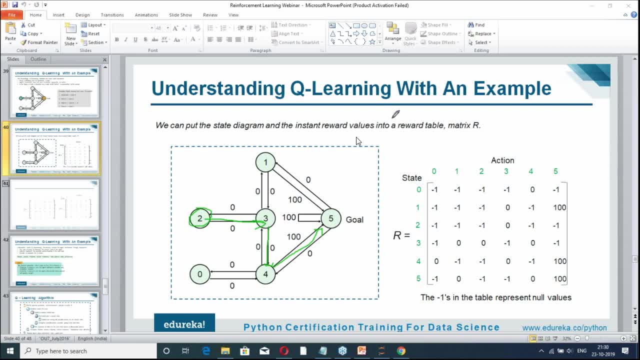 That not only knowing, will be doing a lot of projects. He said to reach and get a few algorithms which you guys have not seen, even till now, And even you have seen, not into much, very much detail and things you will be going through and you for this course, and today there is 25% of, if you do webinar and eat five as 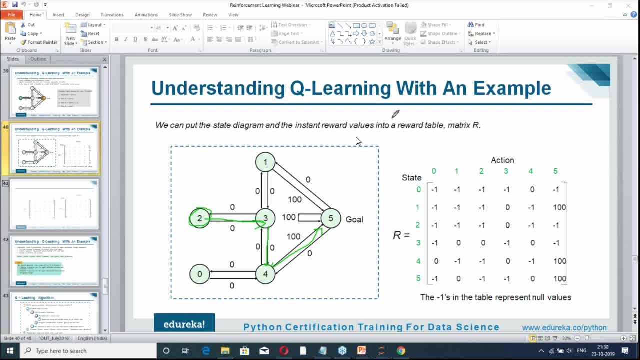 So in the cabs it is webinar And if the whole fair and just shift you and roll for this. Thank you very much guys for listening with so much special and asking good questions. I know there might be still some ship, some curiosity might be there, but we cannot go into much detail of these things, but I hope so. 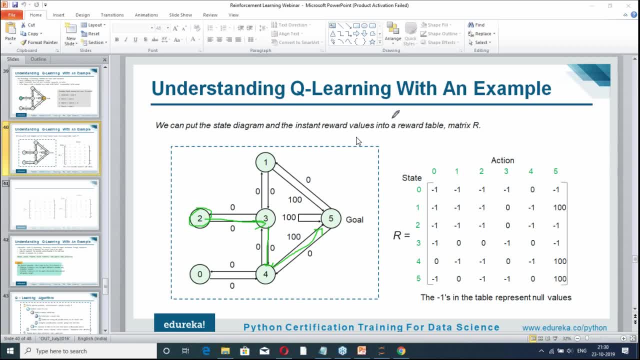 It gives you a clear idea How wonderful this reinforcement learning algorithm is: any problem statement converted into this moment learning column and that you apply it. Thank you very much, guys. Bye, Bye, Okay, Happy Diwali. See You after the body.